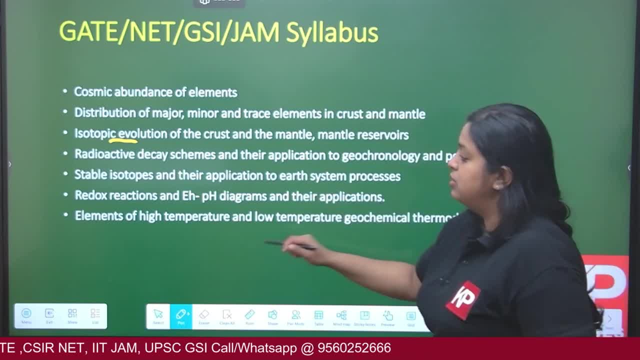 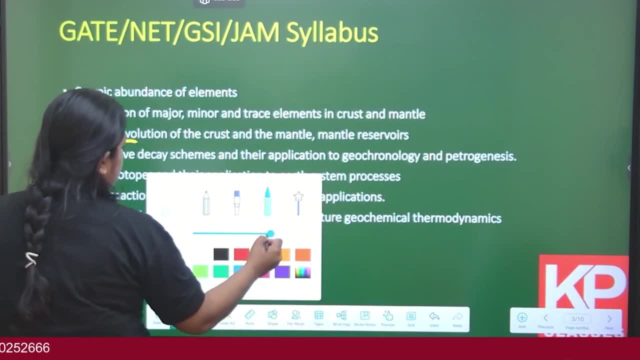 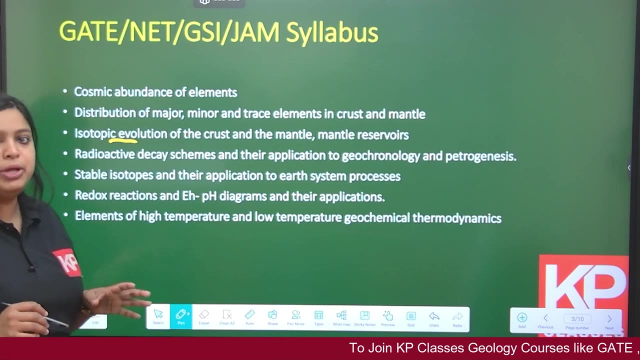 redox reactions and EHPH diagrams and their applications. elements of high temperature and low temperature, geochemistry, thermodynamics. So when, when you come to these portions- actually these are very important In GATE- mainly minimum three questions come from this section Sometimes. 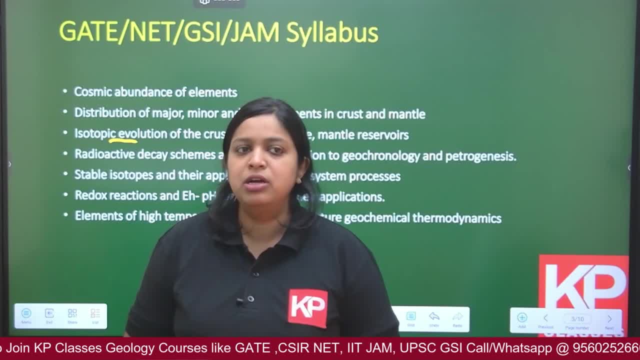 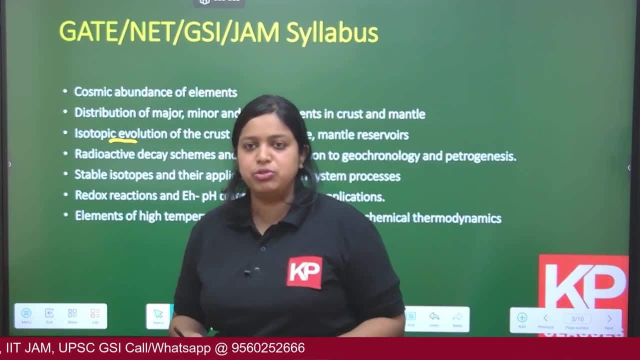 two to three questions will be there minimum in GATE paper. In NET also there will be three to four questions will be there from geochemistry portion. In GSI maximum two questions can be asked from the geochemistry portion. Numerical questions do come from this section. 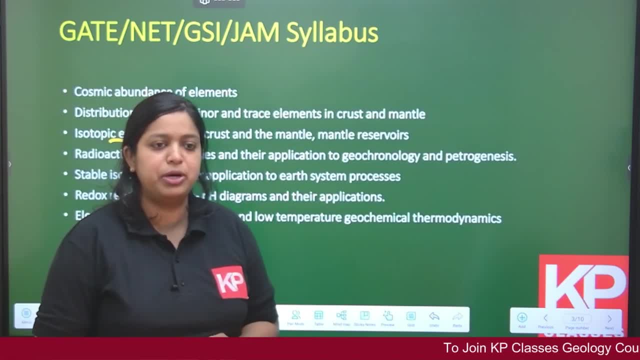 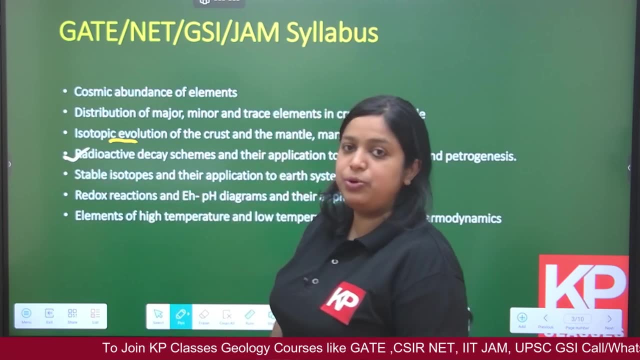 This is a very important part. Geochemistry is a very important part. when it comes to the numerical questions, They ask numerical questions related to, you know, radioactive decay schemes, the equations related to that, half-life, mean life or the number of parent atom. 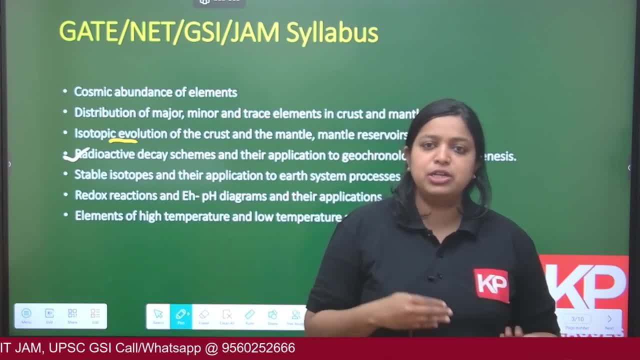 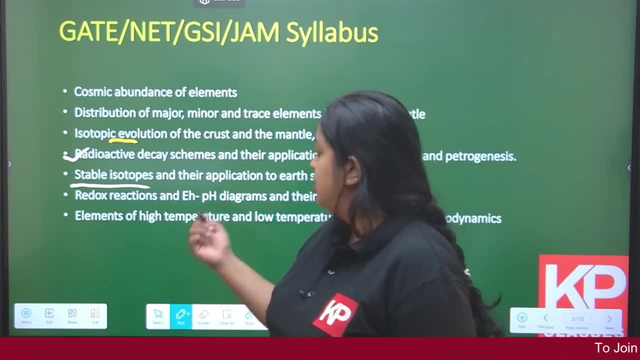 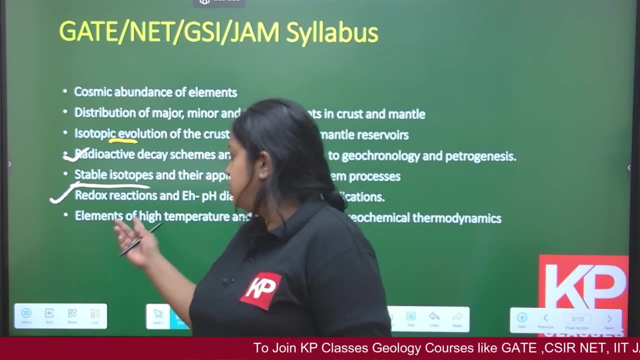 number of daughter atom. those equations are very important When it related to stable isotope also, questions can be asked Del oxygen value questions can be asked. EHPH equation is very important. They have asked multiple times in GATE, also In NET also these questions, elements of high temperature and low temperature. 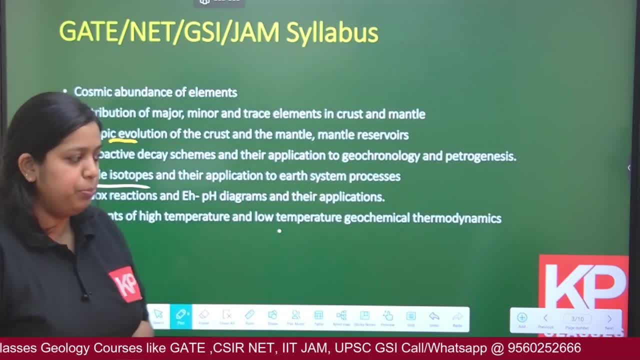 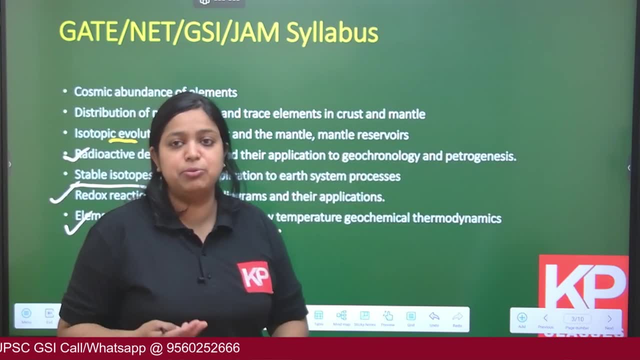 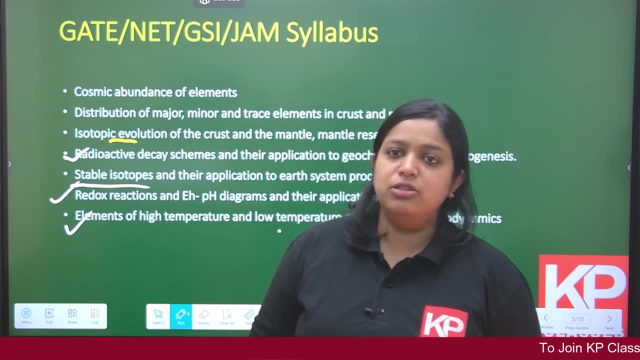 geochemical thermodynamics part is also very important for numerical questions And in GSI mainly they ask about the reserve, mantle reservoirs, The different types of mantle reservoirs and the trace elements and their applications. Those are the things that evolution of earth, geochemical evolution of earth, isotopic evolution of crust and 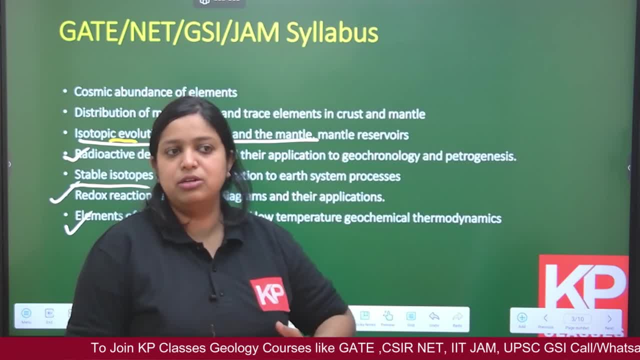 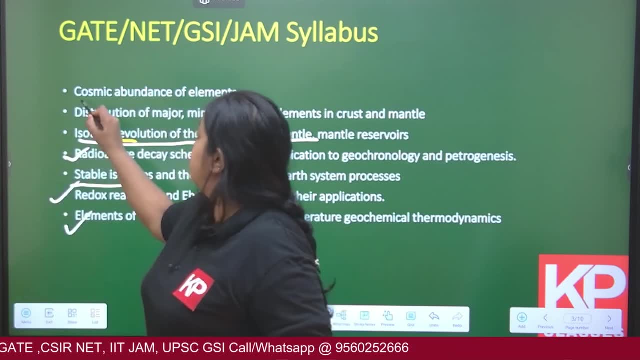 the mantle. These are very important for GSI In the with respect to GSI paper. these portions, these portions are very important. So in net, even this cosmic abundance of element is also important. you should know how the elements are, the abundance of elements present. 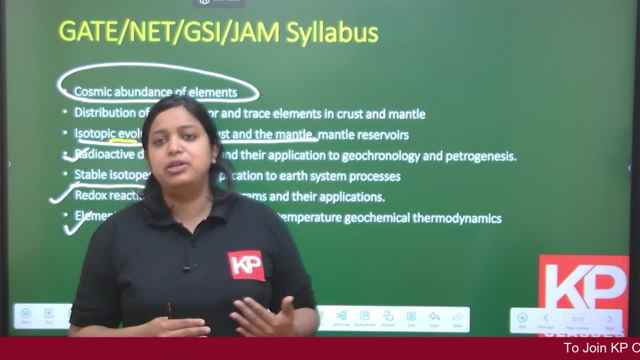 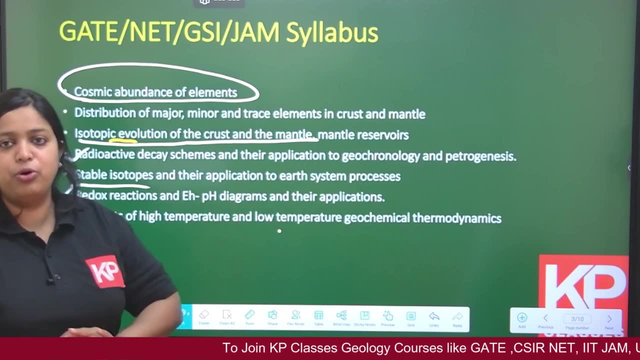 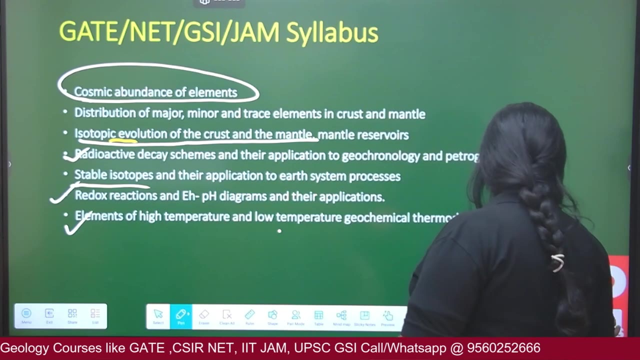 on the earth as in a universe, how the abundance is. abundance of element is elements are. So the whole topic is actually very important for all the competitive exams. So geochemistry is a very important topic. So today let us start with the ah portion, that is, of trace. 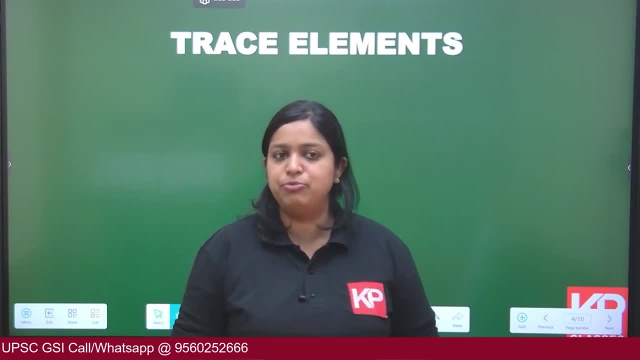 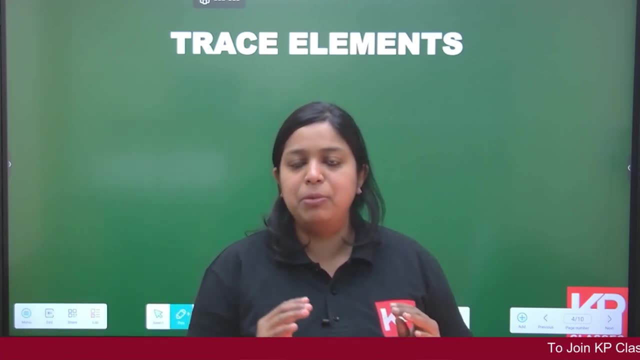 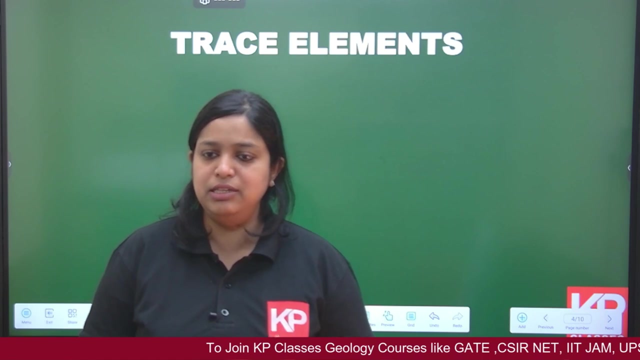 elements. So, as we know, a rock is a mixture of minerals or it consists of a lot of elements present in a rock. So, depending upon the weight percentage of elements present in the rock, we can divide the elements into major elements, minor elements and trace elements. 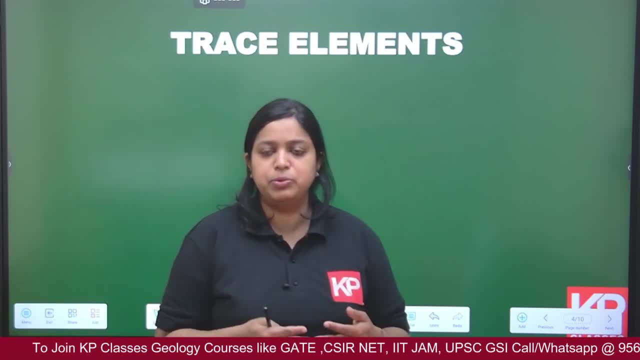 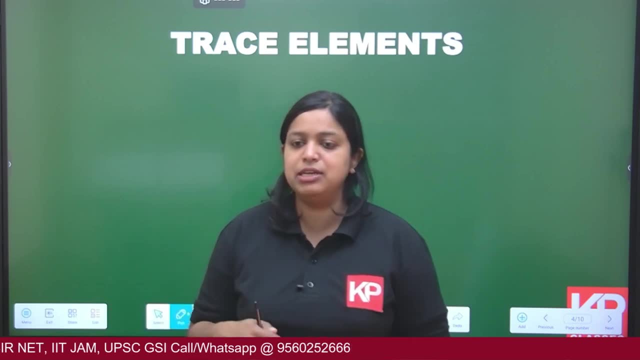 So major element means weight greater than one weight percentage of the rock is on the earth and minus one percent of the rock is on the earth. So we can divide the elements of that element. minor means 0.1 to 1 weight percentage. trace element means less than. 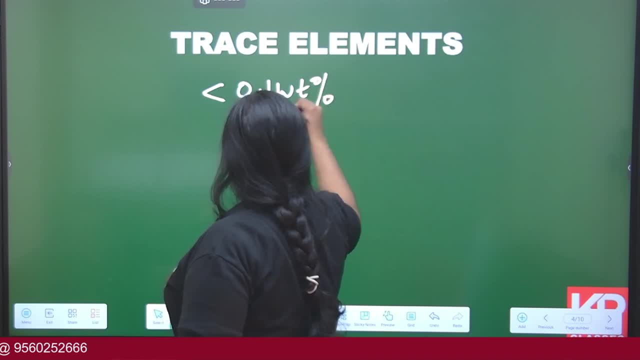 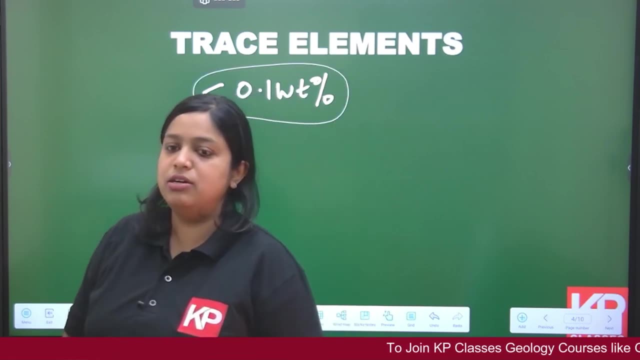 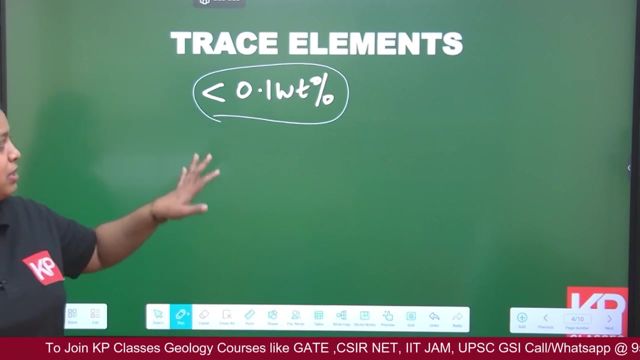 0.1 weight percentage The elements that has less than 1 weight percentage of in the rock. less than 0.1 weight percentage is of a particular set of elements. those are called as trace elements. So even though the amount present in a rock is much lesser, trace elements of. 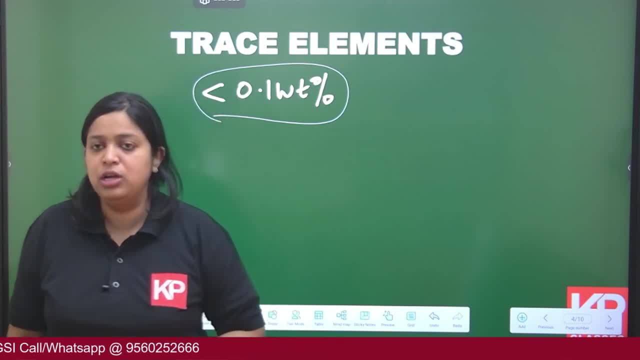 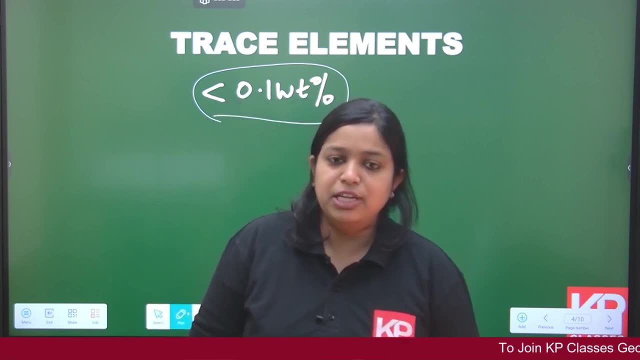 only less than 0.1 weight percentage in a rock, but still their application is much higher. We can use the trace elements present in a rock to find the magmatic evolution, to define the age of the rock, to define the like, the processes that has happened from the time of crystallization. 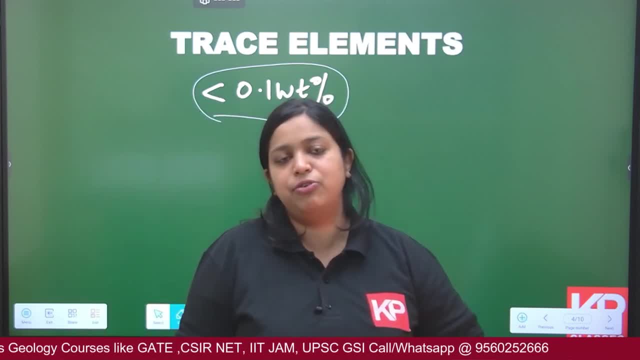 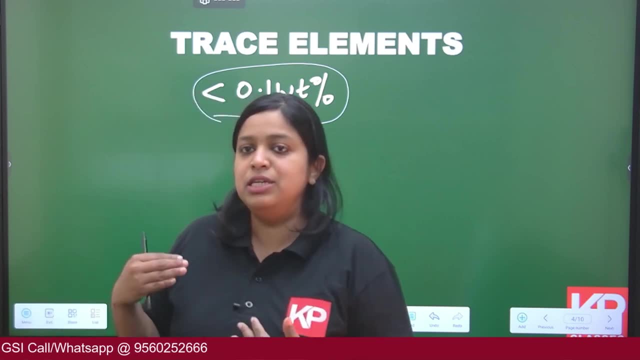 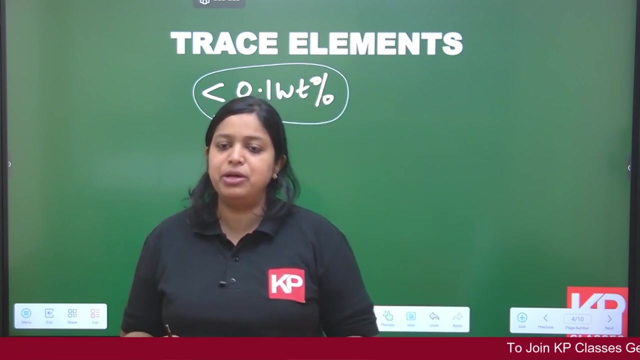 till now, etcetera. There are so many applications for the trace elements. This only 0.1 weight percentage of elements present in a rock. So this trace element concentration varies from rock to rock. Simply trace elements during crystallization of magma. 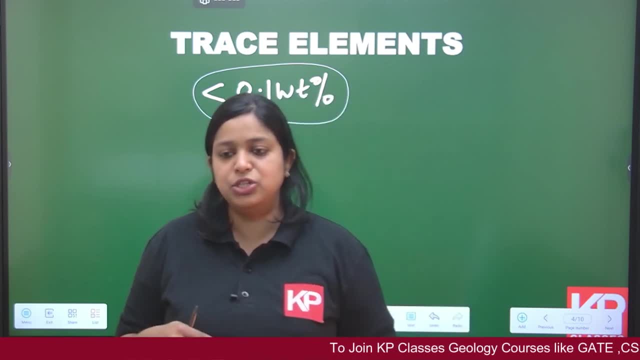 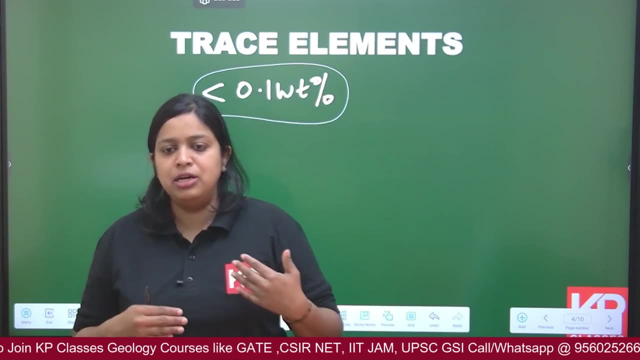 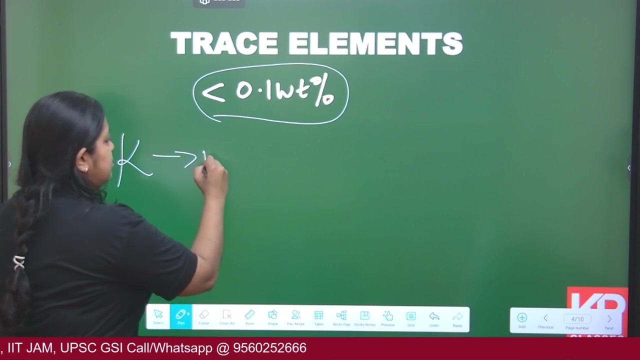 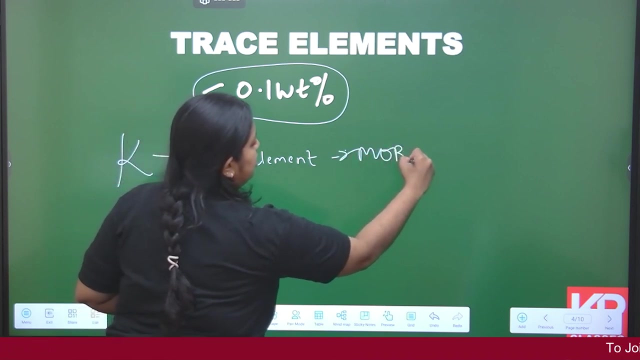 they get substituted for a major element in the structure, in the crystal structure, or they may remain in the melt, or they may remain in the magma. For example, potassium. it is a trace element in midoceanic ridge basalt. It is a trace element in midoceanic ridge basalt, Whereas we all know potassium is one of the major. 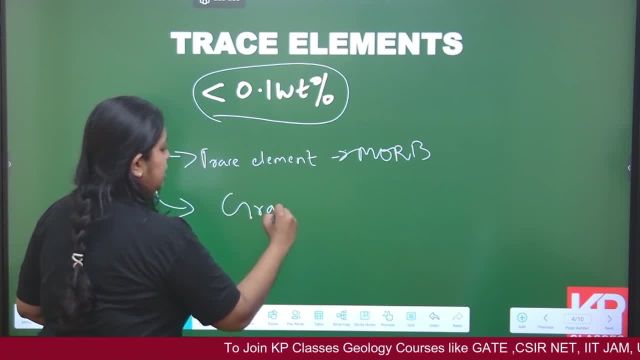 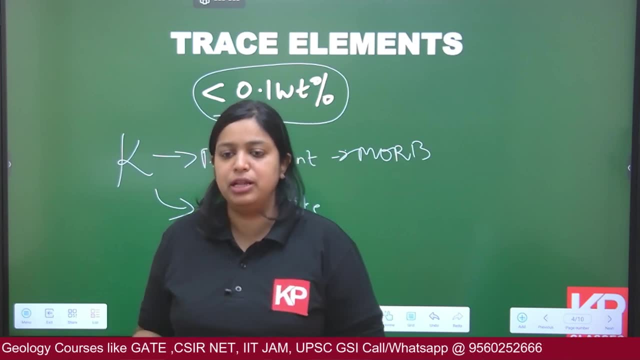 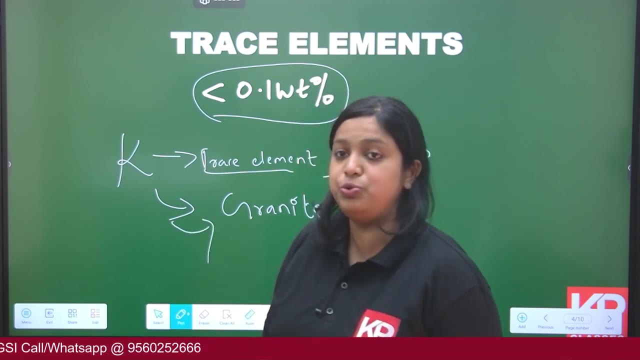 element in granite Granite. it is not at all a trace element in granite. So in different rock for a different element will behave separately. So a particular element may be a trace element in a different rock and it can be one of the major constituent of granite. 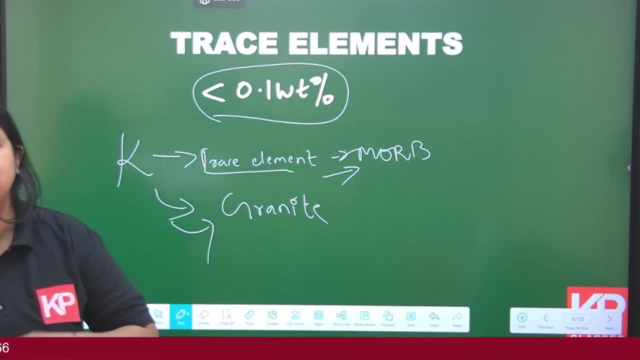 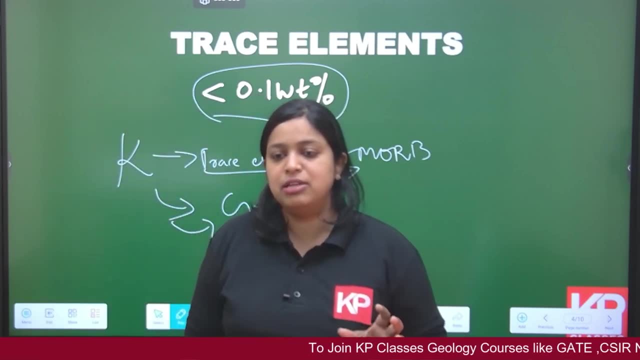 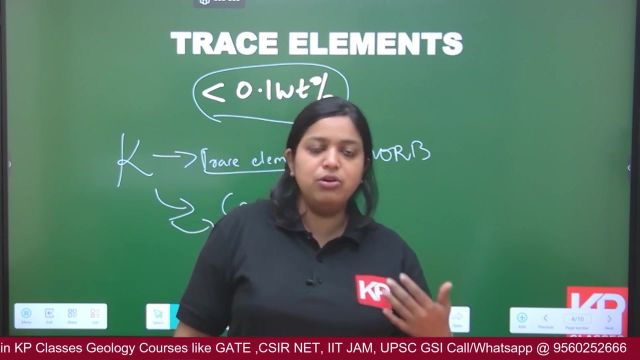 So a trace element concentration varies from rock to rock. During crystallization of a particular mineral, the trace elements will be substituting for a major element in the crystal structure, or sometimes they may not even participate in the crystallization. They will remain back in. 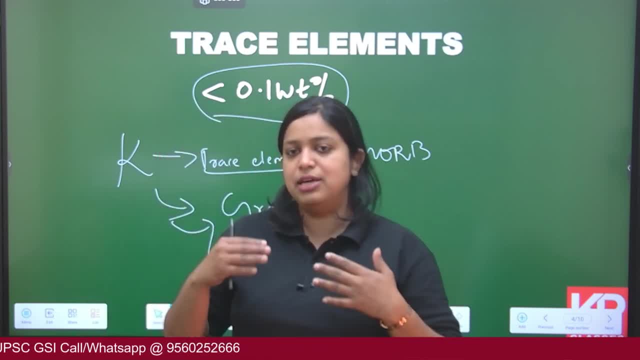 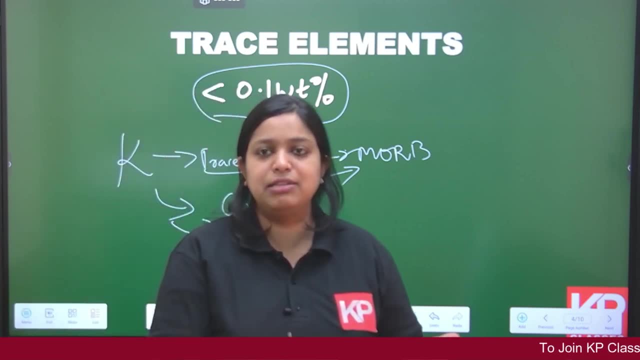 the magma depending upon their property. like this, this has the that depending upon the affinity of trace element. So this is a trace element, So a trace element concentration varies from a trace element to that particular crystallizing mineral. So we can divide the trace element. 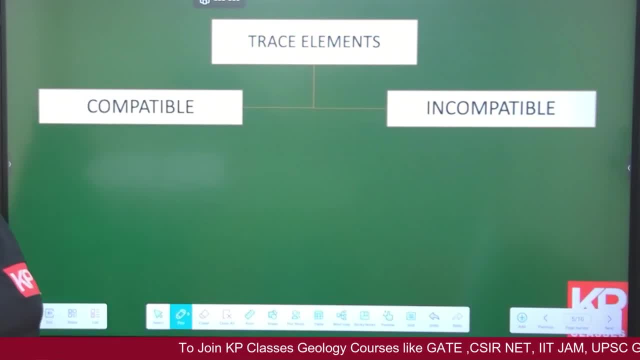 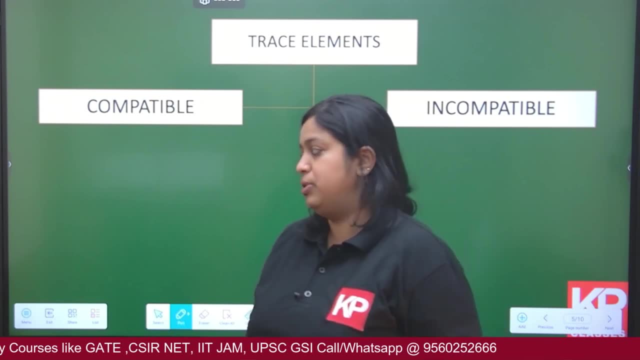 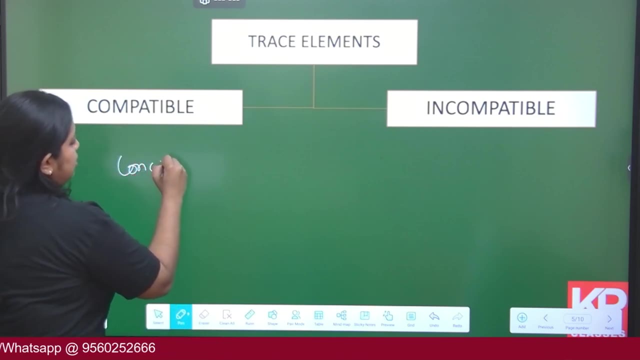 into two: compactible trace elements and incompactible elements. The entire elements can be divided into compactible elements and incompactible elements. Compactible elements means that are concentrated in solid relative to liquid. concentrated in a solid relative to liquid are called as. 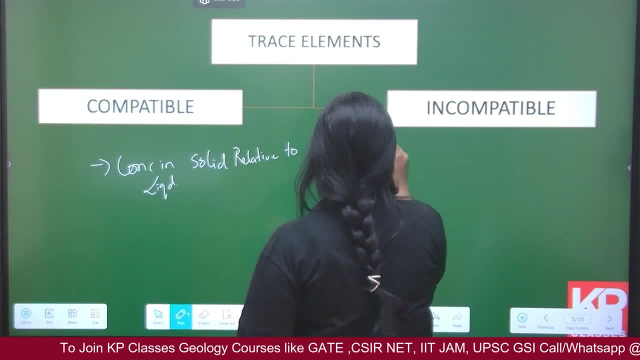 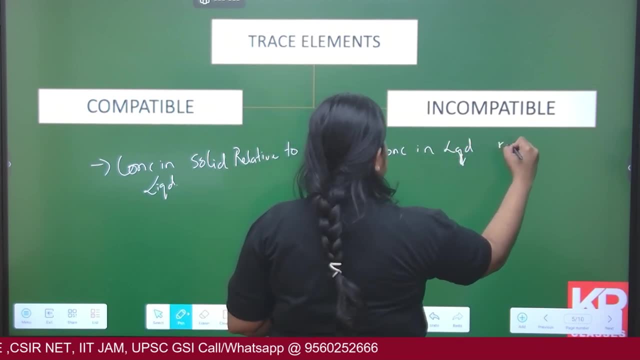 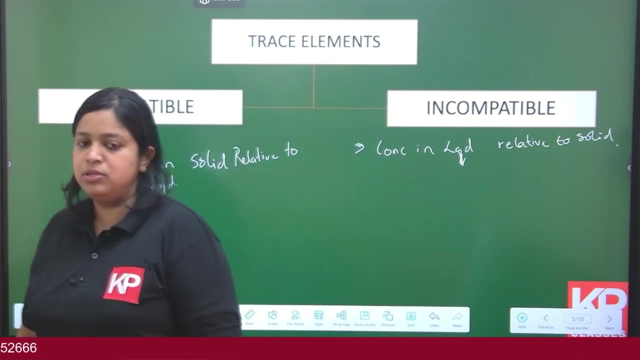 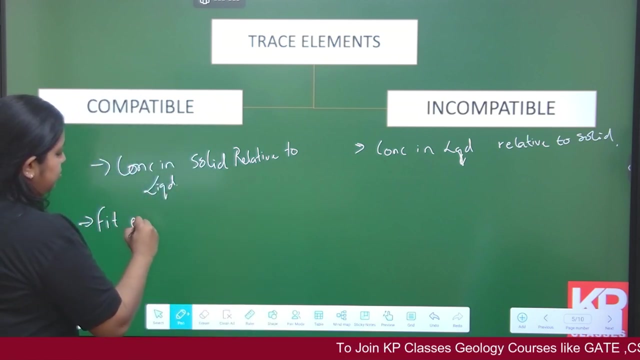 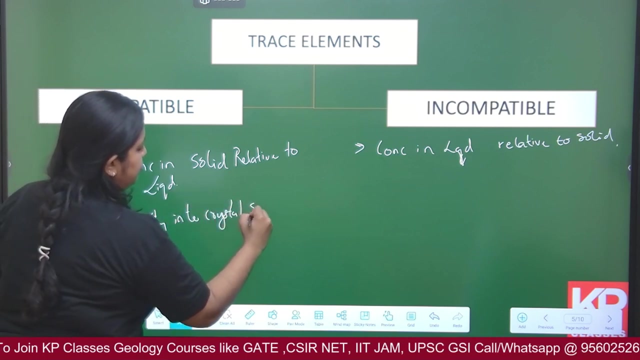 compactable elements, whereas incompatible element means the one that are concentrated in liquid relative to solid. those are called as incompatible elements. so compactable elements, they fit easily into the crystal structure, fit easily into crystal structure, crystal structure. that's why they can. they. they are more in the solid relative to. 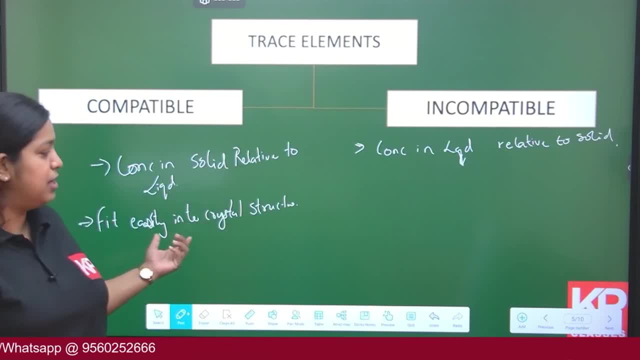 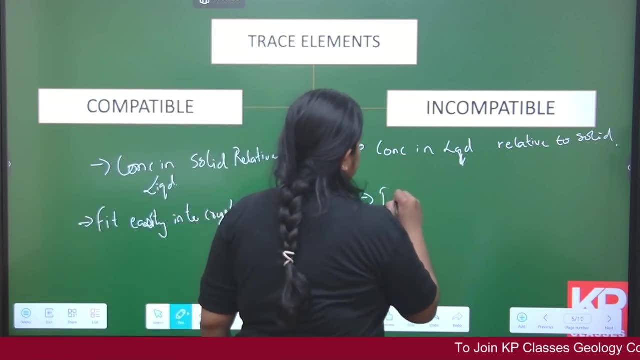 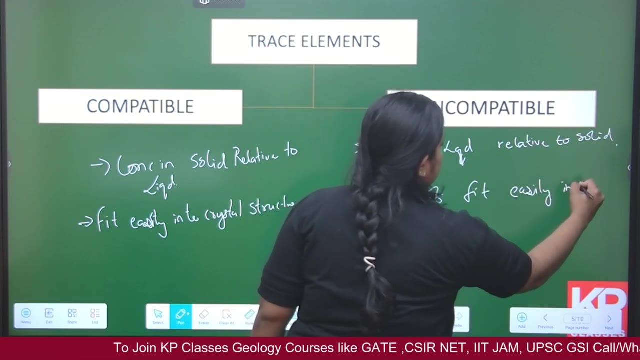 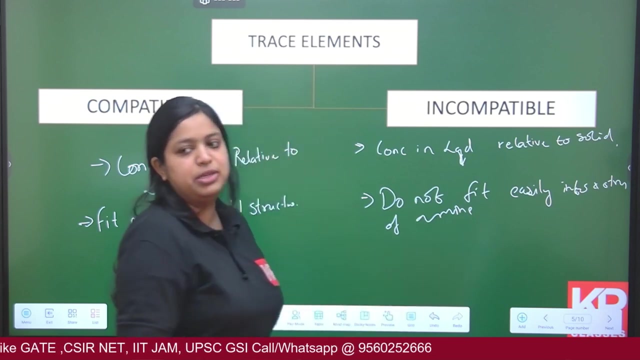 liquid. they can fit easily into the crystal structure, crystal structure of a mineral. okay, now when it comes to the incompatible elements. they do not easily fit into the crystal structure of a mineral, do not fit fit easily into crystal structure of a mineral, of a mineral. Now the incompatible elements. 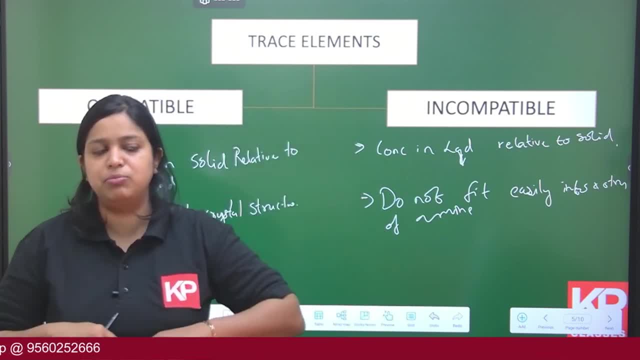 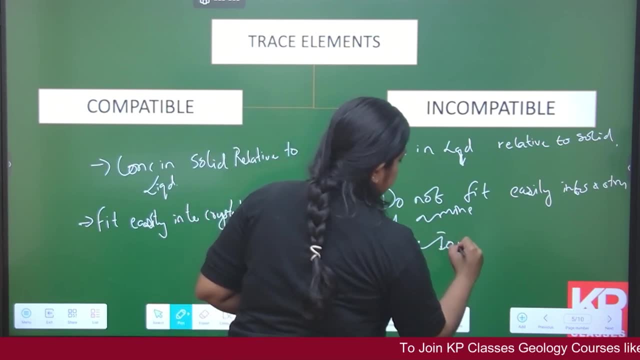 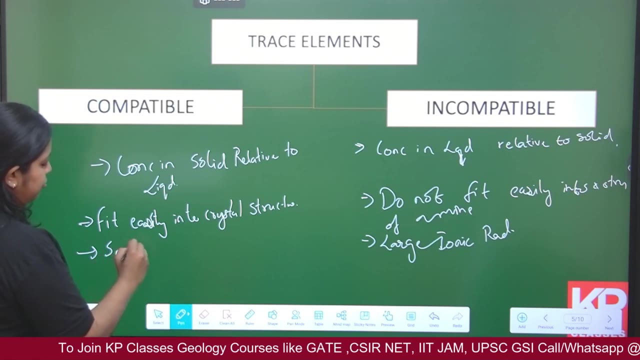 and compactible elements. incompatible elements are mostly must have large ionic radius, large ionic radius, whereas the compacted elements are mostly smaller, have small ionic radius, small ionic radius. Now the major, some of the most important or most common. 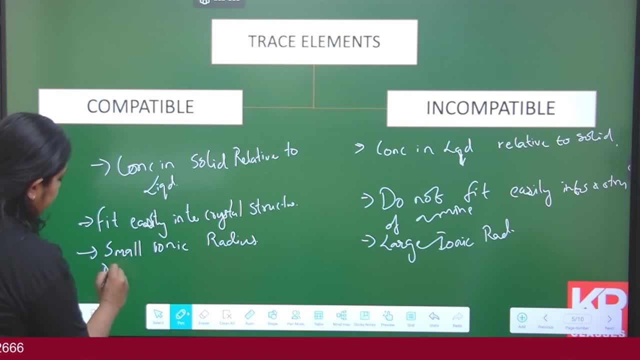 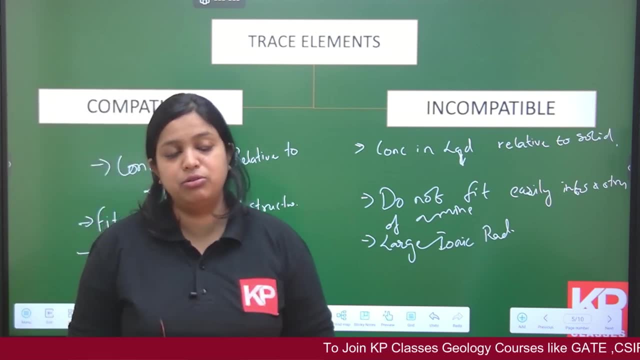 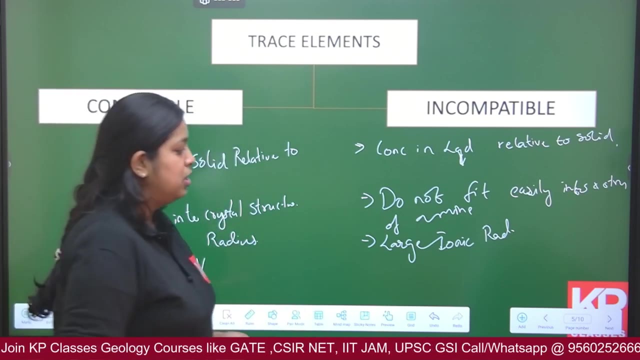 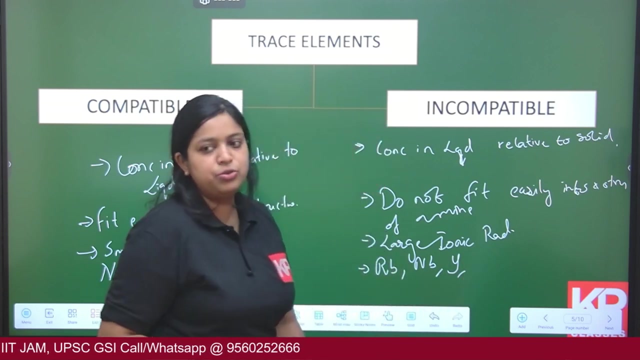 compactible elements are nickel, chromium, cobalt, vanadium, etc. These are the major. these are the more common compactible elements, whereas the common incompatible elements are rubidium niodymium yttrium, rubidium niodymium yttrium. 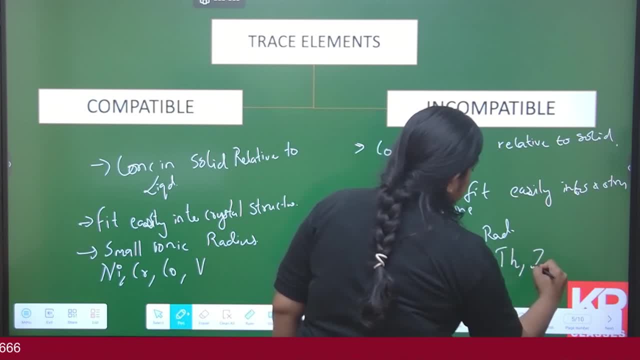 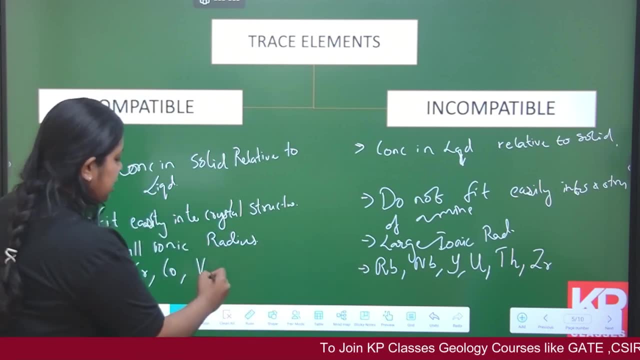 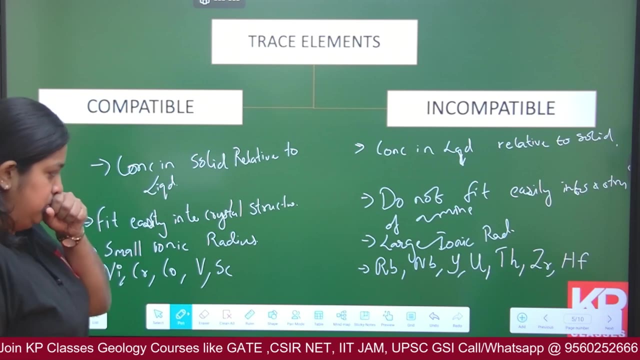 uranium, thorium, zircon, etc. All these are considered as the incompatible element. hafnium Here scantium, is also a compacted element. Compactible element can include hafnium also. Excuse me, Yeah, So this is the compactible. 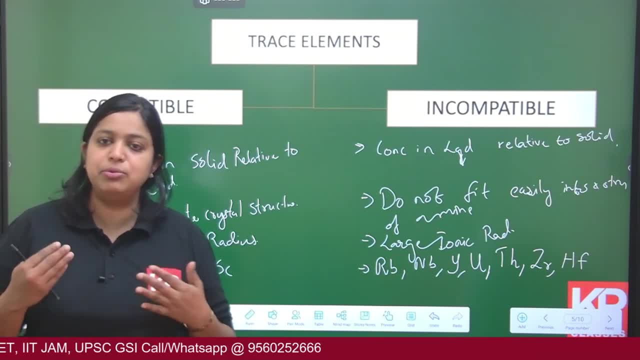 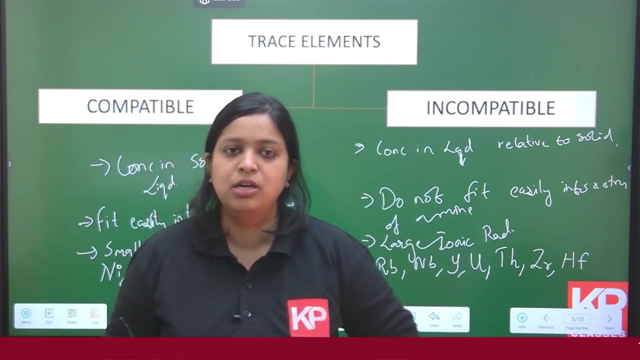 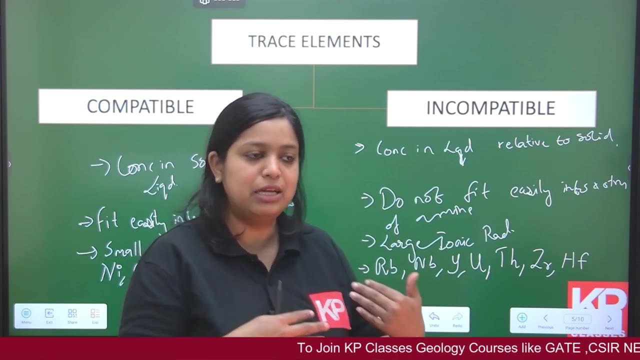 elements and incompatible elements. So trace elements can be divided into two on the basis of their affinity towards liquid or solid. Whenever magma crystallizes whether the trace element will prefer to go into the solid or whether the trace element will prefer to stay in the melt, Depending upon that, we can divide the trace element into two. 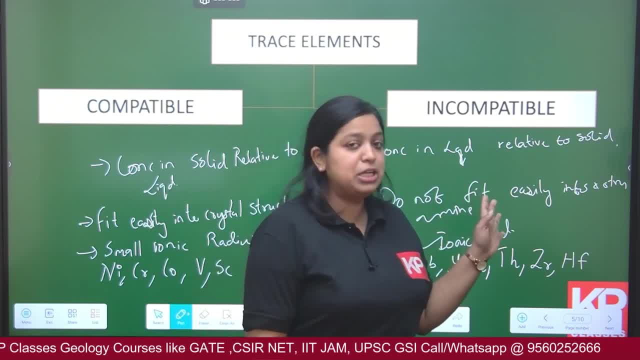 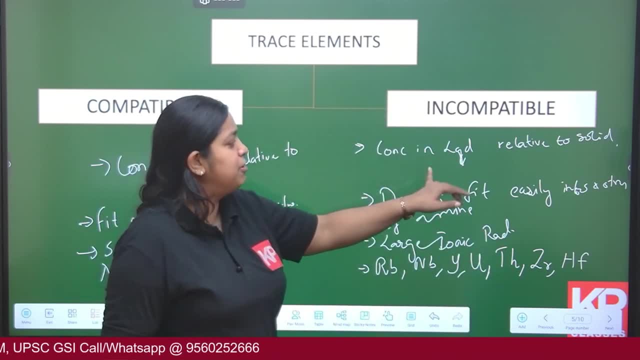 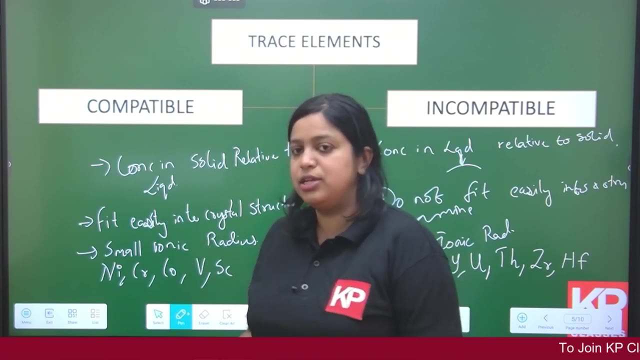 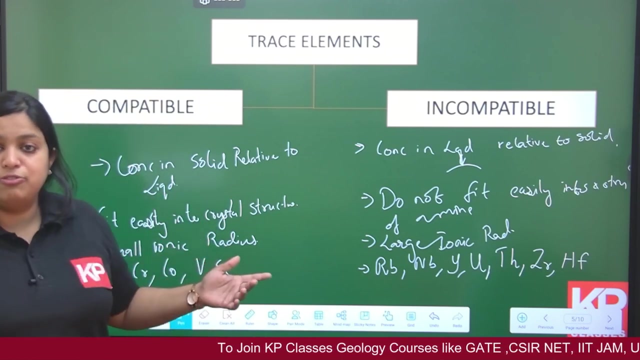 Incombat. sorry, compactible and incompatible trace elements. Compactible trace elements have concentration in solid relative to liquid. Incompatible trace elements have concentration in liquid relative to solid. The compactible ones fit easily into the crystal structure. incompatible elements do not fit easily into the crystal structure of minerals. Now compactible: ones comparatively smaller ionic radius, whereas it can. Studọito Solid is the alsoacióng there is aいるk to, I think, toietnamium- This is mine- and then the abouriteAg polymer, eurum toionalial, is taking In combatible elements, theschaftible elements in lead would 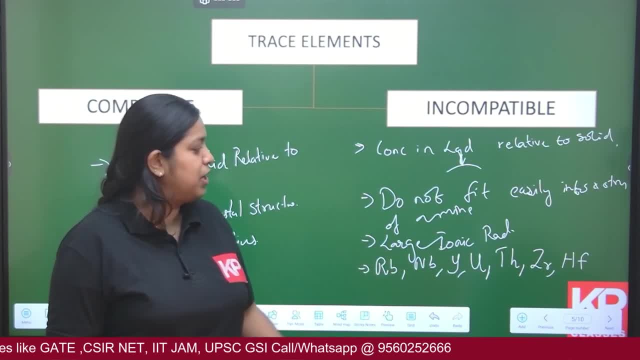 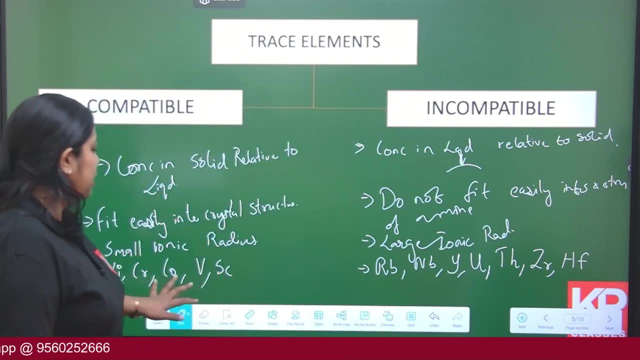 Solute and this oxide is lead. So this is takingAlso winning iron. we parle of ،because we would- whereas most of the incompatible elements have larger ionic radius and has provided the most some of the important ah compactible and incompatible elements. 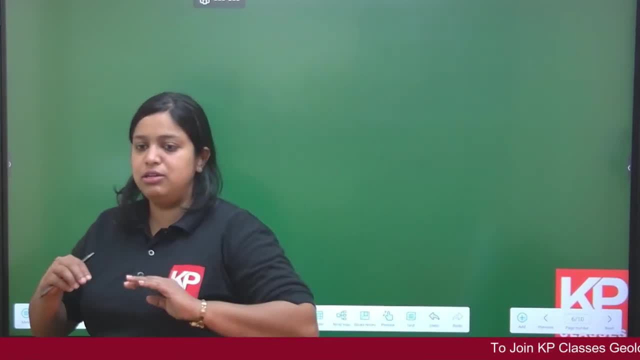 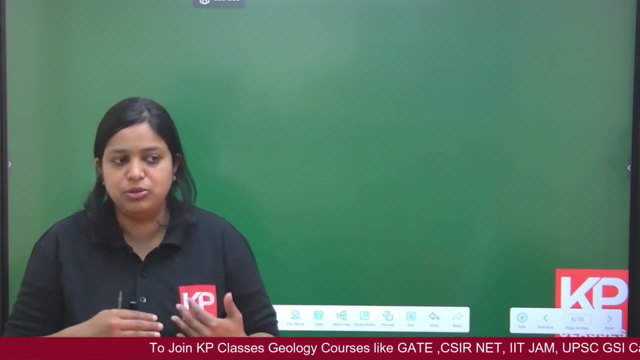 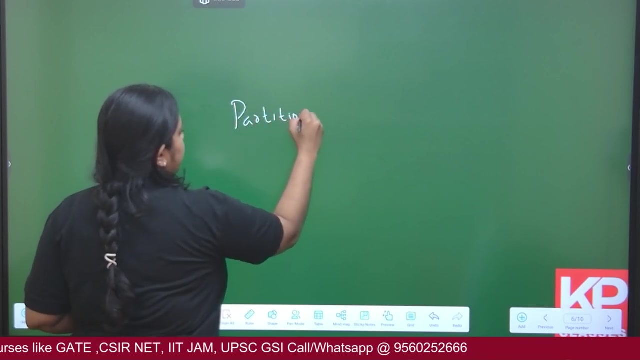 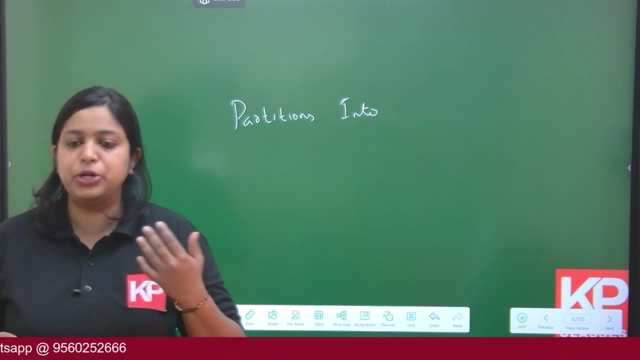 Now, when it comes to ah, the like ah, each element, each trace element, there is an its efficiency to an element like ah. efficiency to an element to in partitions, into efficiency of an element to get partitioned into a particular phase. ah, whether it will go to other ah magma. 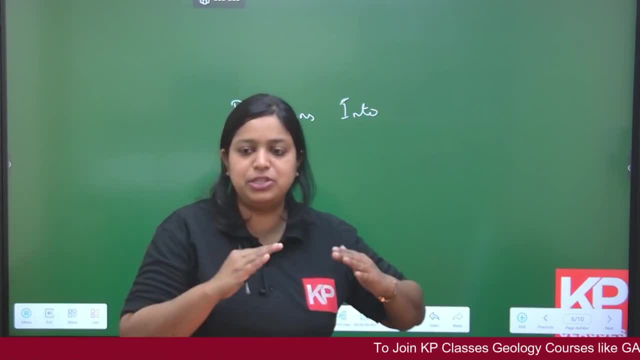 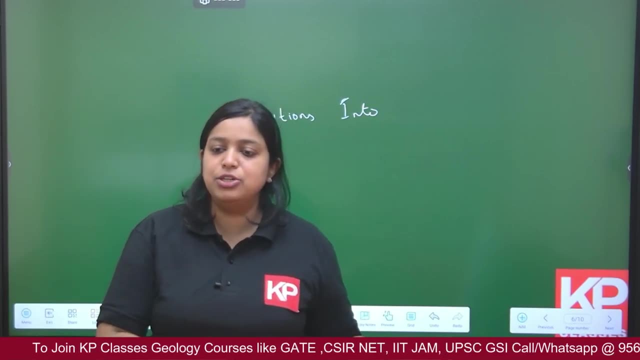 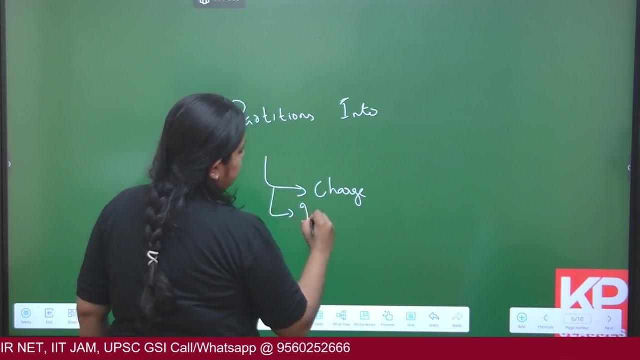 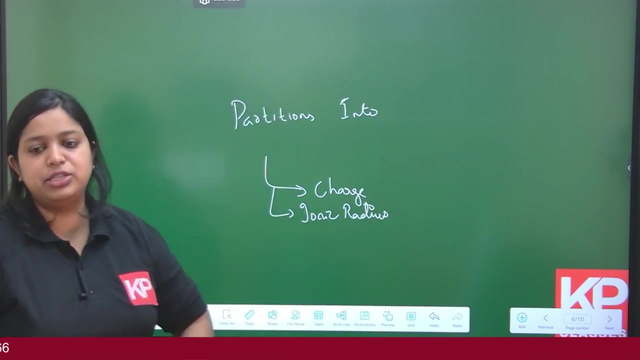 stage, the liquid stage, or whether it will go to the solid, say its efficiency to get partitions, partition, partition, sorry, Partitioned into a particular phase, into a particular phase, is controlled by charge and ionic radius. charge and ionic radius, So these are the two conditions, like charge valency of the element or the ionic radius of 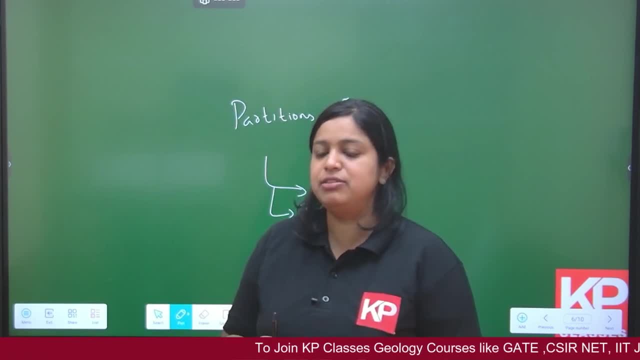 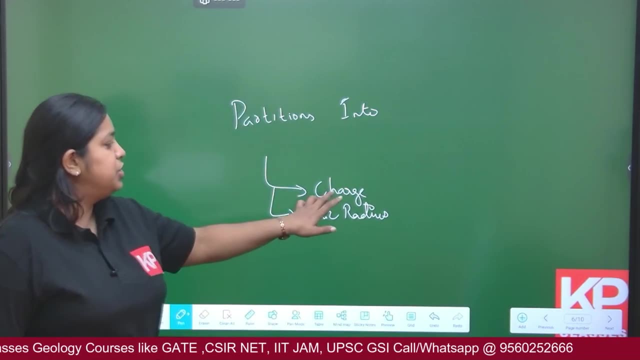 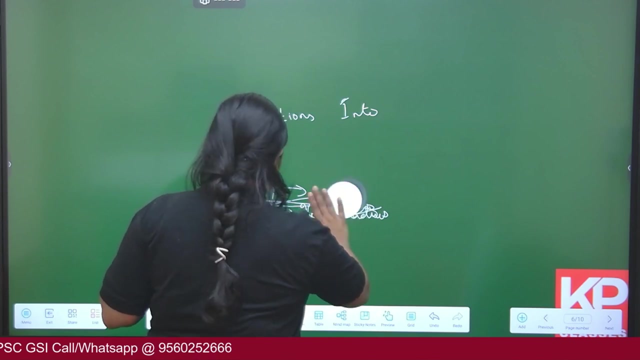 the element. These two terminologies defines the efficiency of an element, efficiency to which an element partitions into a particular phase, and that is controlled by charge and ionic radius of the element. So so how can we predict? So, if I have two elements, are there? 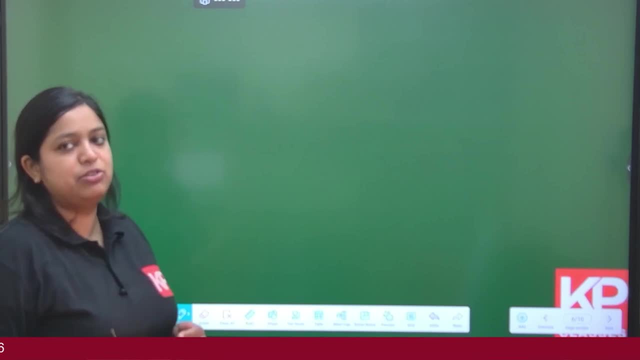 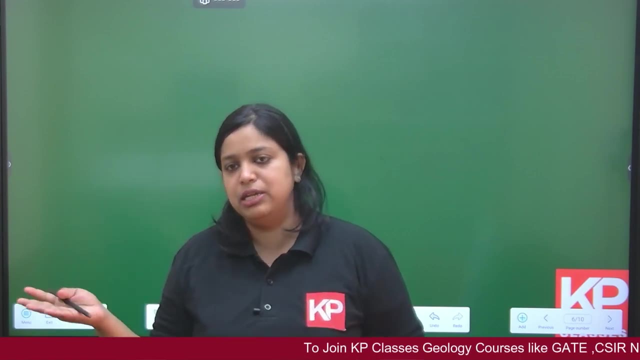 two different types of elements are there. So how can I say like which one will stay in the magma, which one will go to the mineral structure? So how can we predict? So this, how the trace elements behavior, or the trace elements behavior of the element is controlled by charge and ionic radius of the element. 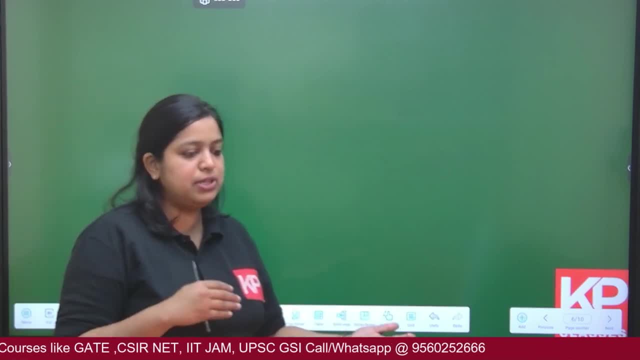 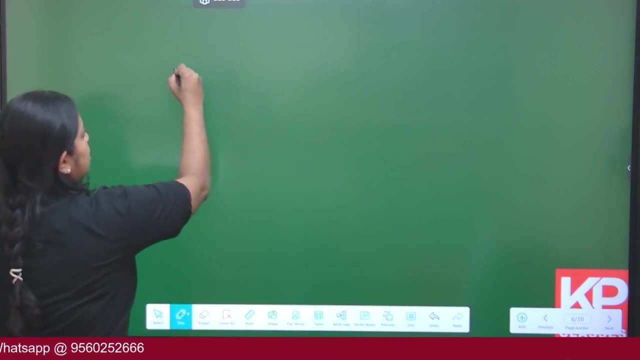 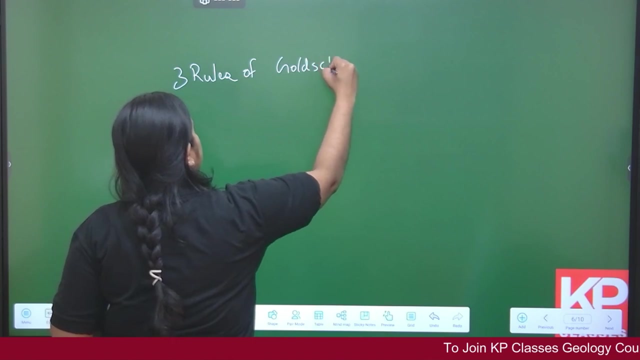 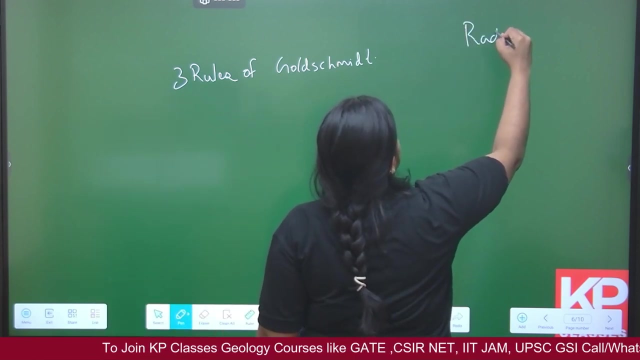 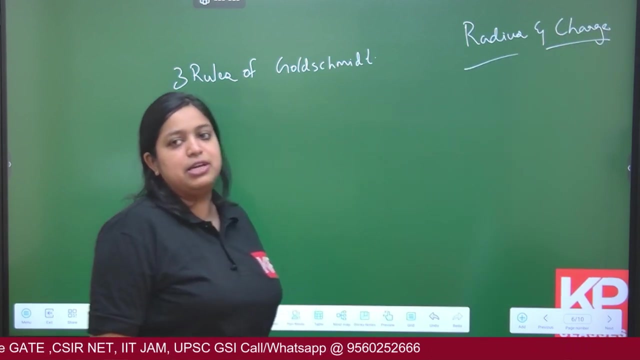 So the trace elements- affinities to liquid state or to solid state- is defined by Gauss-Schmidt's three rules. So this is based on, as I said, radius, and radius and charges are the two factors that defines the efficiency of an element to partition, get into a partition into. 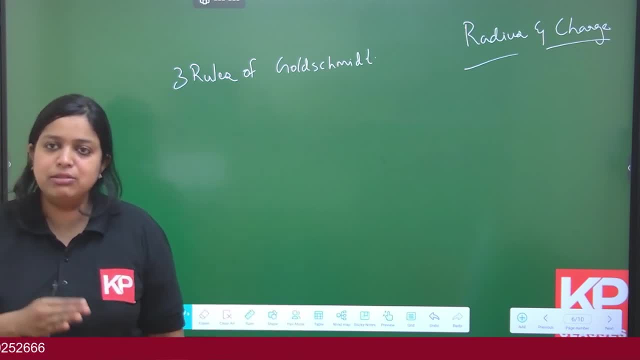 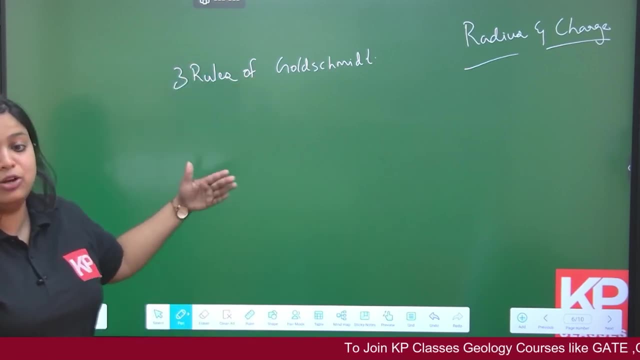 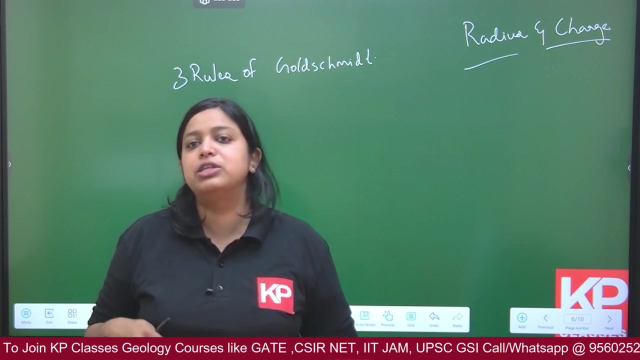 a crystal structure or to stay back in the magma. So this is defined by the radius and charge of the element. Now Gauss-Schmidt has defined three rules. depending upon the radius and charge, what will happen to the trace element, whether it will stay in the melt or whether it will go. 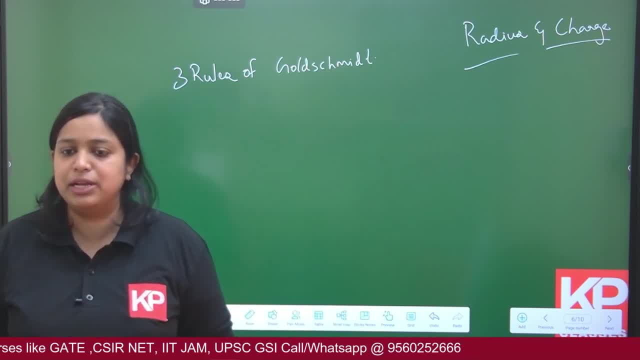 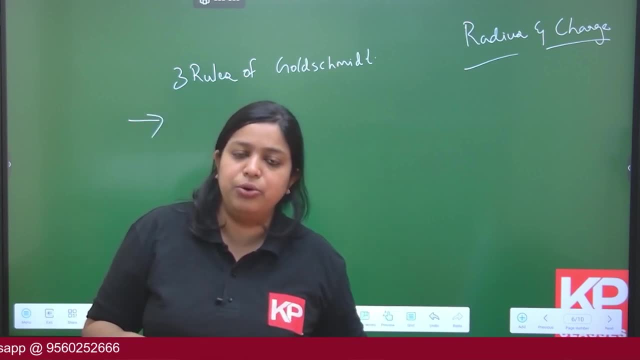 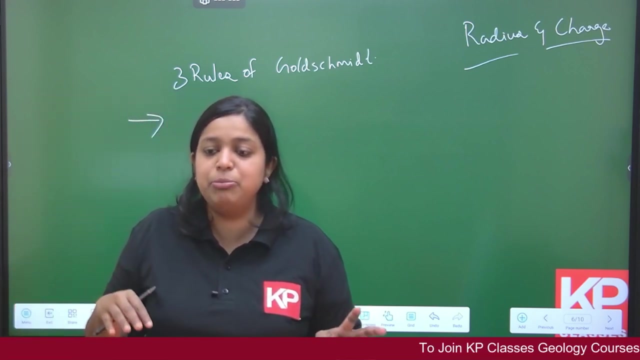 into the in the crystallizing phase, whether it will get into the mineral structure. So first one is: if two elements have same in ionic radius and same valency, same charge, So what will happen to two elements that have same ionic radius and same charge? They behave. 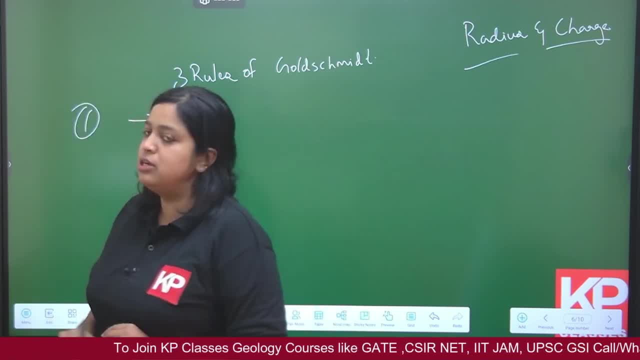 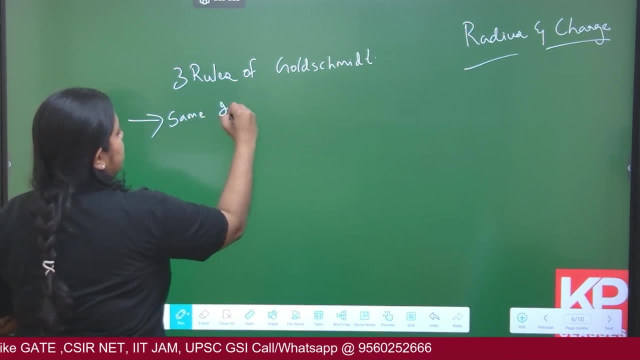 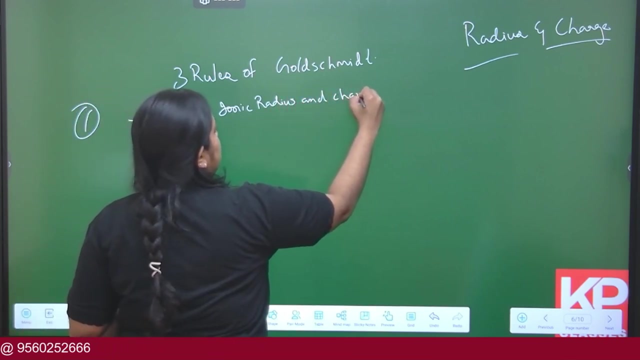 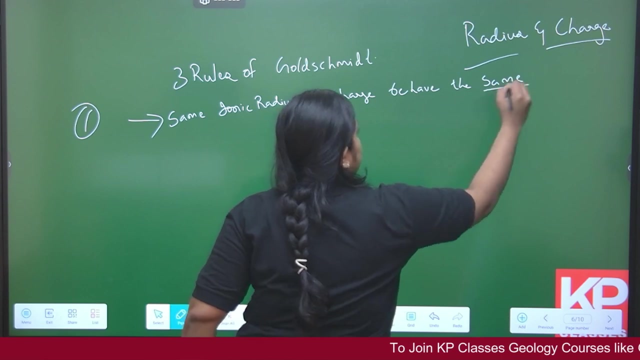 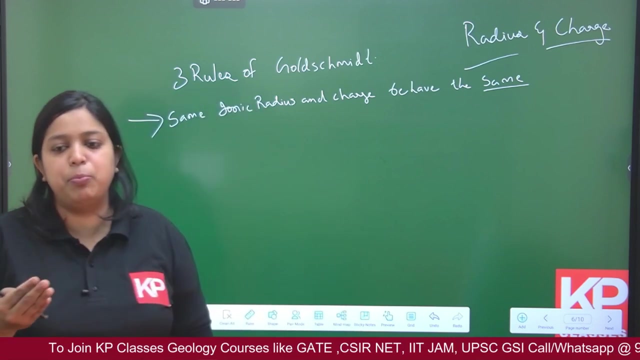 the same. That is what the first rule of Gauss-Schmidt says: that two ions with same ionic radius, same ionic radius and charge behave the same. They behave the same. So what will happen? when they behave the same, They will be entering like in the same proportion. they will enter into a. 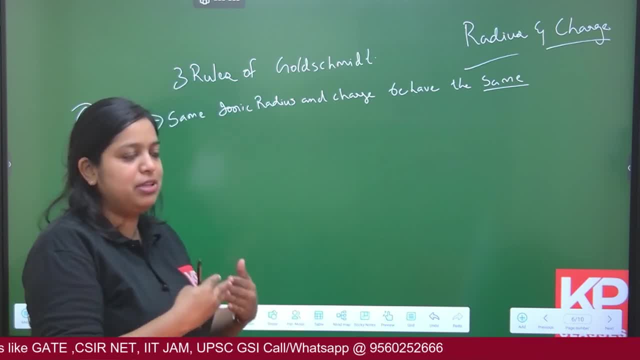 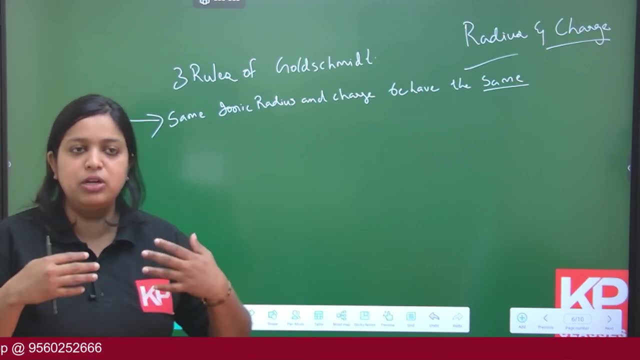 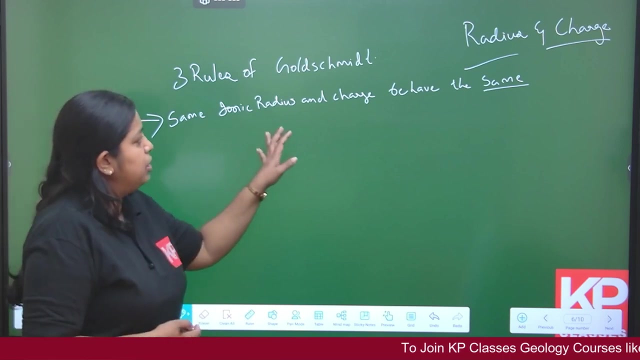 mineral structure, Like if both of them have the same behavior, then both elements will get into 50-50 percentage or 25-25 percentage whatever, in equal way or in the same way they behave, or they will get into the, a crystal structure. So this particular behavior or this particular substitution is called as. 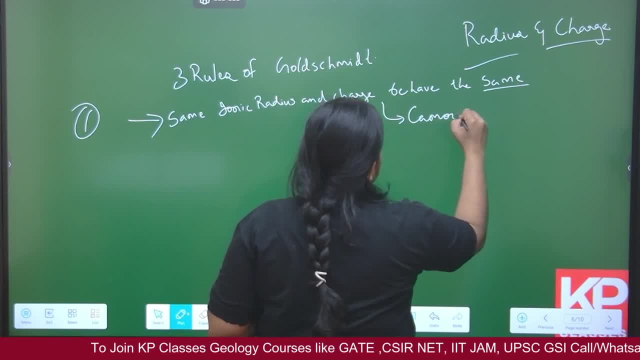 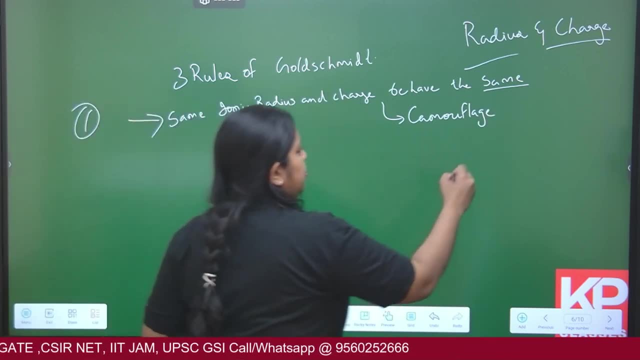 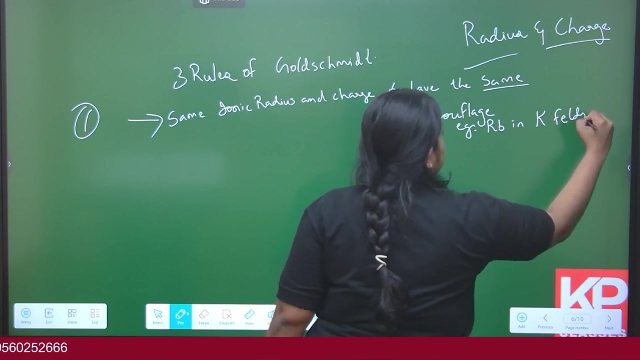 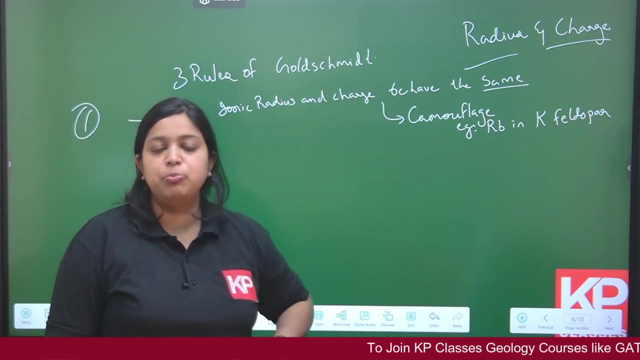 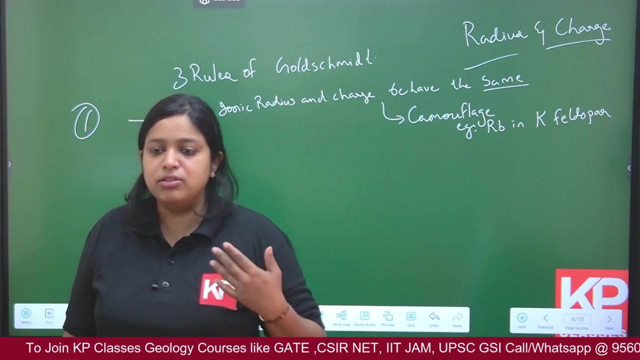 camouflage substitution. Camouflage substitution: Major example is rubidium in potassium feldspar, Rubidium in potassium feldspar. So what happens is rubidium and potassium. both have similar ionic radius and similar charge, So both behave the same. So hence rubidium can. 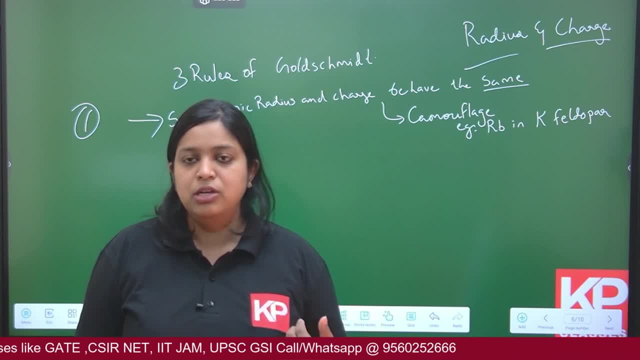 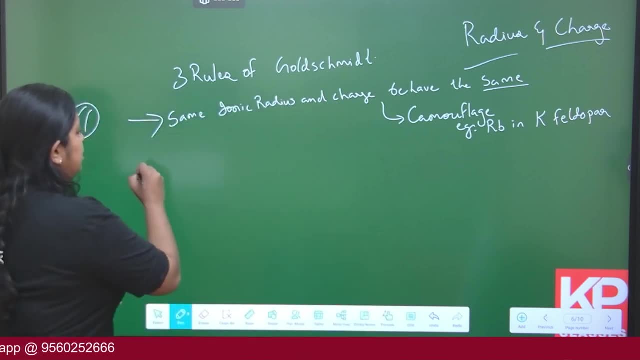 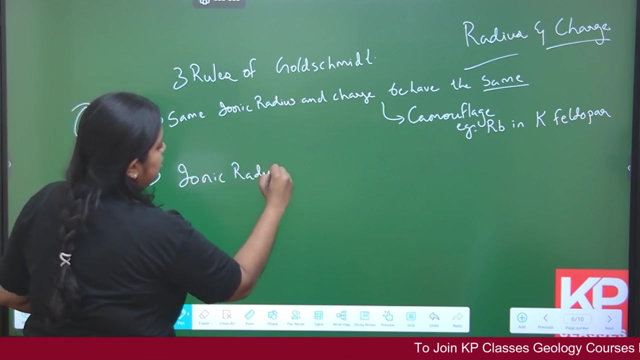 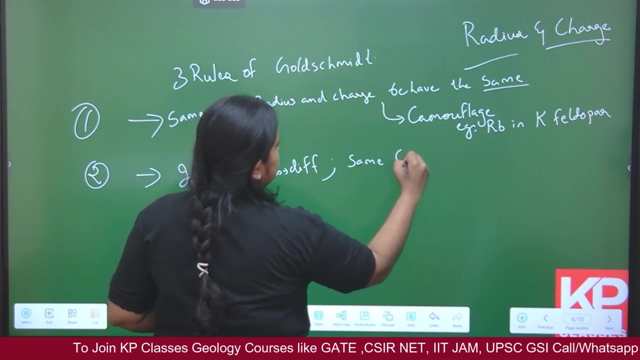 substitute potassium in the potassium feldspars. So camouflage substitution happens to rubidium in the potassium feldspars. Now next, let us see So second case, where the ionic radius is different. Different ionic radius, same charge. 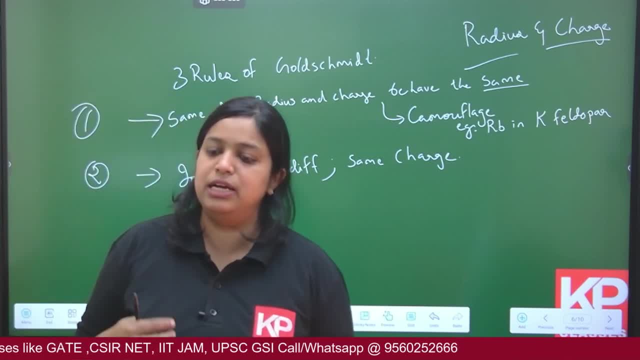 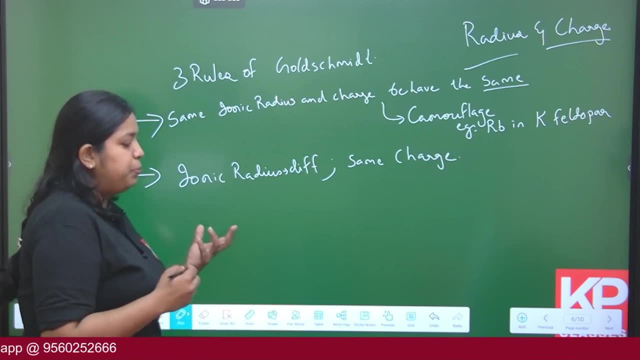 Two elements that has different ionic radius and same charge condition. So what will happen to this case? The larger one will prefer, the larger the ionic radius, whichever which element has a larger ionic radius. So the larger the ionic radius, the larger the ionic radius, the larger the 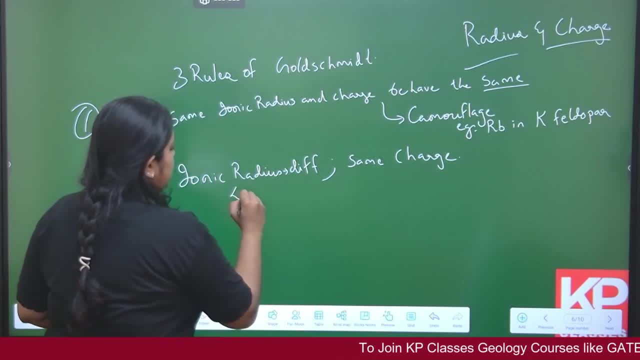 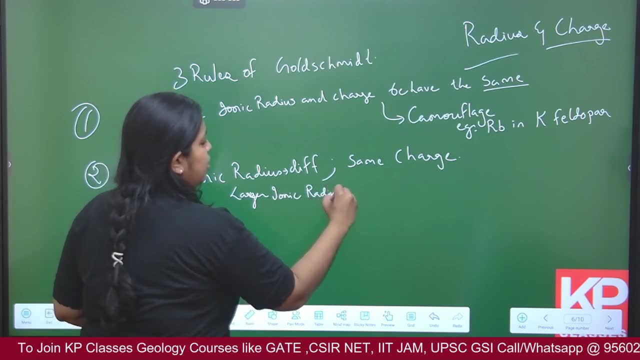 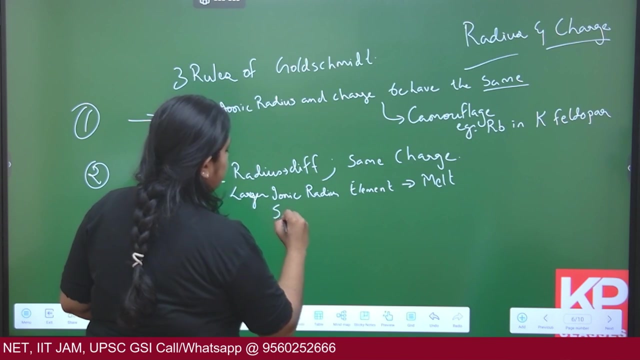 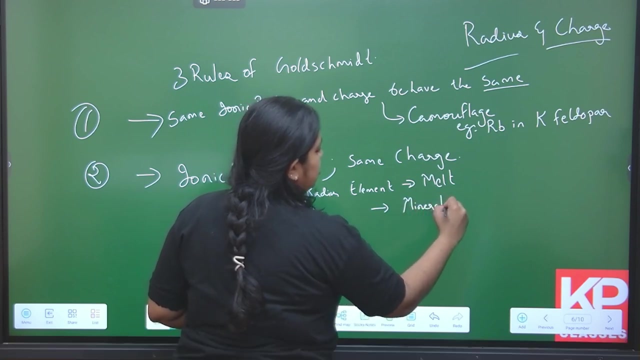 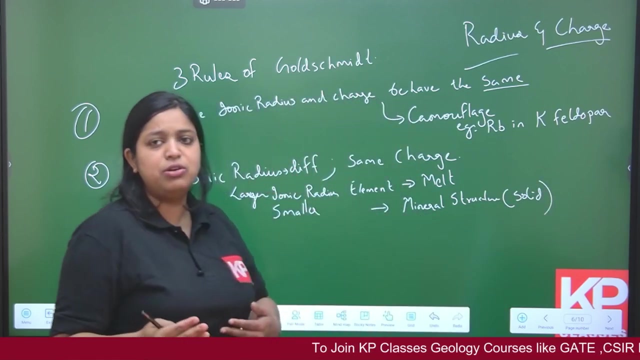 ionic radius, they will prefer to stay in the melt. Larger ionic radius element will prefer to stay in the melt, whereas the smaller one. smaller ionic radius element- will prefer to go into the mineral structure. Mineral structure means solid, Simple. Larger one, it is easier to crystallize the smaller one, It is easier for a smaller element. 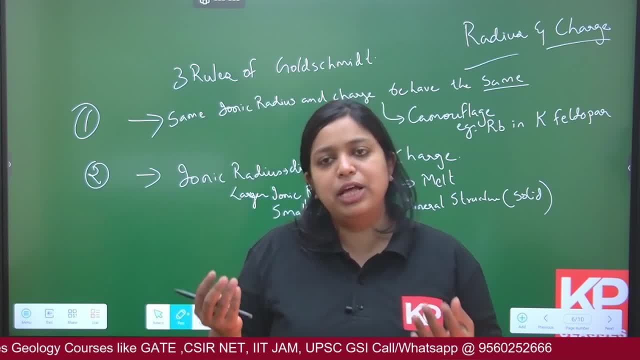 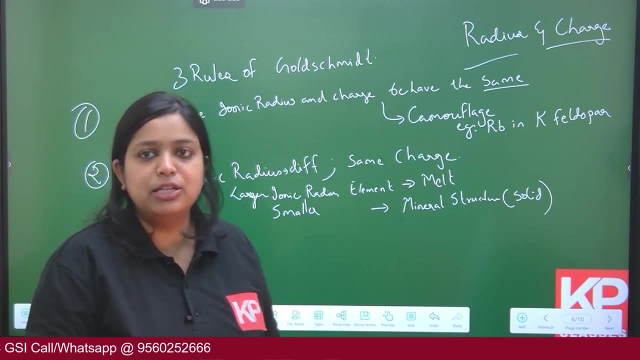 to fit into a crystal structure. So even though if both elements have same ionic charge, one will be getting into or one can incorporate the other one, For example strontium and rubidium Strontium rubidium, both have same. 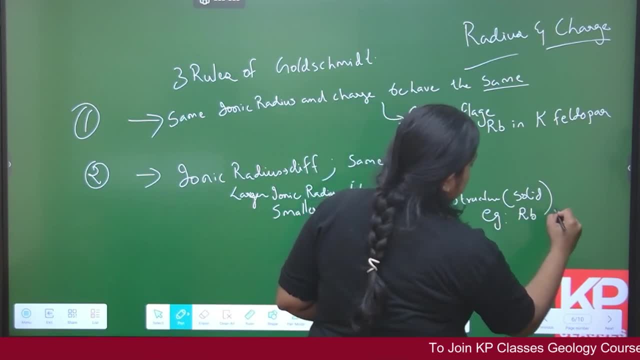 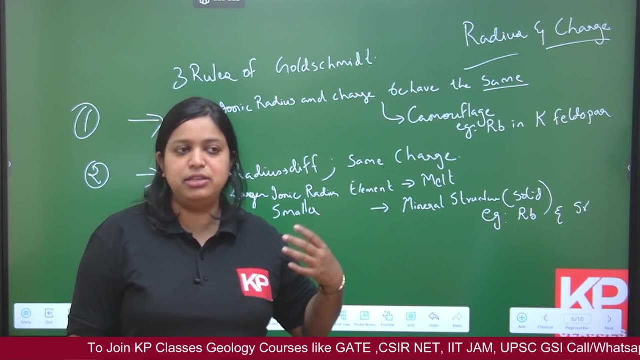 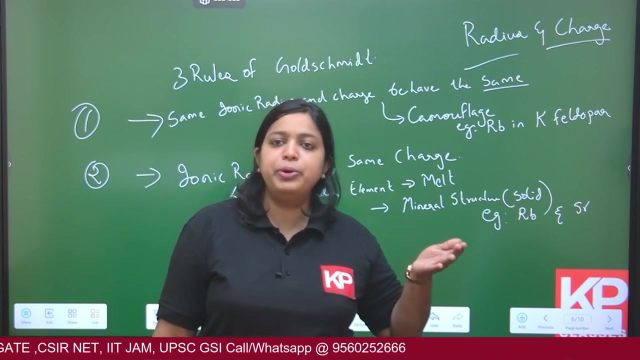 rubidium and strontium. Both have same charge, But rubidium has higher ionic radius. It is much more larger than larger ionic radius than the strontium. So what happens When crystallization occurs? rubidium will prefer to stay in the melt. 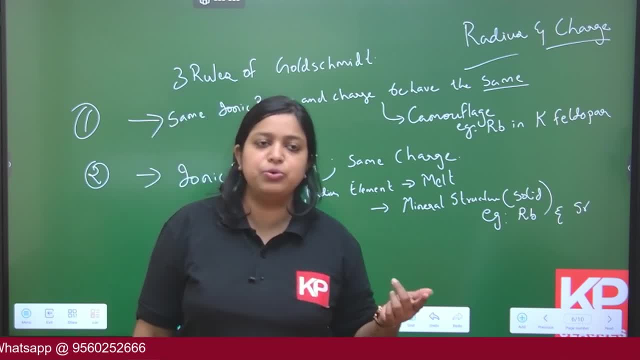 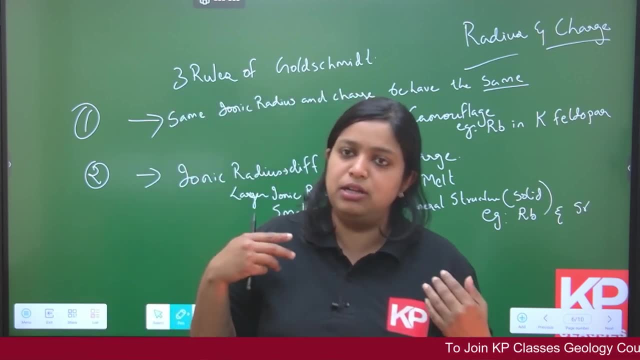 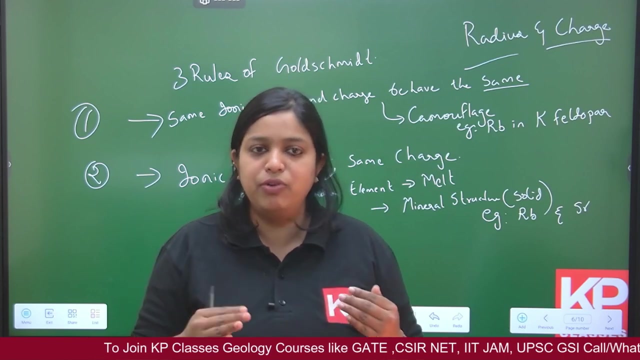 comparing with strontium: Strontium will prefer to get into the. when you compare with rubidium and strontium strontium, both of them has same charge. Strontium has lesser size or the ionic radius is smaller, So strontium can will be crystallizing. more will get into mineral. 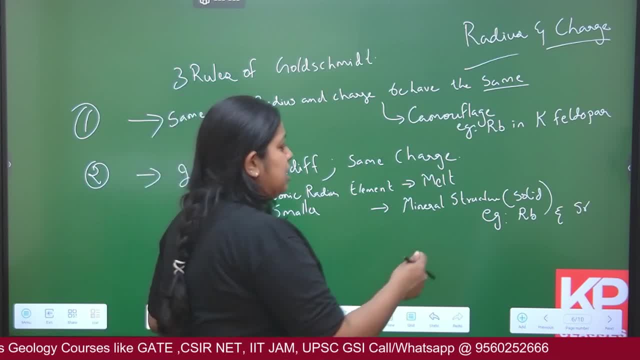 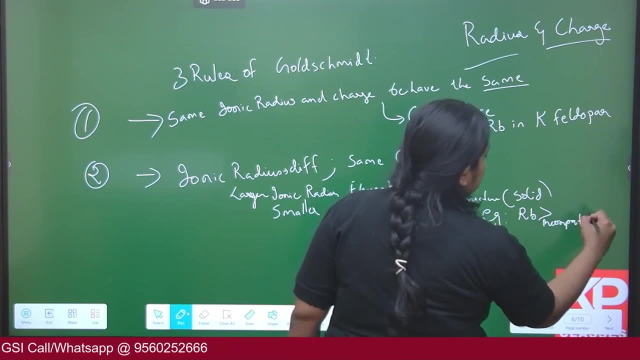 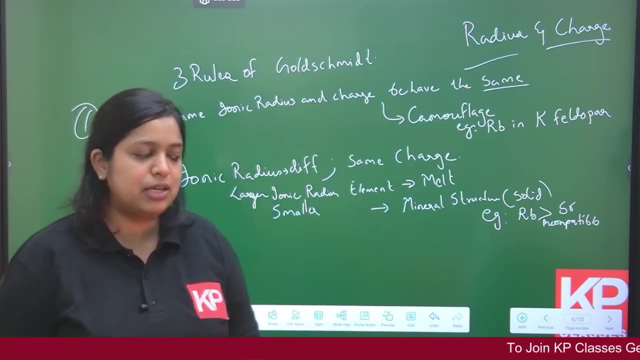 More than that of rubidium. So we can say that the rubidium is more incompatible than more incompatible than strontium. Rubidium is more incompatible than strontium. Okay, Now the next case is the third rule, defining So what is left First. we say both. 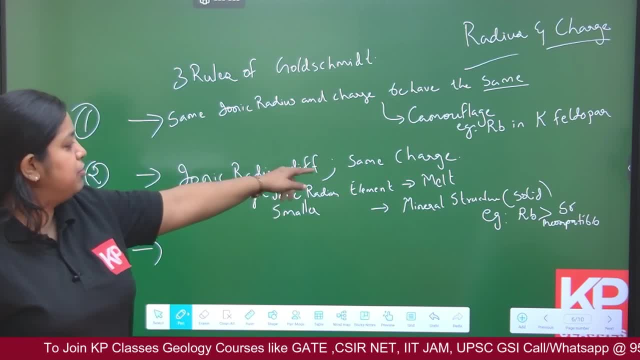 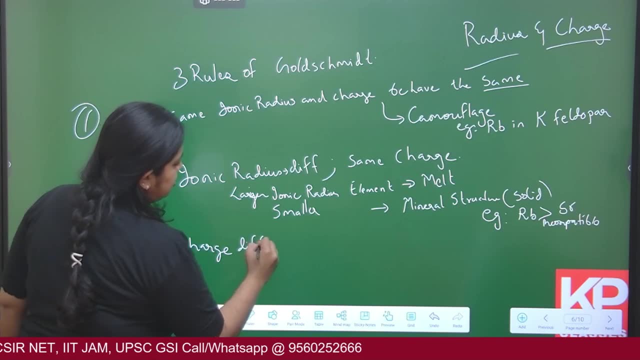 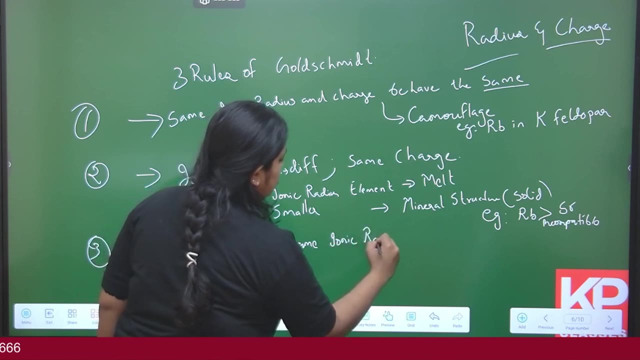 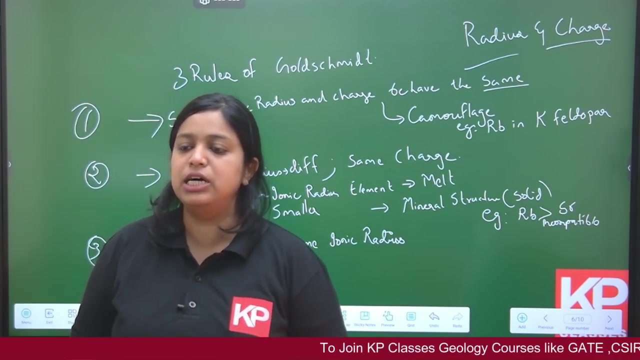 radius and charge are equal, Then if ionic radius is different, charge is same. Now, obviously, charge is different. Two elements that has different charge, but same ionic radius or same size. So what will happen in this case? Here, higher the charge element, the element that has 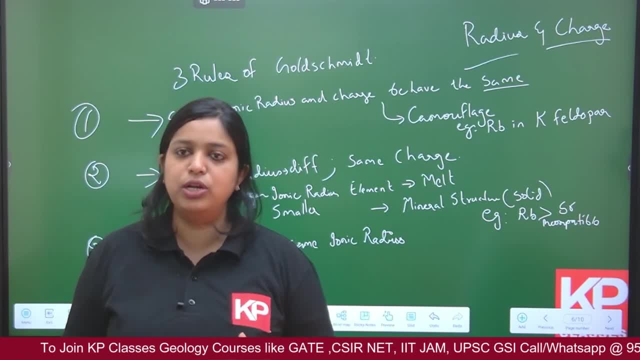 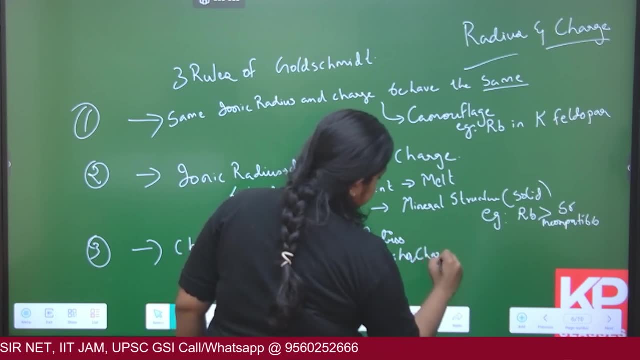 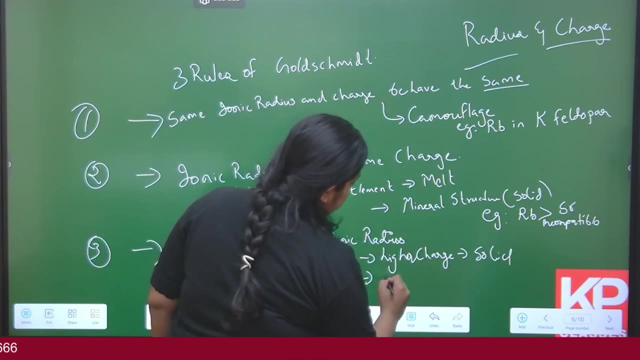 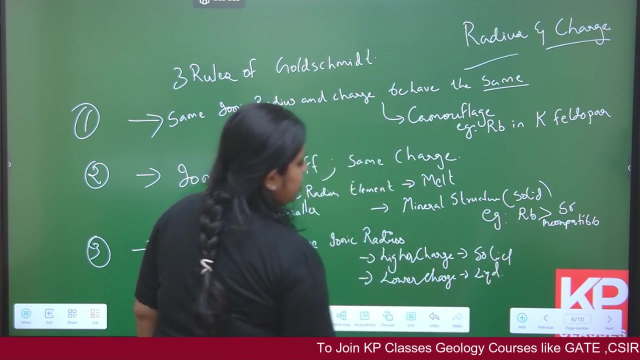 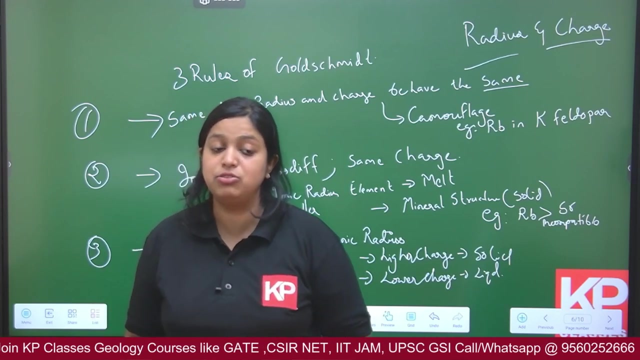 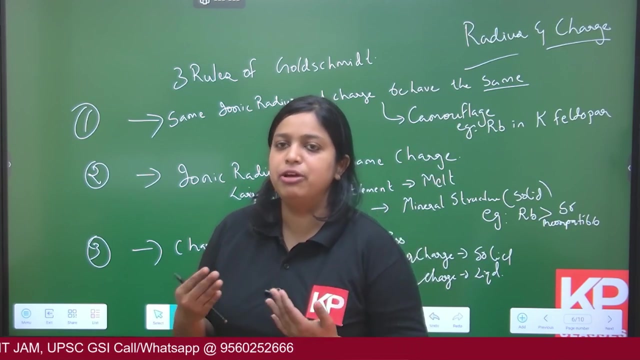 that have higher charge will get into the solid over liquid. Higher charge, one will get into the solid, Lower charge will get into the liquid. Okay, So these are the three rules defining the trace elements: affinity, affinities towards liquid state and the solid state, whether they behave compatible or whether they behave. 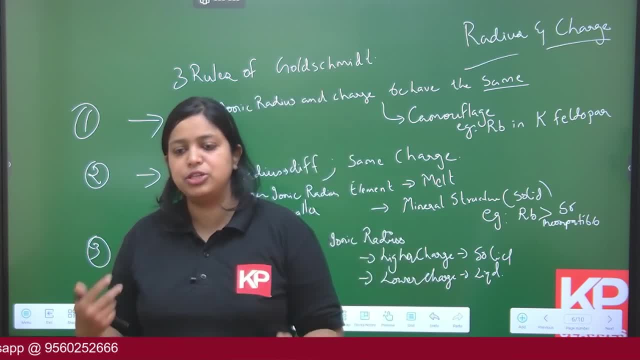 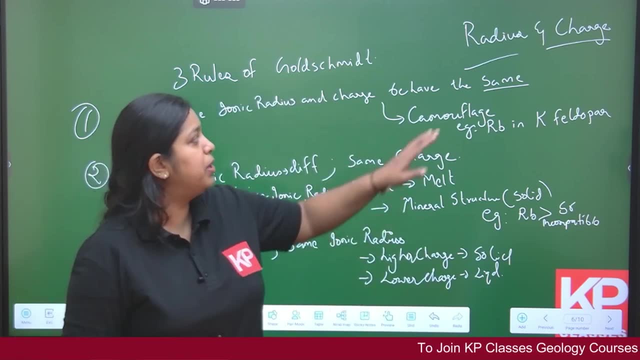 incompatible. So let us see the third rule. So let us see the third rule. So let us see the third rule. that is defined by the three rules. and it is actually defined. the efficiency of a trace element to get partitioned into a particular phase is controlled by radius and charge. 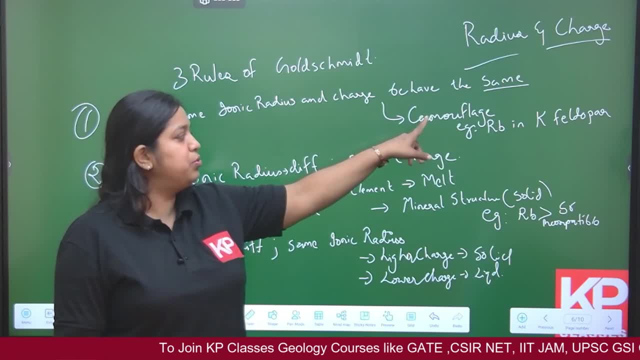 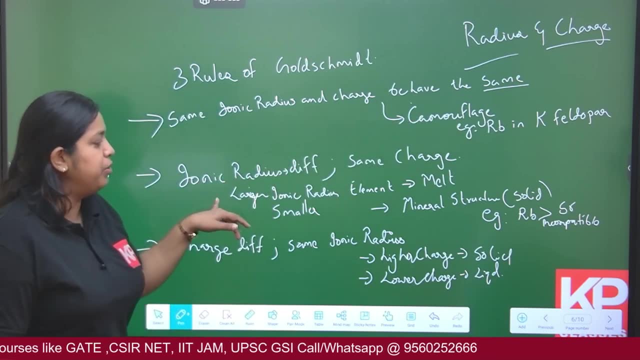 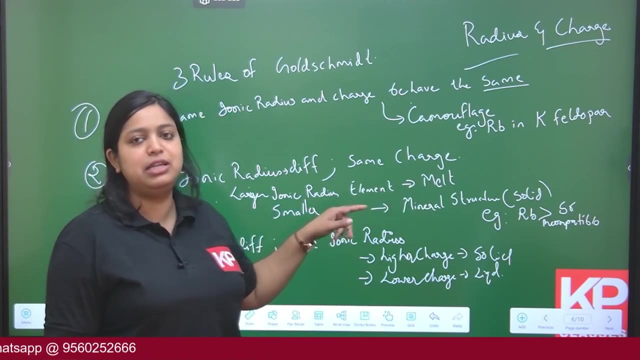 Hence, if both of them have same radius, one will substitute the other. that is the camouflage substitution. both of them will behave the same. If ionic radius is different and the charge are same, then the larger ionic radius element will stay in the melt. smaller one will stay in the 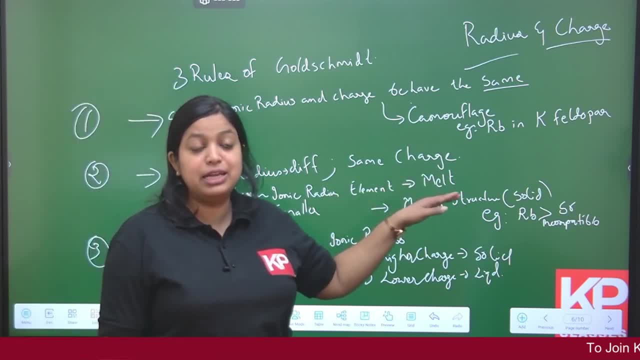 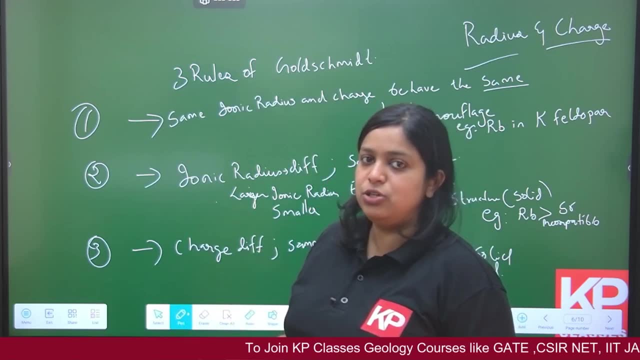 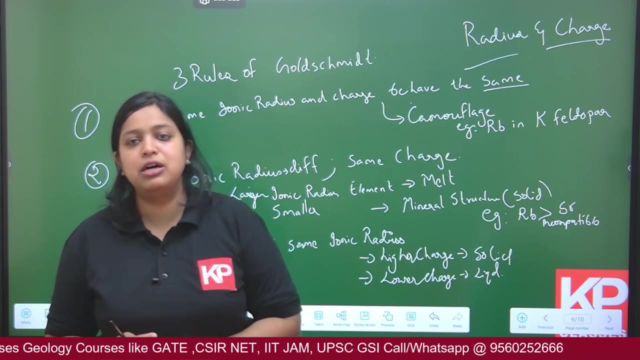 liquid state. Sorry, smaller one will stay in the mineral, can get into the mineral structure or the smaller one can participate in the crystallization of a mineral. Third one: if the charge is different and it has the same ionic radius, higher the charge will stay in the solid, lower the charge. 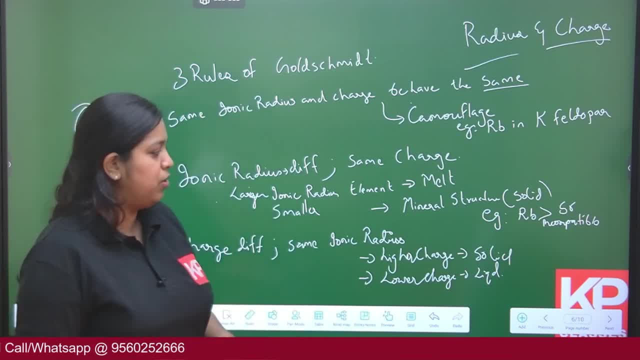 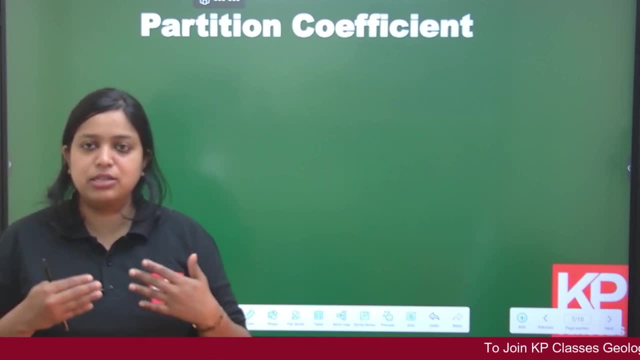 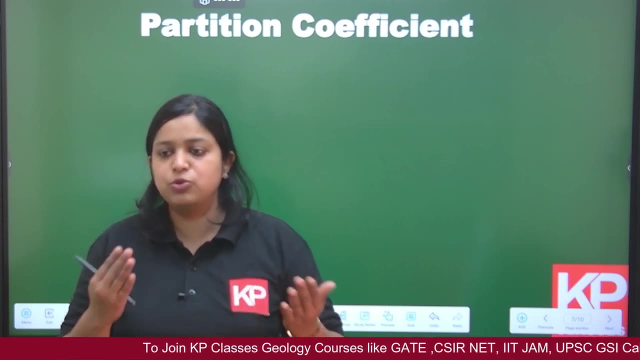 will stay with the magma. Okay, So now to quantify this MO like how partitioned, happening, a trace element, how, what is the value of its incompatibility or what is the value of its compactibility? So to quantify that, we have come up with a terminology called as partition. 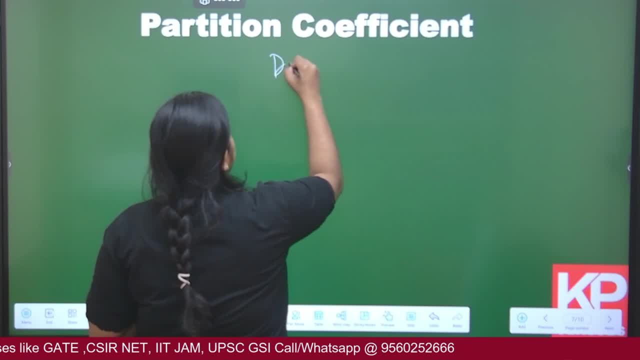 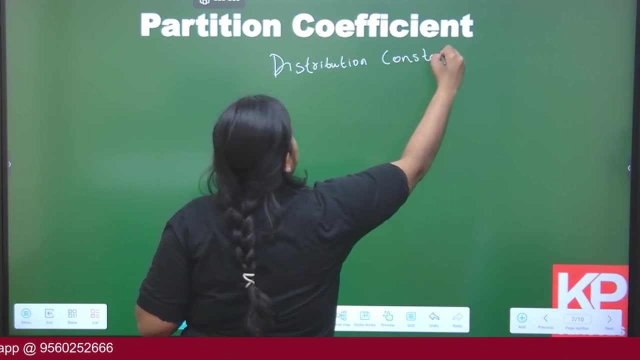 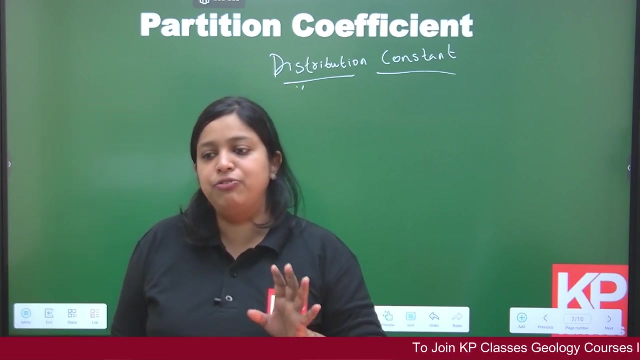 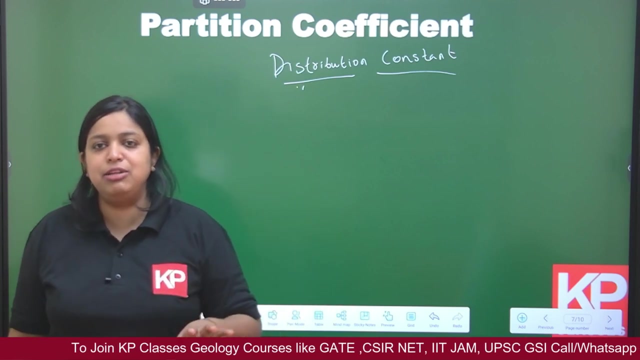 coefficient, or it is also called as distribution constant, Partition coefficient or distribution constant simple. The chemical fractionation of a trace element is called as partition coefficient, So this is called as partition coefficient Of an element is unevenly under equilibrium condition and that is defined by partition. 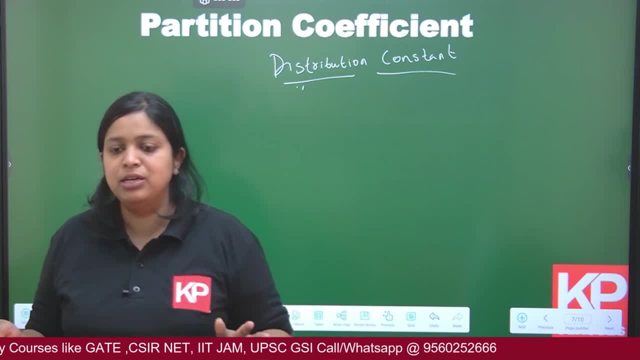 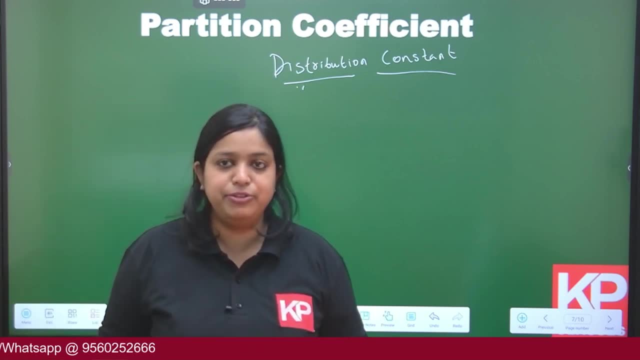 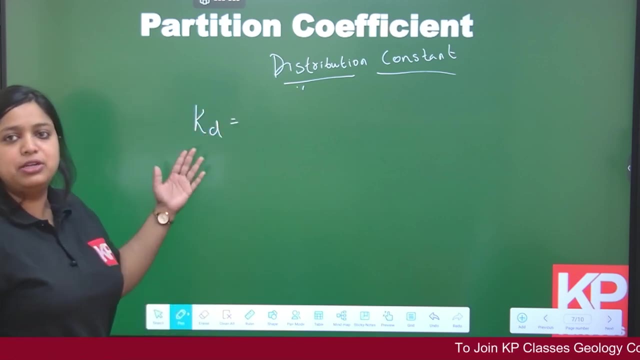 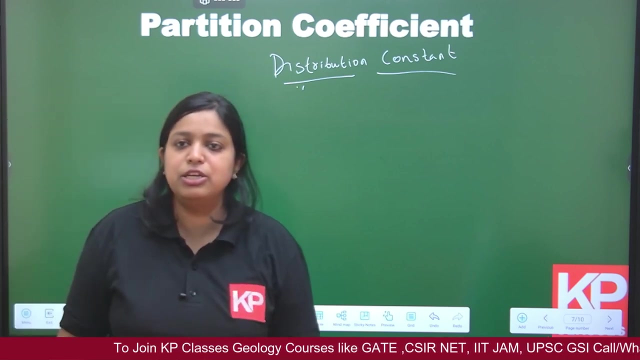 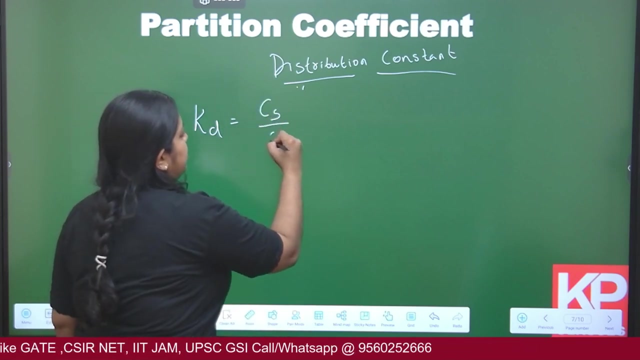 coefficient. Chemical fractionation of an element unevenly under equilibrium condition is defined by partition coefficient or distribution constant, which is notated by the letter KD. In different textbooks they uses different way to represent the terminology partition coefficient or distribution constant. Here I use the term KD terminology. Now, KD is equal to CS divided by CL. 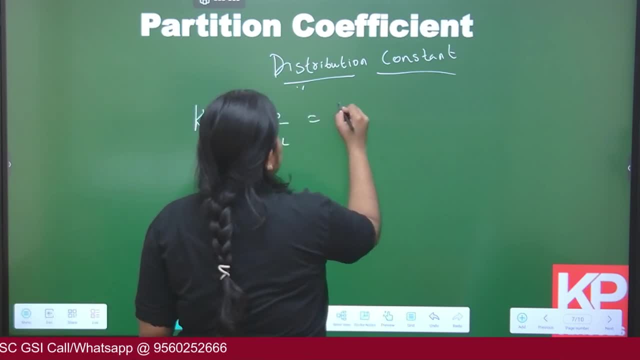 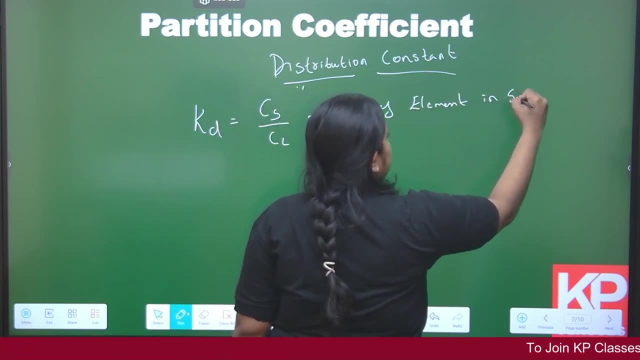 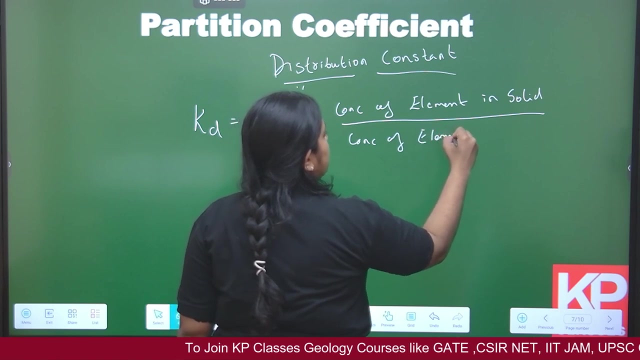 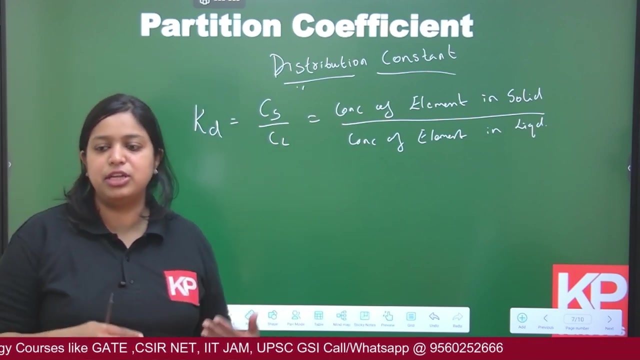 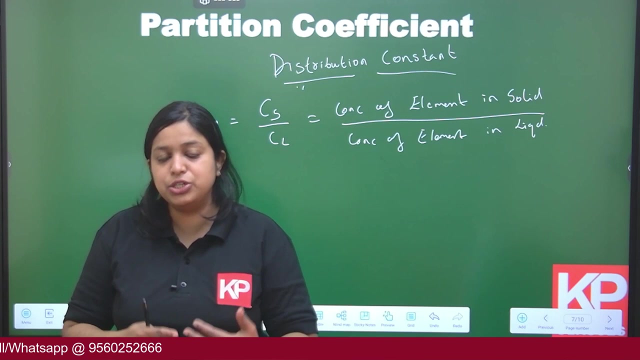 Whereas CS is the concentration of a particular element in solid divided by concentration of that same element in liquid. This is this is what is called as partition coefficient, So it is a ratio of concentration of an element in solid phase to that of that same element in concentration of that same element in. 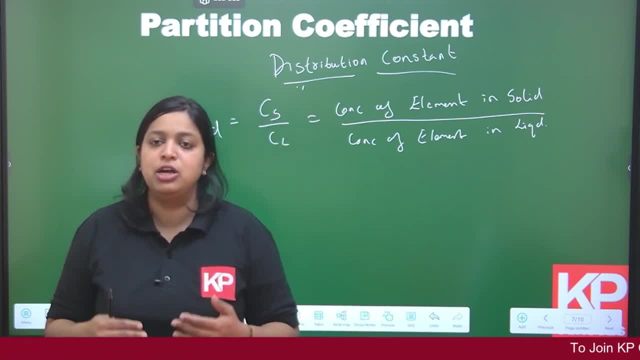 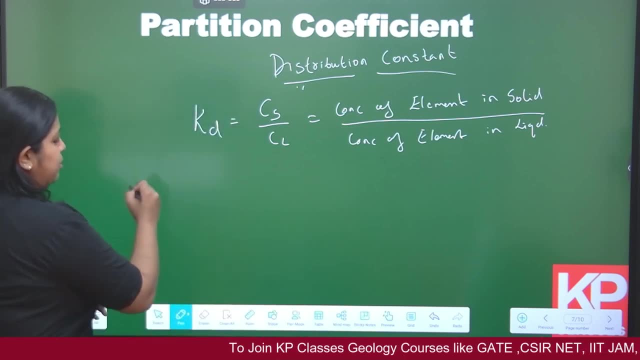 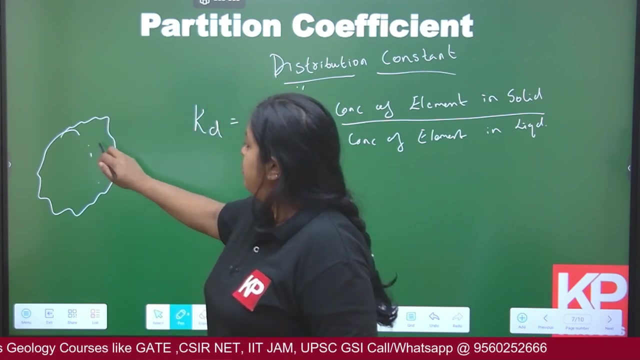 the liquid phase. This is called as partition coefficient or distribution coefficient, distribution constant. Simply, when a mineral crystallizes, if I have a magma, if there is a magma present, a liquid magma, and from this magma a particular crystal started crystallizing. Now, when this crystallization of this mineral, 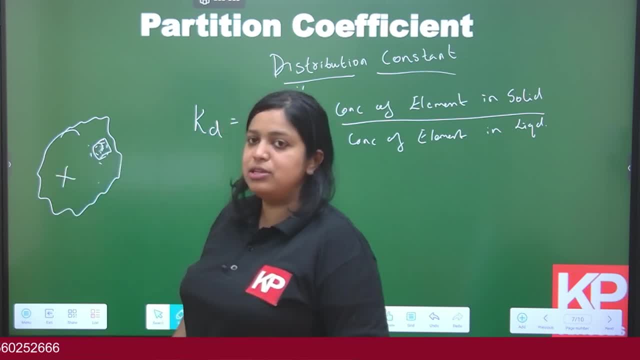 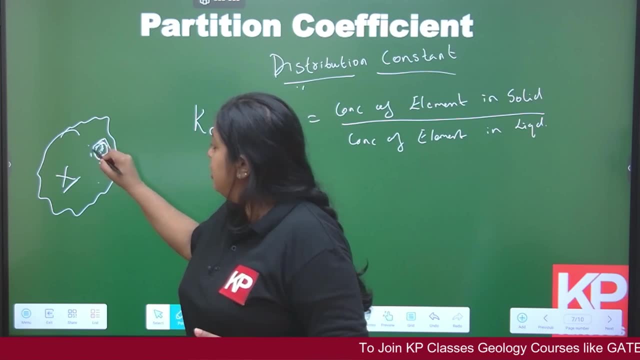 happened if, for example, there is an element called as X. So I should know whether this element is compactable in this mineral or whether it is incompactable in this mineral. So what I will do after crystallization of this mineral I, I will check the concentration. 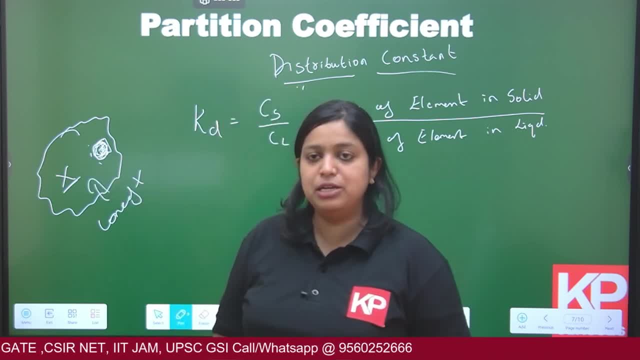 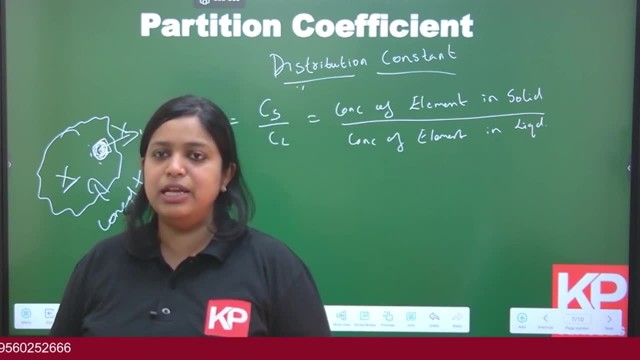 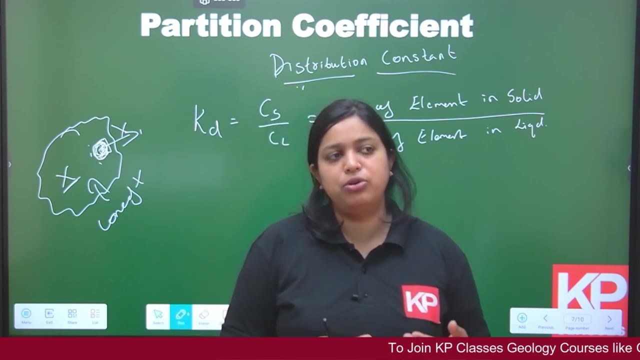 of X in the melt, the residue, the melt. So for trace elements, trace elements analysis is mainly done by spectroscopy. So there are XRD, XRF, there are so many spectroscopies which will we can do on our rock samples that will give the 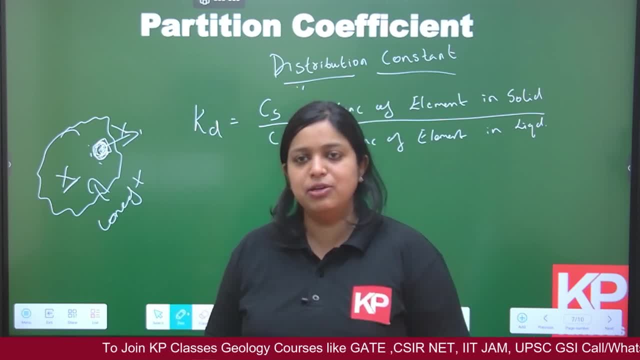 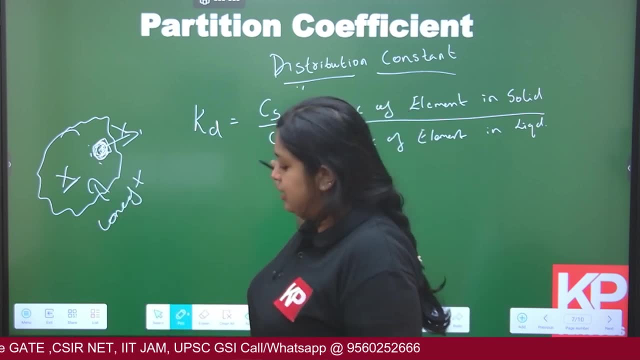 concentration of major elements, minor elements, trace elements, everything. So we can analyze the concentration of trace element in the liquid and the solid And if you take the ratio of concentration of this element in the mineral, then you can get the concentration of this element in the mineral. 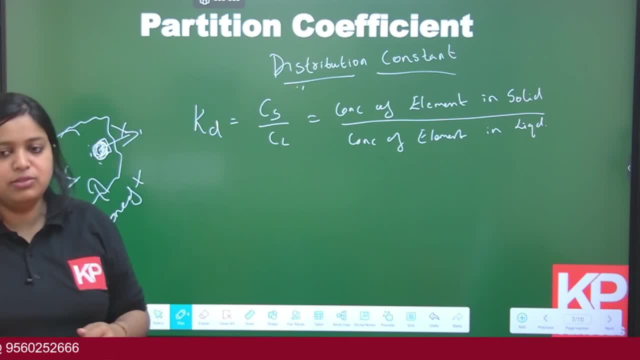 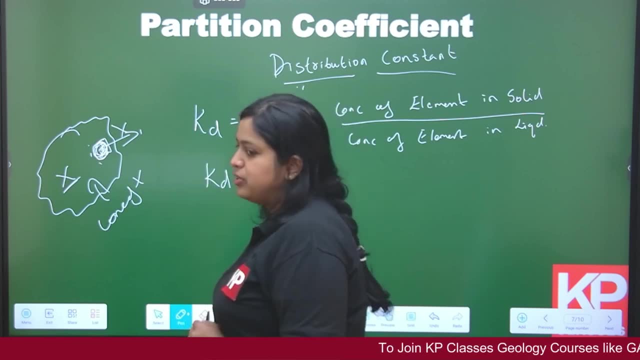 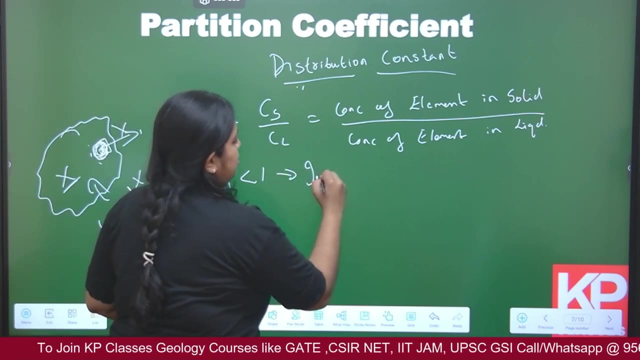 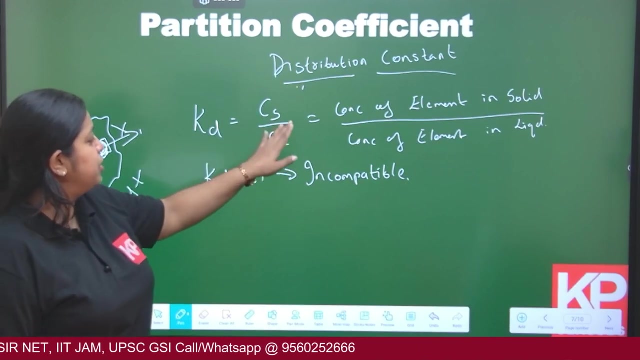 So in the solid to that of liquid, excuse me guys. So in if this ratio comes less than 1,, if this KD value comes less than 1, then we call the element X as incompactable element. Why? Because? why is it incompactable? Because if the ratio comes less than 1, that means 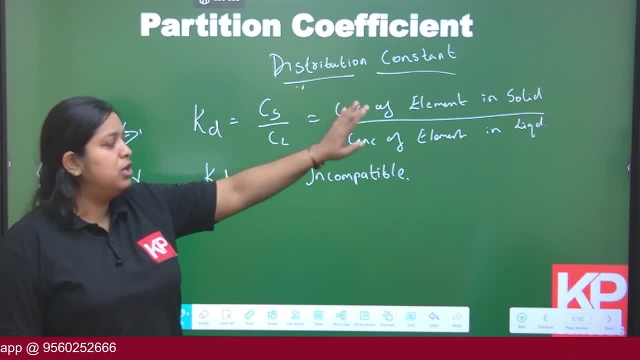 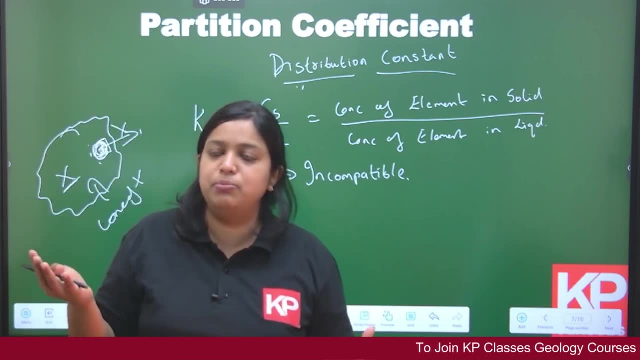 denominator is larger than the numerator, or denominator is larger than the numerator. So denominator here is concentration of element in the liquid. So if, if this element is more in the liquid than the mineral mineral phase or than in the solid phase, that means it is more it want. 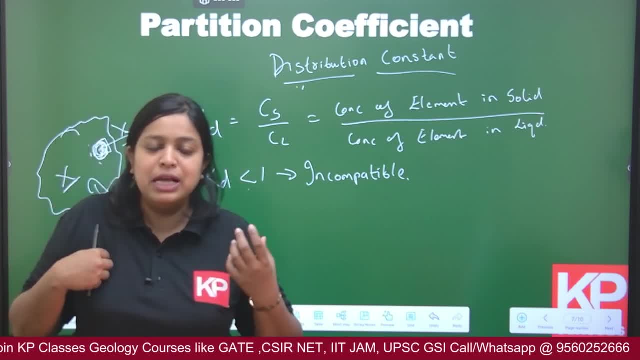 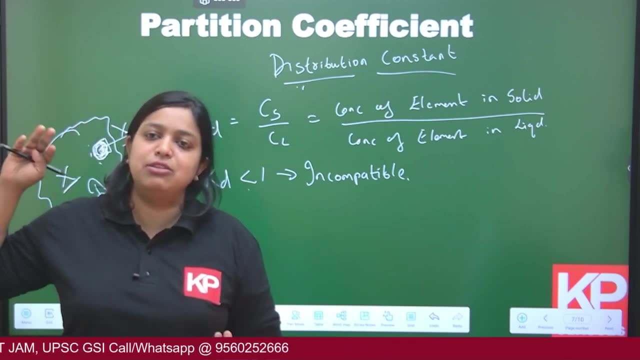 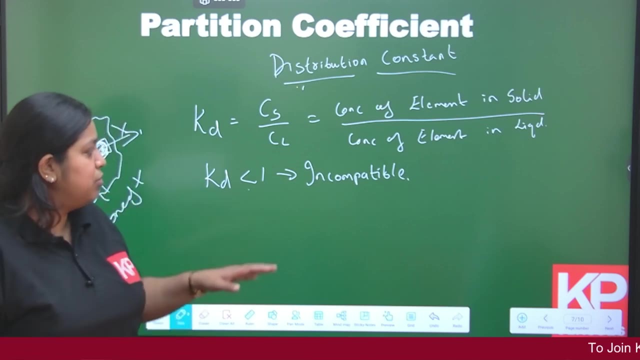 to stay in the liquid phase much higher, or it is more stable in the liquid phase than in the. its affinities towards the liquid phase is much higher than that of its affinities with the solid phase. That means it is an incompactable element or it is an incompactable trace element. So 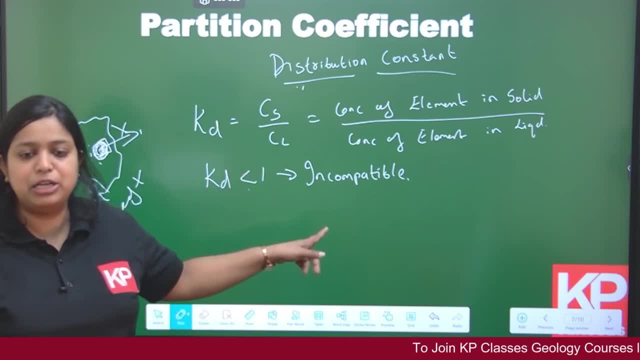 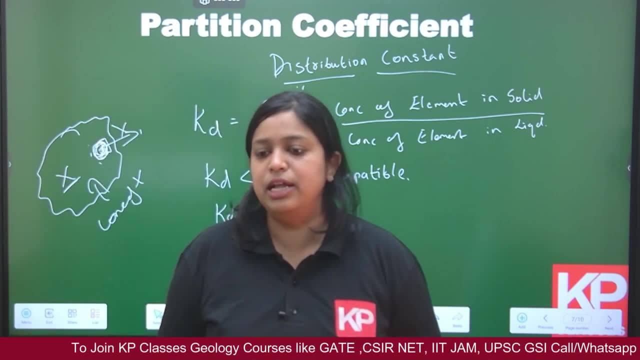 if KD value is less than 1, then we call the element X as incompactable element. So if KD value is less than 1, that element is an incompactable element. If KD value is greater than 1, then we call: then the element is actually a a compactable element. 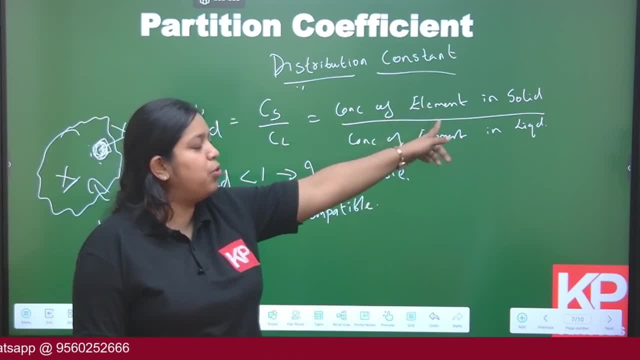 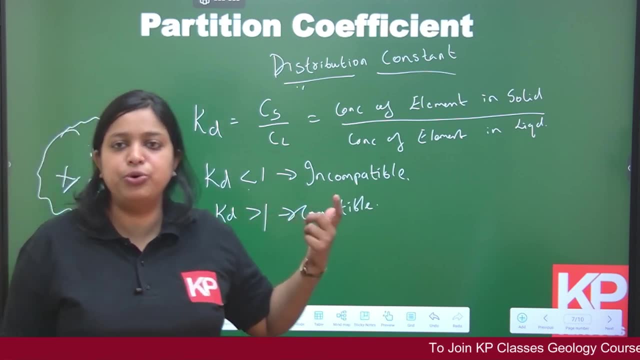 Compactable element greater than 1 means concentration of element in solid is greater than that of concentration of the same element in the liquid. That means this element can fit into a crystal. So if KD value is less than 1, that element is an incompactable element. So 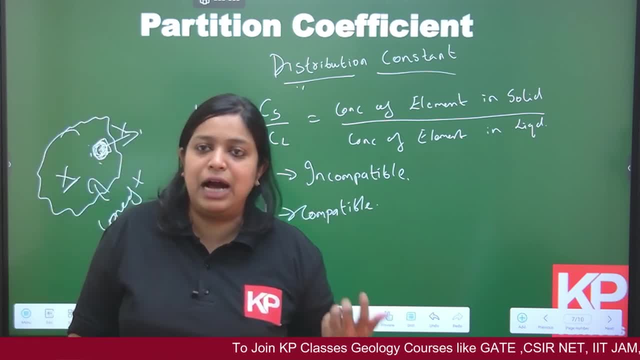 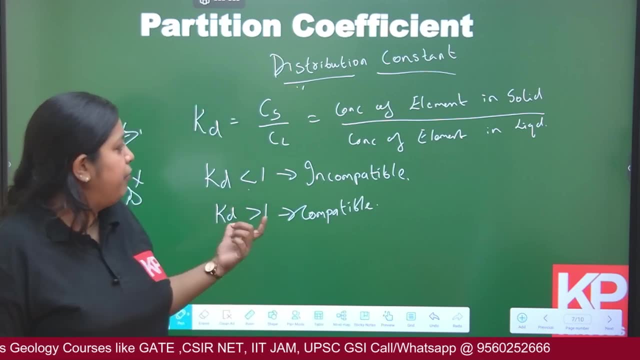 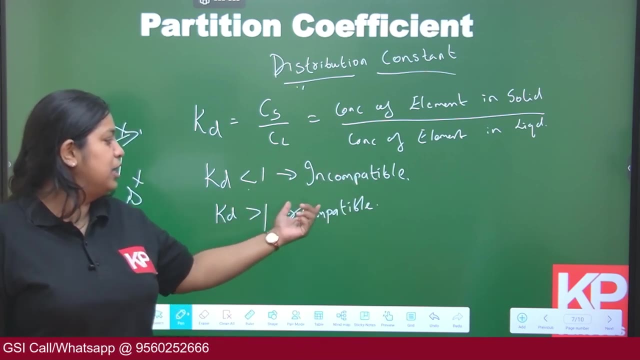 a structure, and that is affinity towards the solid phase is higher than that of the liquid phase affinity. Hence it is an compactable element. So KD value less than 1 means an incompactable element. If KD value of an element comes as greater than 1, that means it is a 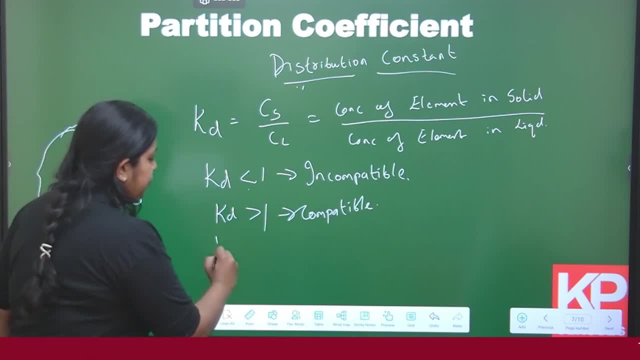 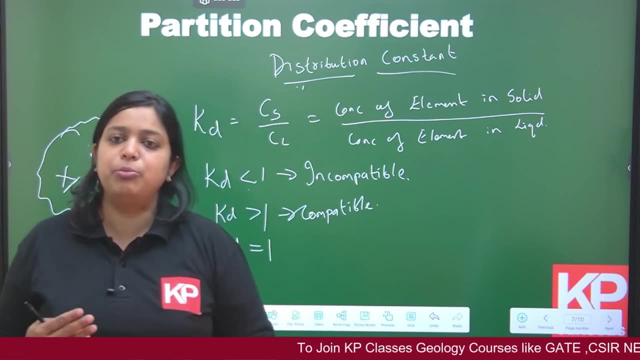 compactable element. And if KD value of an element comes 1 in a particular mineral, like in a sound principle, it is a compactable element. So if KD value is greater than 1, then it is a means KD value of an element comes 1.. That means it is neither compactible nor incompatible. 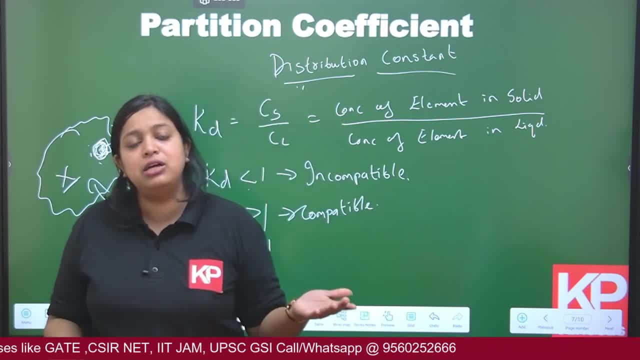 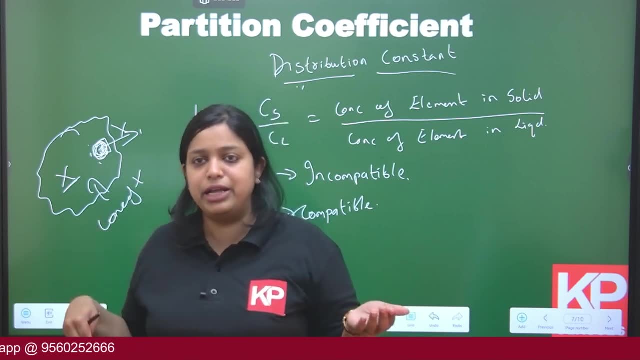 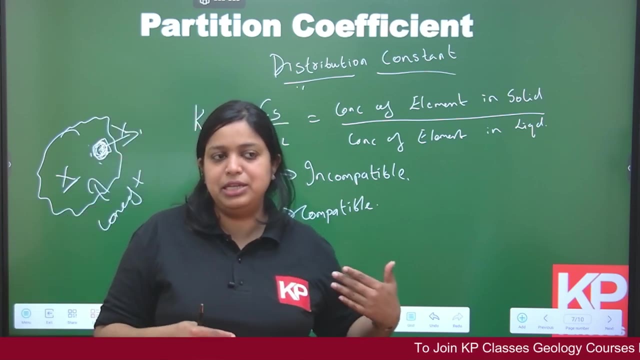 It behaves the same with liquid and the solid phase. Whatever percentage of concentration it went into the solid it equal percentage. it left back in the melt during crystallization Or during melting, when the mineral was melting, same amount of concentration of the element. 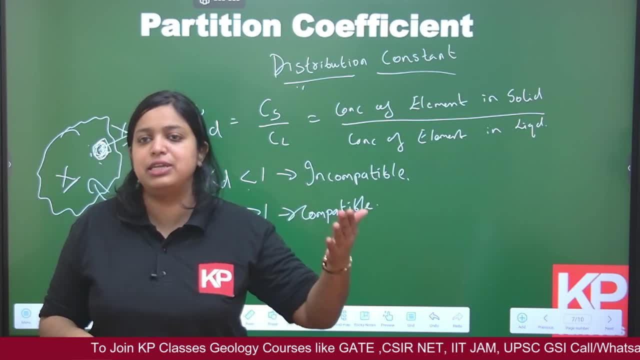 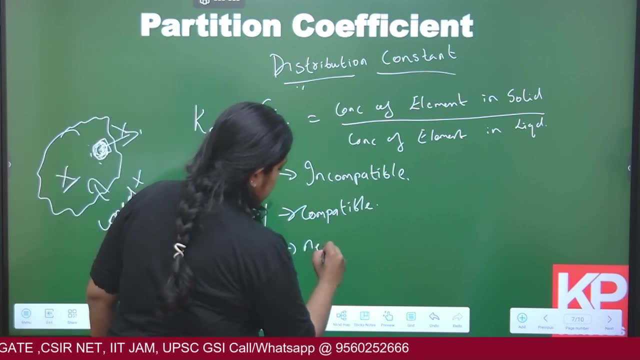 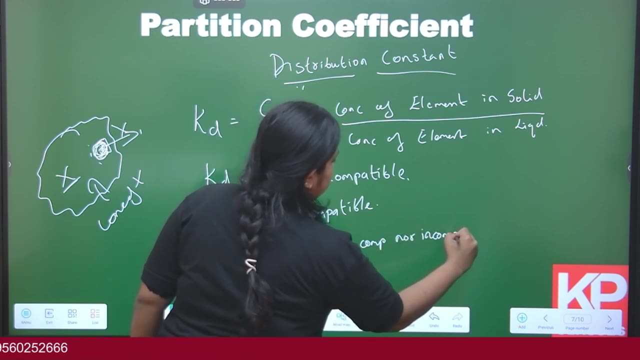 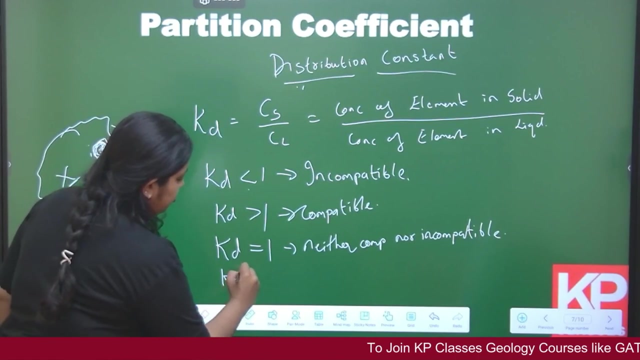 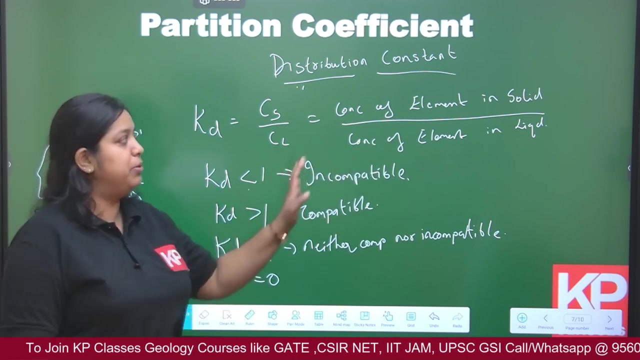 went to the melt phase and same concentration stayed in the solid phase. That means it is neither compactible nor incompatible, Nor incompatible. Now. if KD value is come, value comes as 0. That means it is a perfectly, perfectly incompatible element. The entire numerator part goes 0.. That is why the value 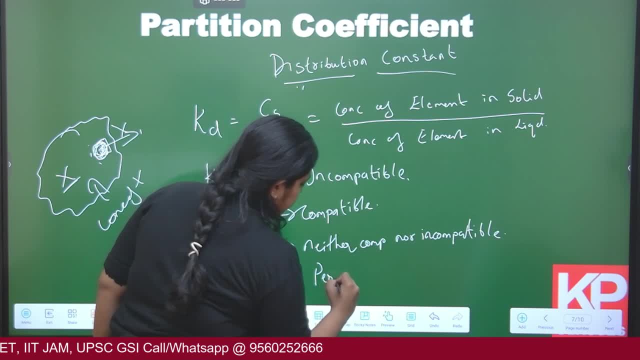 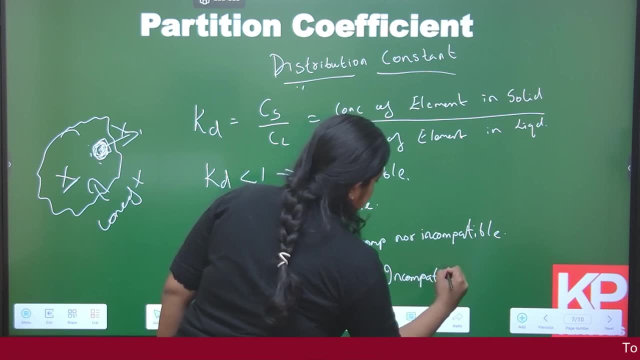 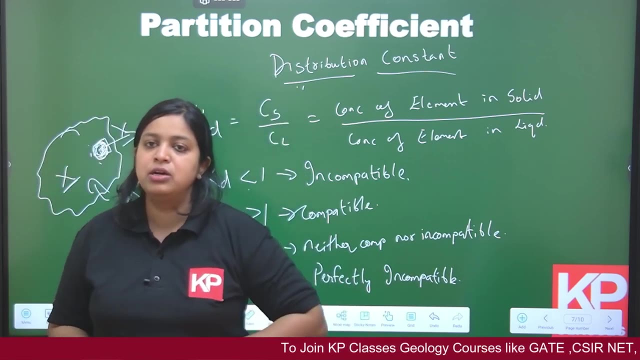 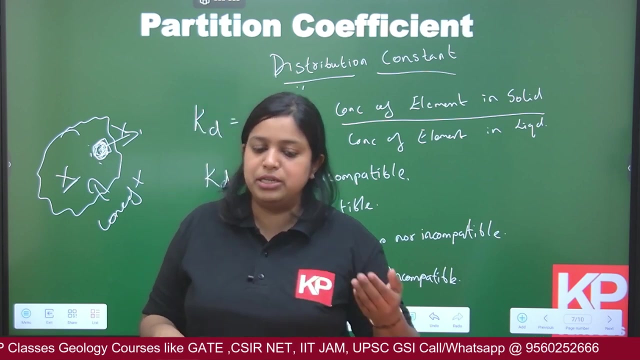 becomes 0. That means it is perfectly incompatible. Perfectly incompatible. So what we have discussed over here symbol an element, whether the element has an affinity towards a mineral, whether the element is a part Partition into the mineral phase while crystallization, or whether the element stays in the mineral. 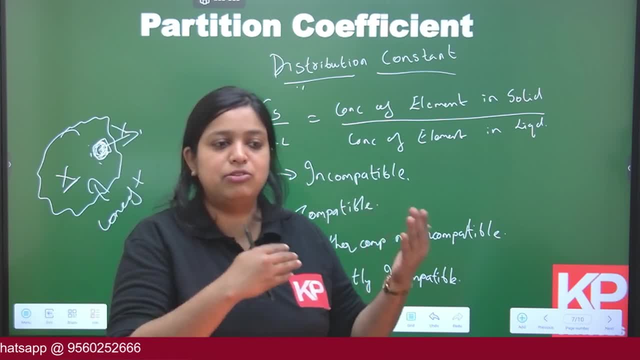 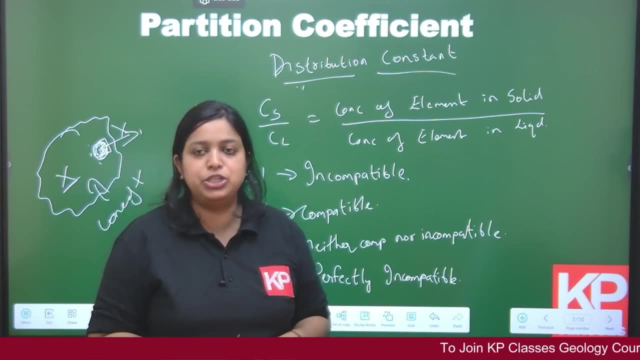 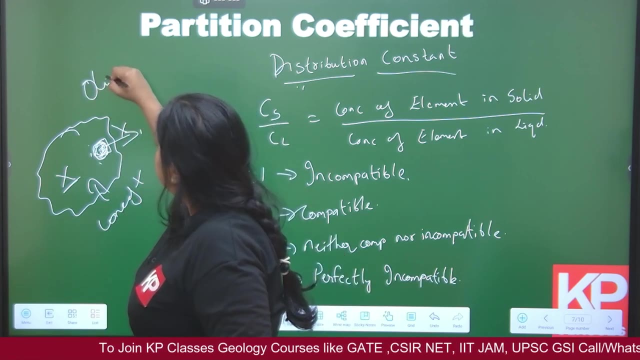 while melting. So, whether it has the affinity to stay in the solid phase or whether it has affinity to stay in the liquid phase, That is quantified by the terminology partition coefficient or distribution constant. For example, if a mineral olivine is crystallizing, 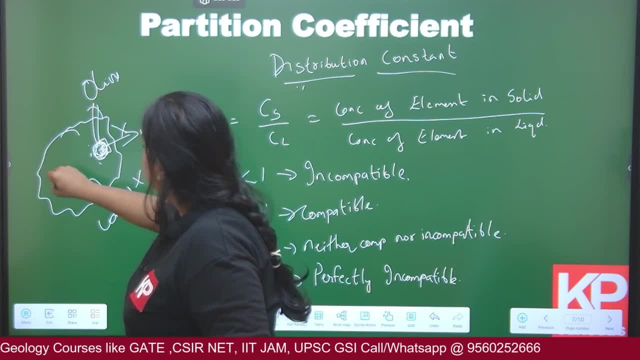 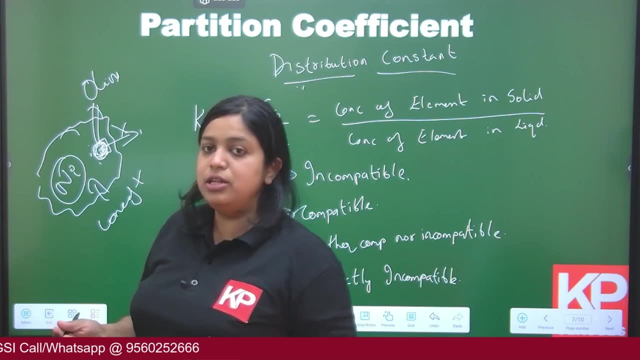 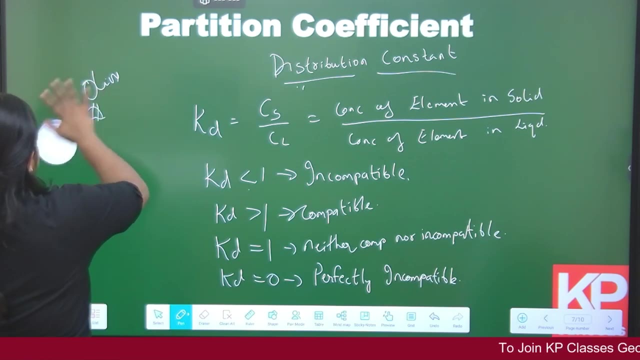 and we are talking about the element nickel, Nickel. So in the liquid. and imagine, olivine crystal is been an olivine crystal is been melting, So a melt has been formed. This is the melt. Now the, the concentration of 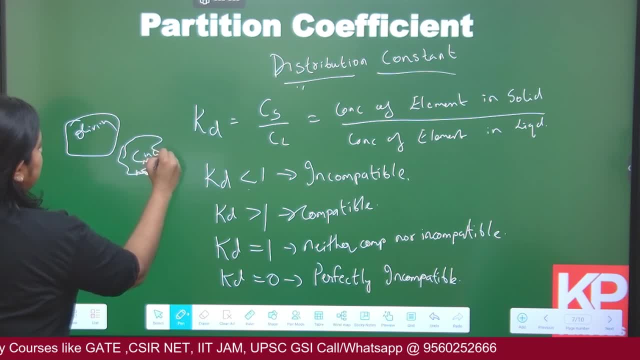 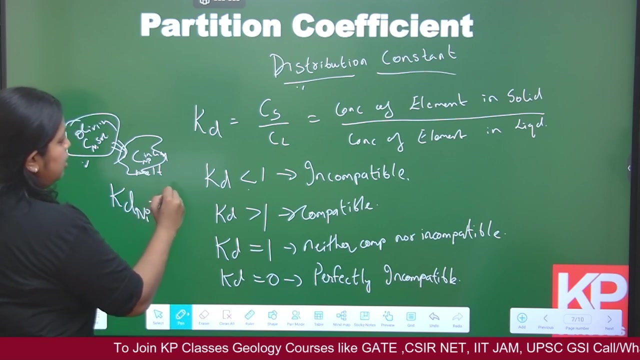 nickel in the liquid concentration of nickel in solid. I calculate the concentration of nickel in the olivine crystal, olivine mineral and melt from this particular mineral, Like when it got molten, the amount of nickel present in the melt. So if I calculate the k D value of nickel concentration in solid, nickel concentration. 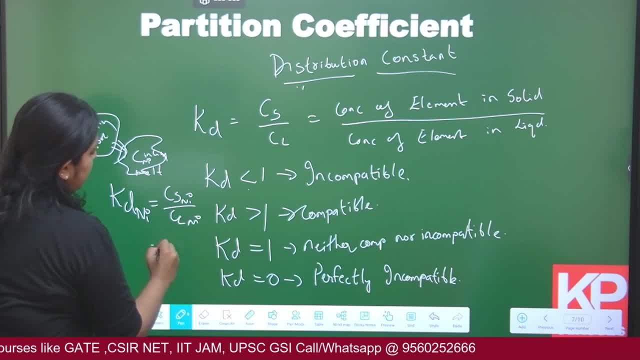 in solid divided by nickel concentration in liquid and if this value comes, value is greater than 1.. That means nickel is compactable in olivine. Nickel is compactable in olivine If Kd value comes greater than 1,. 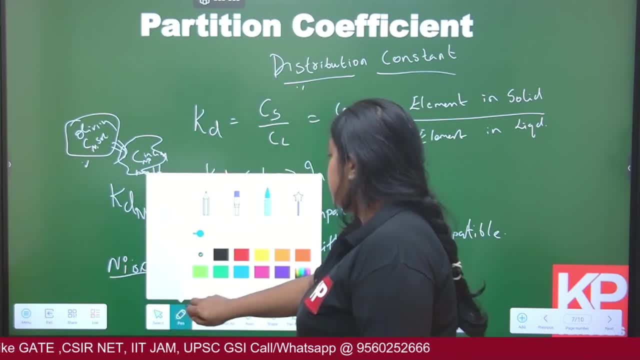 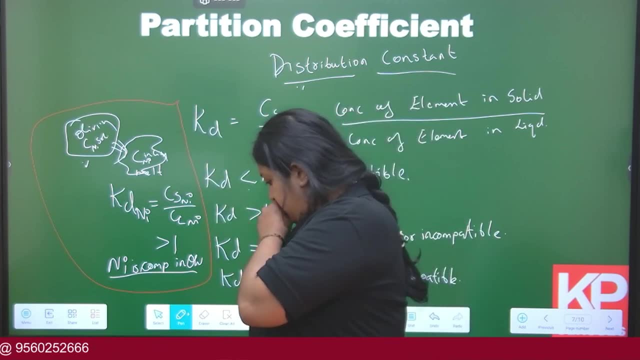 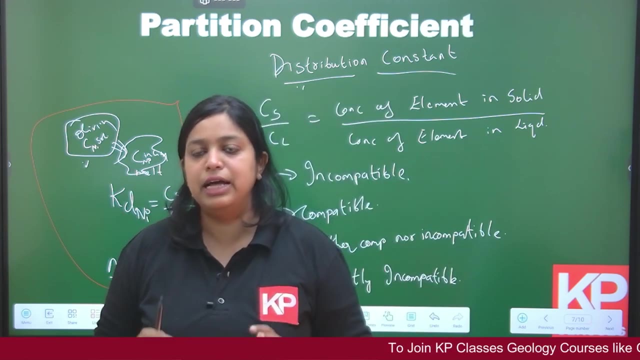 that means nickel is compactable in olivine. Actually, nickel is a compactable element in sorry. nickel is a compactable element in olivine. So olivine is a mineral and in that mineral, nickel as an element, whether it is compactable or incompactable, defined by the terminology. 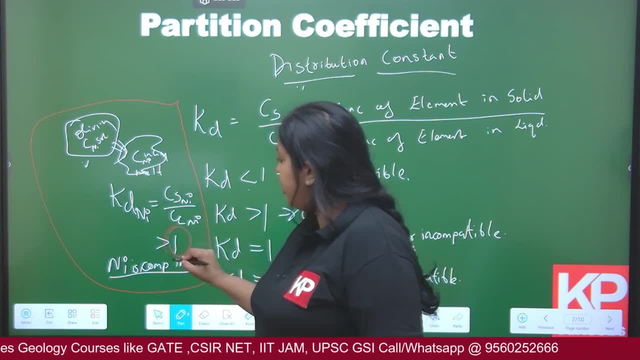 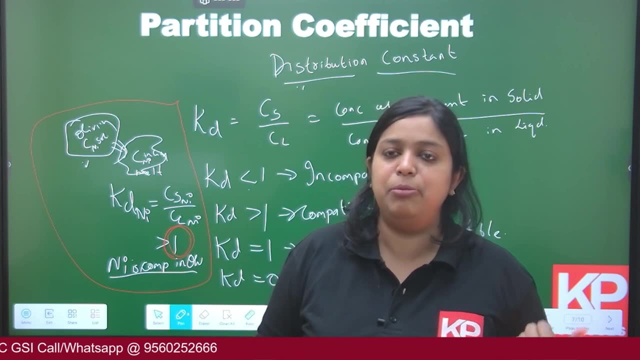 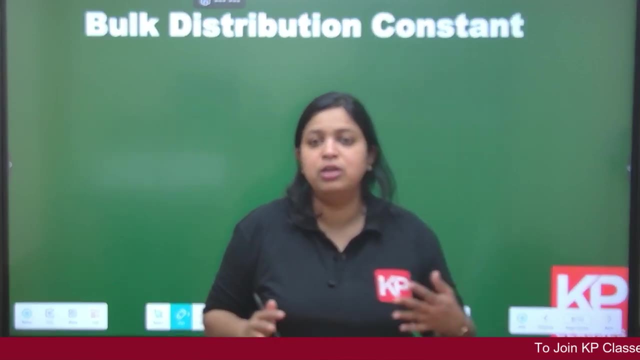 partition coefficient. So, depending upon whatever value I get over here that defines how compactable is an element or how incompactable is an element, that is defined by the partition coefficient terminology. Now, as we know that a rock is not only simply consisting of a single mineral, For example, a single set of rock may have three different types of minerals. So this is a single rock for a garnet, lahersalite or lapidotype, simple in any in a garnet, sorry, a granite. or a mid-oceanic rich basalt. 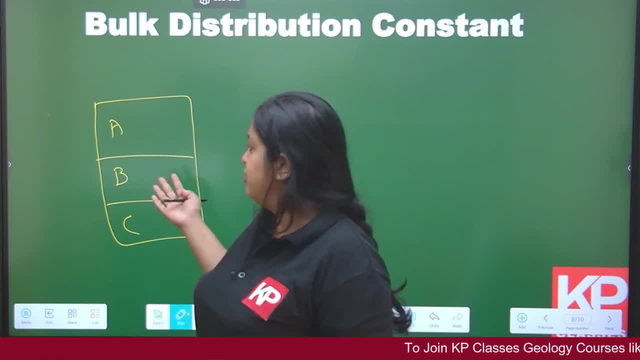 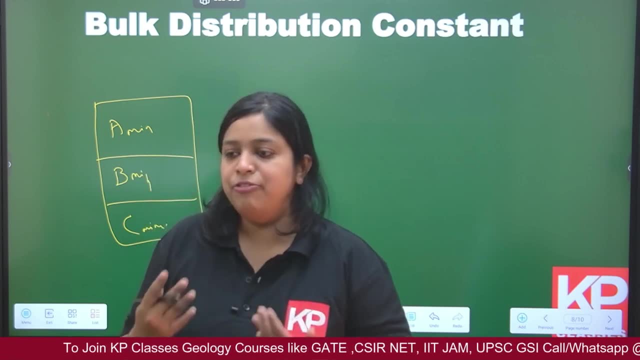 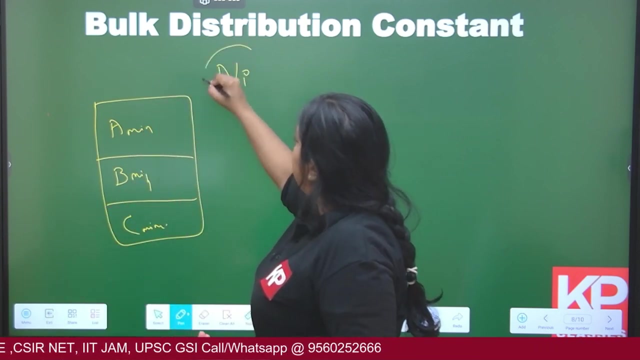 suburb and then a single rock over here. Rocks are aggregated minerals. There are different, different minerals present. So this is a mineral, b mineral and c mineral. Now, if I want to analyze whether an element, for example nickel, whether the nickel element is compactable in 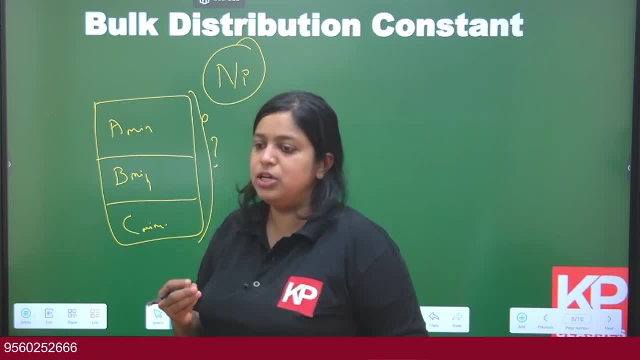 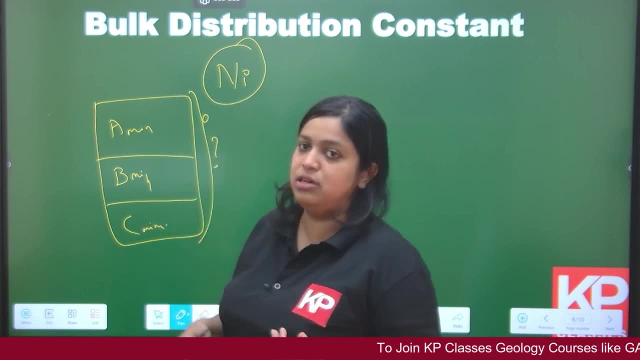 this whole rock, or whether the nickel element is incompactable, or whether the the amount of nickel is higher in rock or lesser, or whether it is compactable to the whole rock or not. that is defined by bulk distribution constant or bulk distribution coefficient. defines: 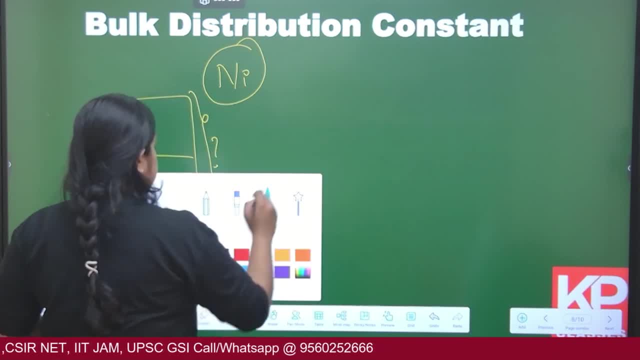 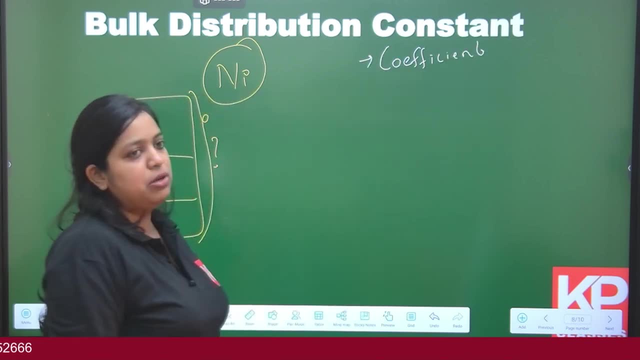 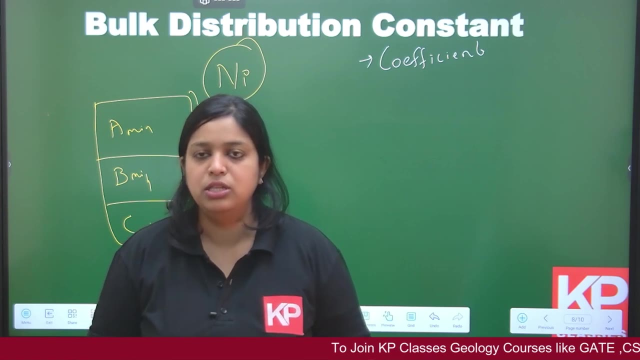 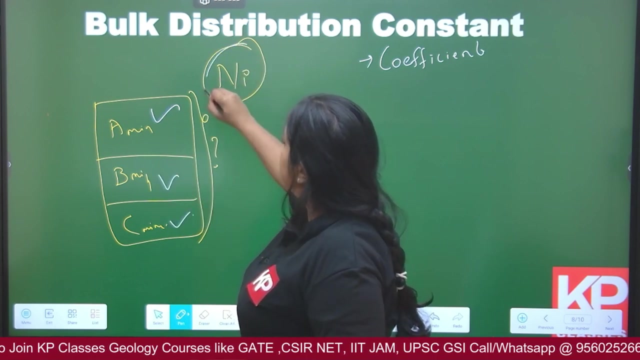 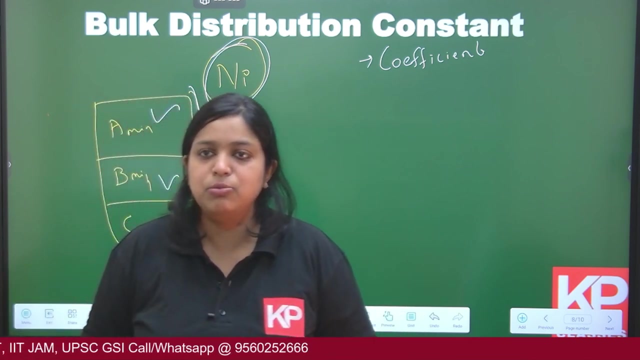 bulk distribution, constant or by coefficient defines the percentage or or the compactability of an element in a whole rock. that is defined by bulk distribution coefficient. so their single rock consists of different different minerals, so and whether the nickel is compactable in this rock or not, that is defined by bulk distribution coefficient. bulk distribution coefficient is: 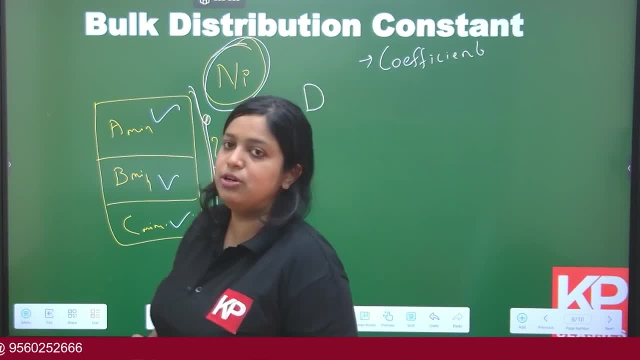 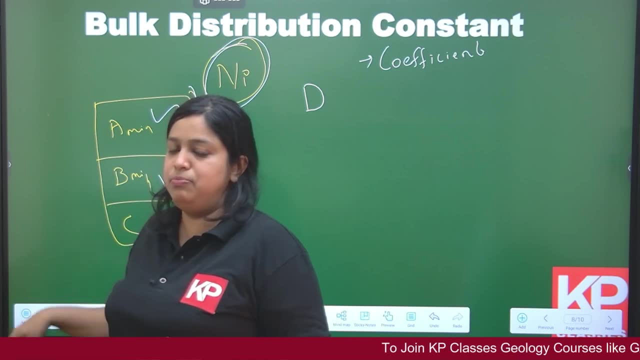 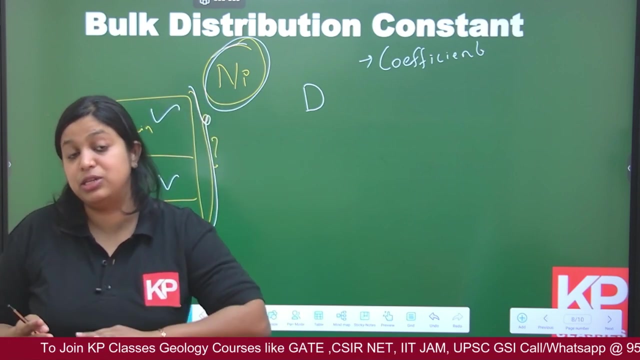 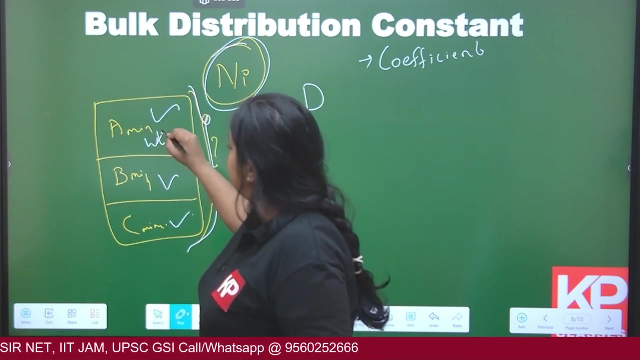 notated by the letter d is what we use to define the bulk distribution coefficient. so it depends upon the weight fraction of each of this mineral weight fraction of minerals contributing to the melt. that is what is defined by the. that is what one of the factor of bulk distribution coefficient that means, what is the weight percentage of mineral a. 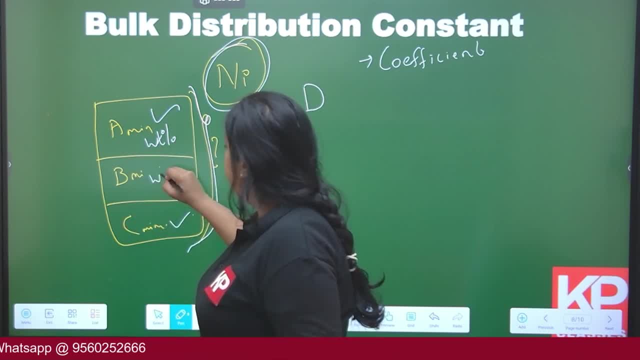 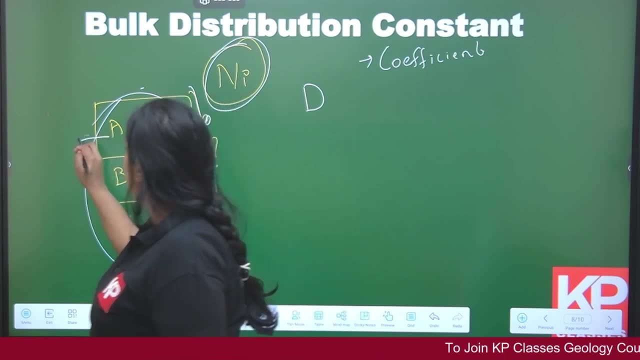 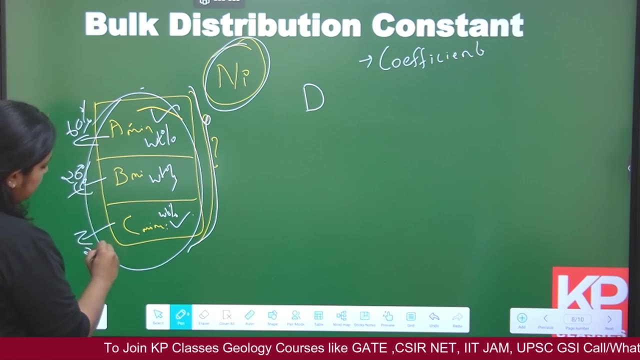 what is the weight percentage of mineral b and what is the weight percentage of mineral c in the rock? maybe a is weight percentage of a may be 60 percentage, b may be 20 percentage and c is also 20. so this is the weight percentage, for you have to consider the mass or weight percentage. we are not. 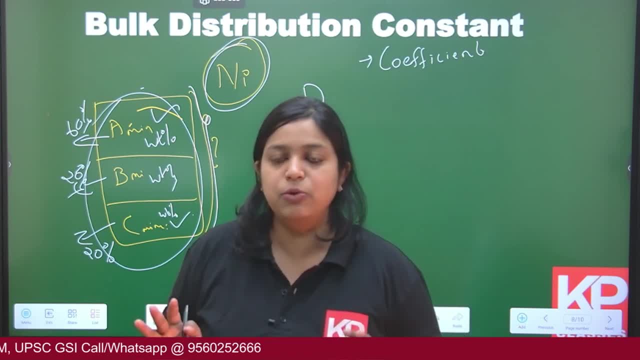 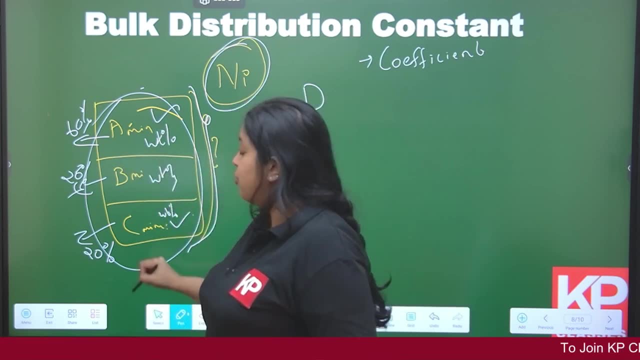 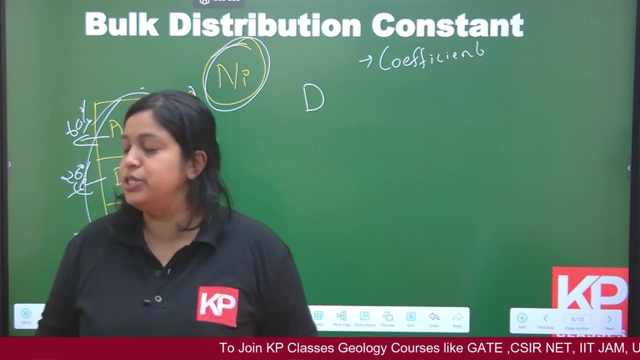 considering the volume percentage. over here we are considering the weight percentage of the mineral present in the rock. okay, so weight percentage of each mineral present in the rock is one of the factor that defines the bulk distribution coefficient. so how to calculate the bulk distribution coefficient? we know from the previous partition coefficient. 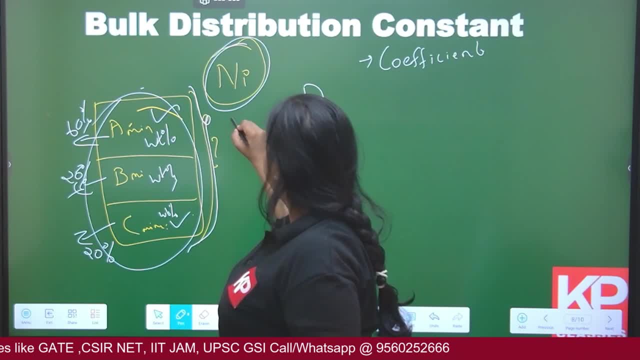 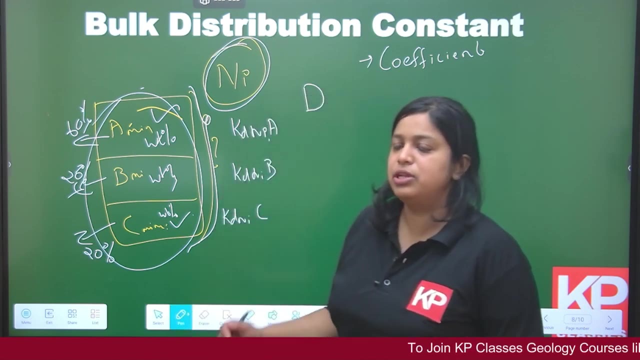 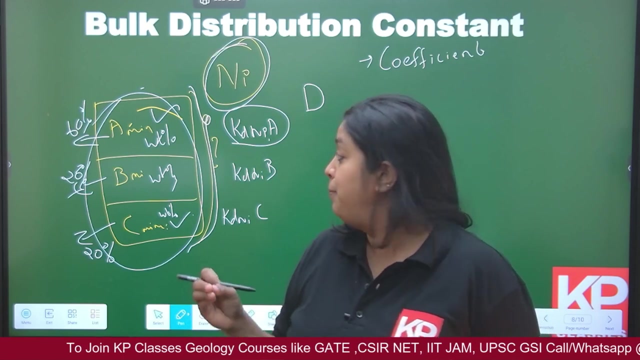 we know that we can calculate the kd value of nickel in mineral a and kd value of nickel in mineral b and kd value of nickel in mineral c can be calculated right mean. kd value of nickel in mineral a means the whether the amount of nickel present in the mineral a and the kd value of nickel 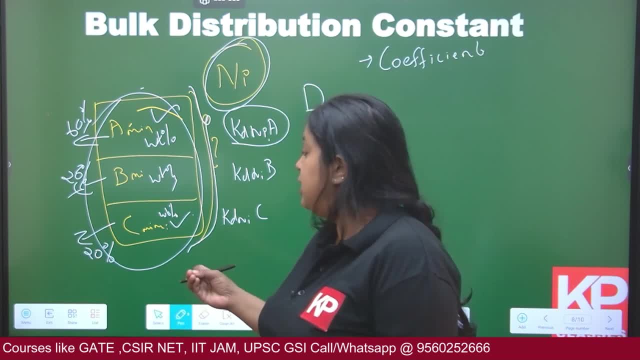 in me b and kd value of nickel. in c means the value of manganese」. Here you will see that the ratio of liquid than the mass, the m and the weight distribution coefficient. you can do you calculate the value to enjoy in the mineral a and the grinding ratio to enjoy in mineral c, its equal. 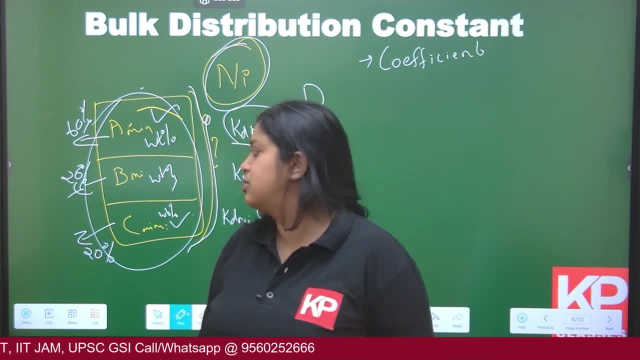 Broken line detracts you, Aruna, sir, is that okay? Voyager00110006 And p in between. the measure is d, it should be 파� to review means amount of nickel that is present in b and the that of c means amount of nickel present in c. 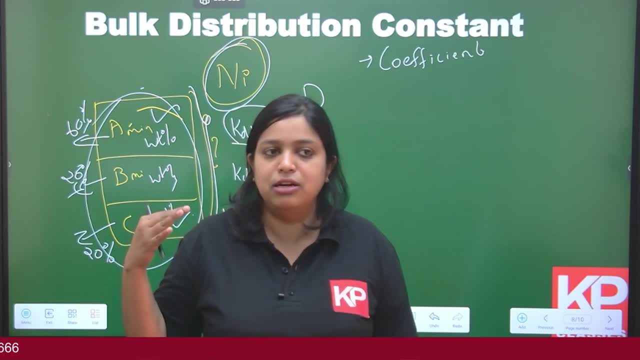 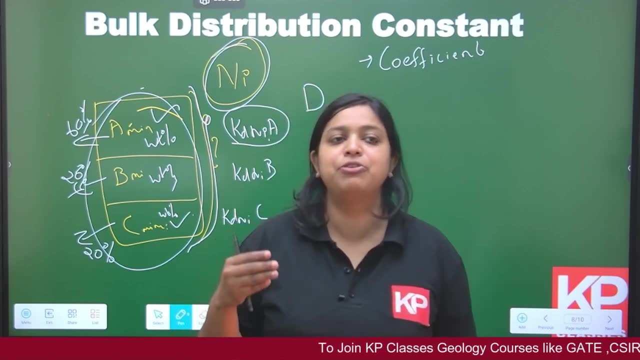 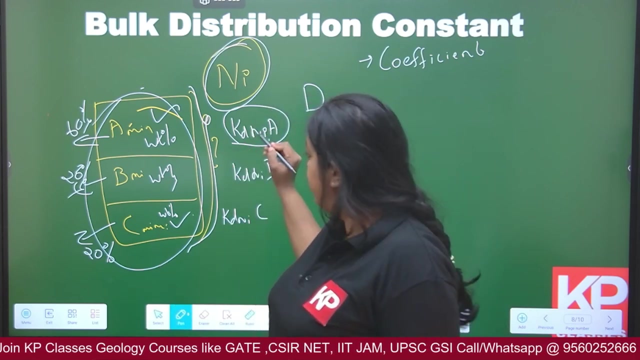 or the ratio of concentration of nickel in mineral to that of the liquid, ratio of concentration of nickel in mineral b to that of the liquid. ratio of concentration of nickel in mineral c to that of the liquid is defined by the kd values now, and we know the weight percentage also. no weight. 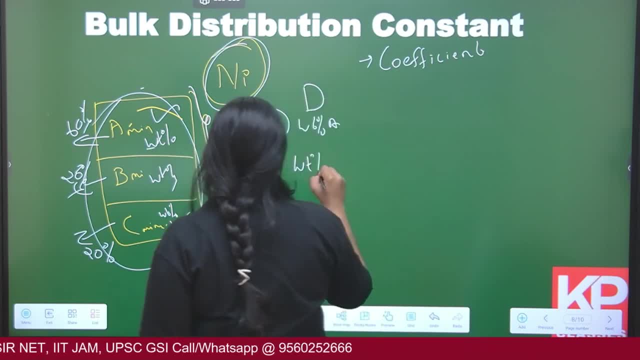 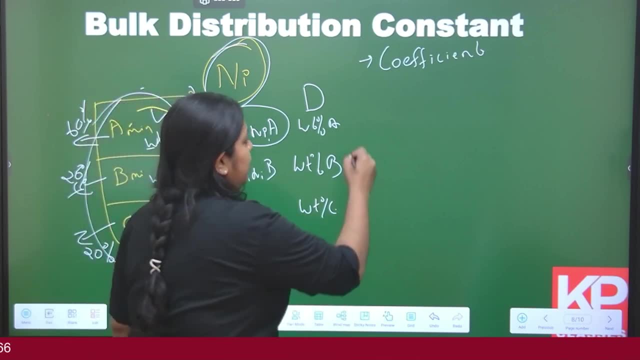 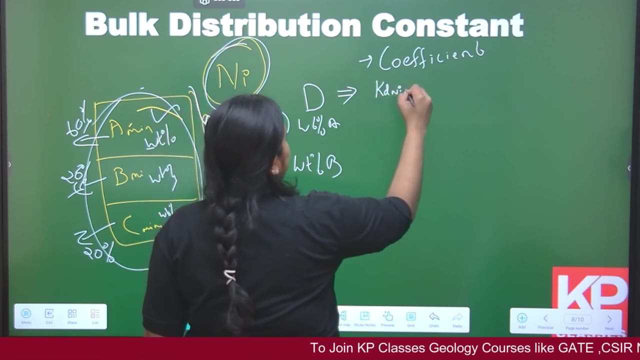 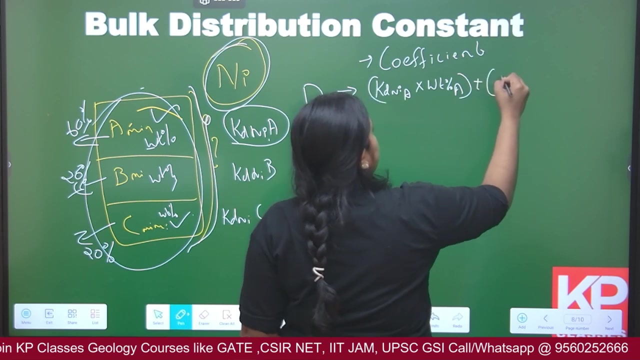 percentage of a is also no. weight percentage of b is also known. weight percentage of c is also not. now, by using all these terms we can calculate the bulk distribution coefficient. bulk distribution coefficient is kd value of nickel in a into weight percentage of a plus kd value of nickel. 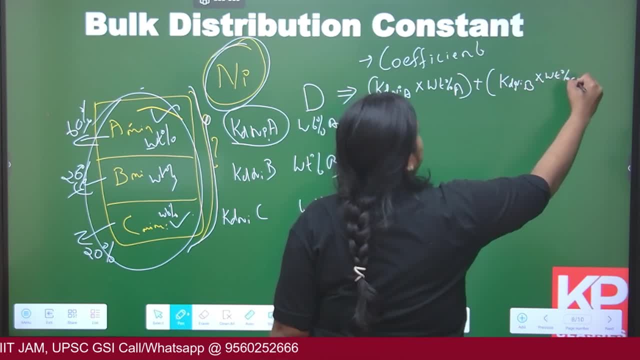 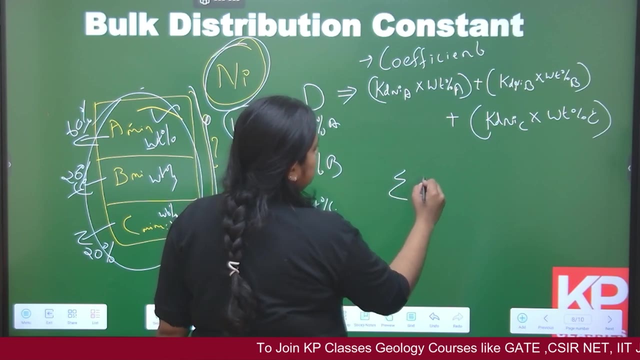 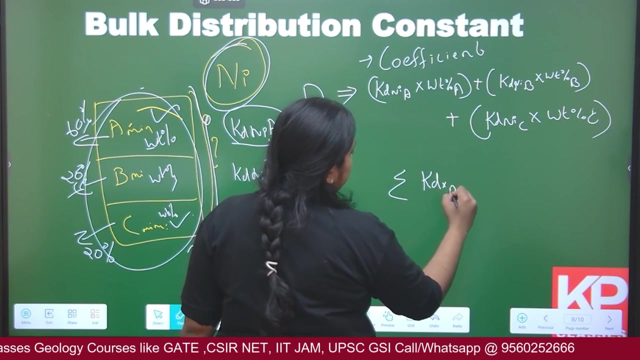 in b into weight percentage of mineral b, plus kd value of nickel in mineral c into weight percentage of mineral c. so summation of, simply, if i write it, d means summation of kd value of the element x in all the minerals a, whatever it is, into the weight percentage of that mineral. so summation of this, how many? 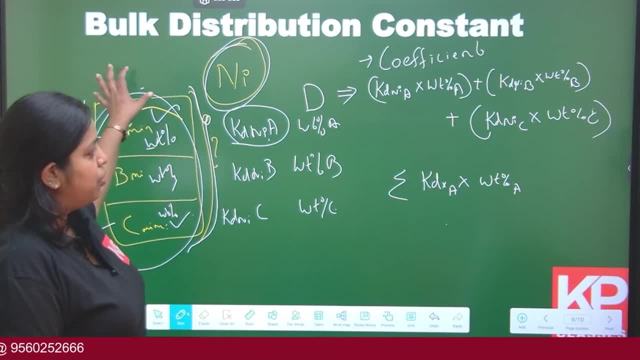 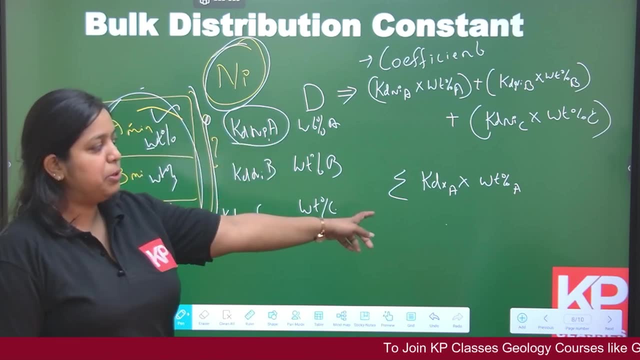 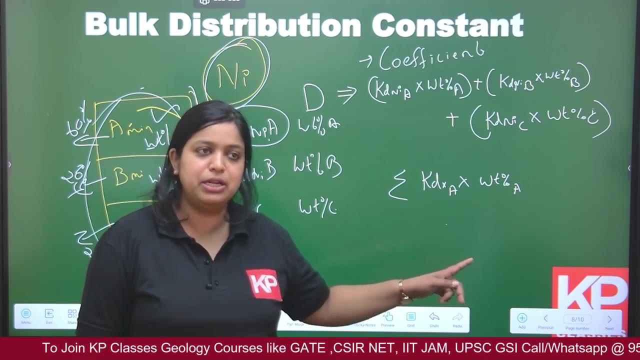 minerals some. maybe there may be six minerals present, so the whole six minerals. kd values of that particular element and its weight percentage. multiply the kd value and weight percentage of the kd value of a particular element in that mineral and the weight percentage of that mineral. multiply it together. add of same values of different, different minerals. add it together. 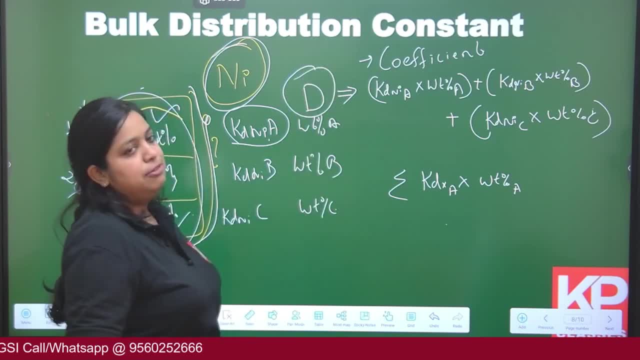 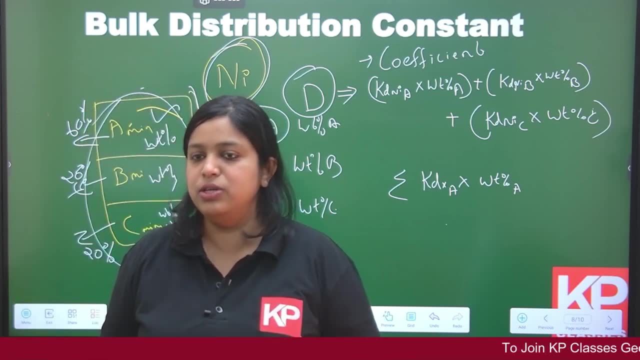 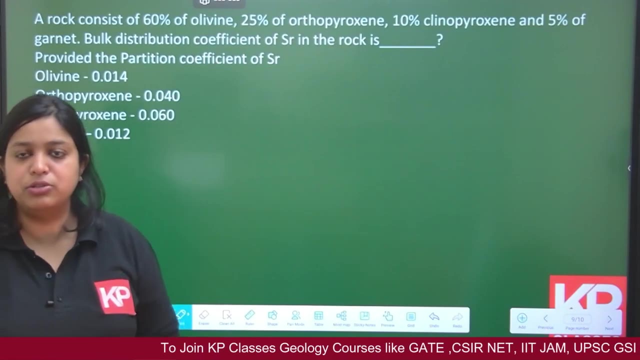 you will get the bulk distribution coefficient, which defines the emulsion amount of or the distribution of an element in a particular rock. that is what is defined by the bulk distribution coefficient. now here the usually a numerical questions do come from this section. this is one of the numerical question. a rock consists of sixty percentage. 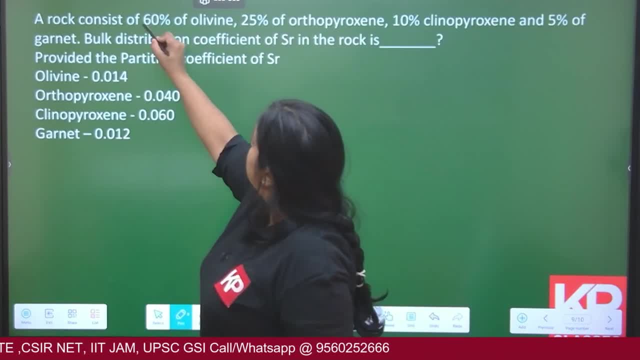 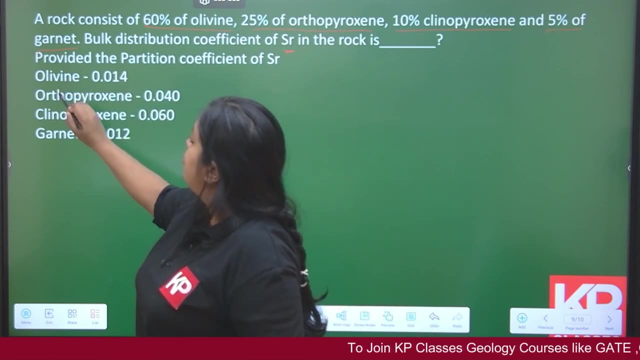 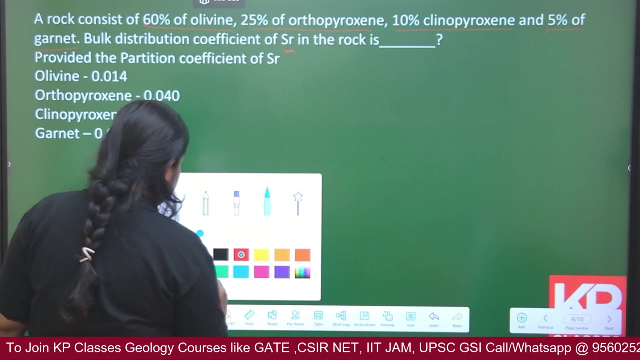 of olivine, ah. twenty five percentage of ortho pyroxene, ten percentage of crinopyrroxene, five percentage of garnet. bulk distribution coefficient of strontium in the rock is equal to kd value of strontium in each of the mineral spices, or you may have heard of the. 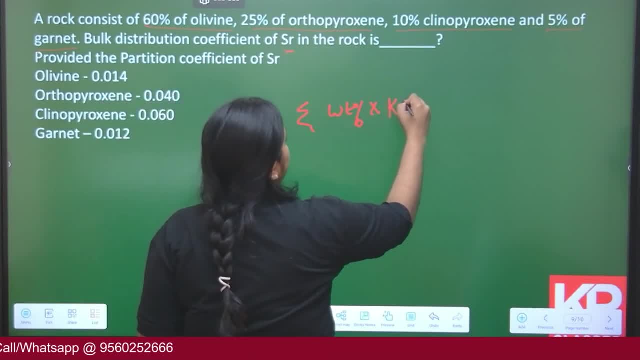 健itzize process for doing so. one of the things that we refer to the end Early Potition Americans was this: co-industrialrika. ok, this part we could by this, we could get that chased started. we can got that. we could get that that pass. 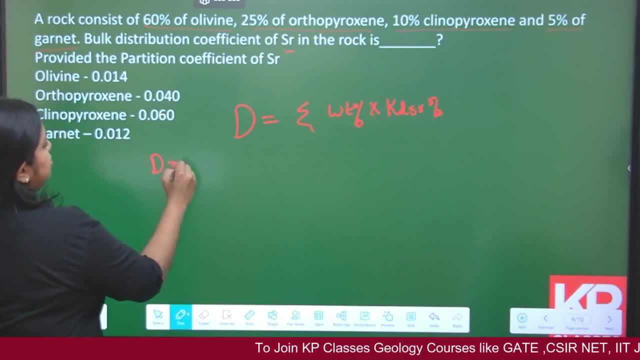 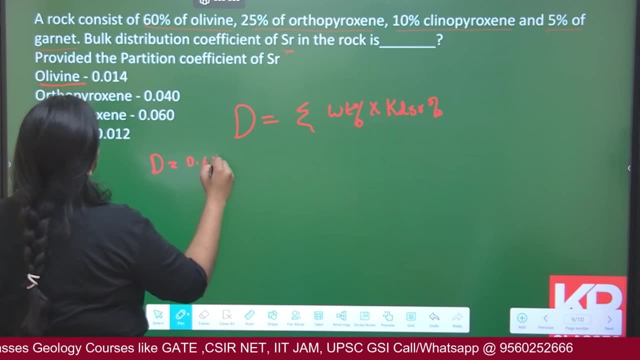 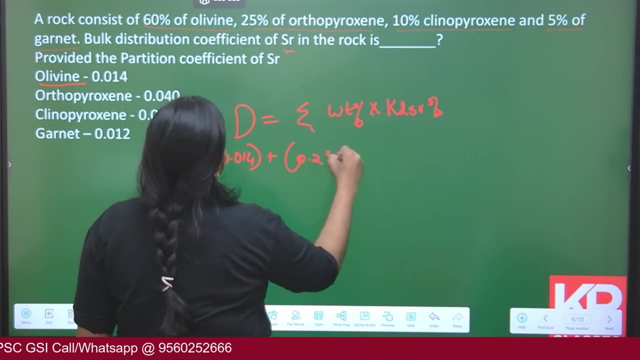 is d, So we know if I calculate d is equal to. first let us take olivine. Olivine's weight percentage is 60 percentage. that means 0.6 into 0.014 plus 0.25 into that of orthoperoxin. KD value of strontium in orthoperoxin is 0.040 plus 0. the percentage of clinoperoxin is 10.. So 0.10 into what is. the KD value of clinoperoxin is 0.060 plus. 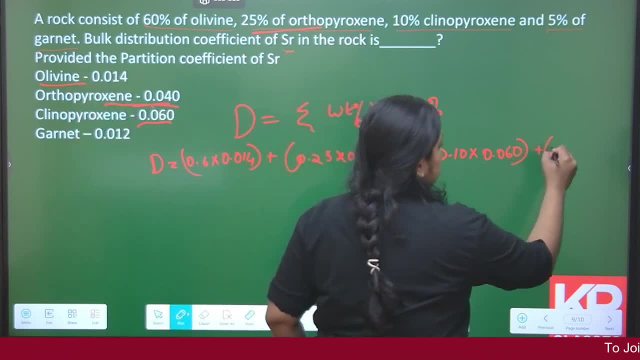 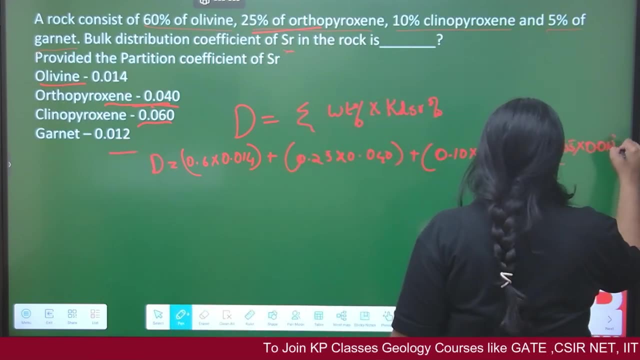 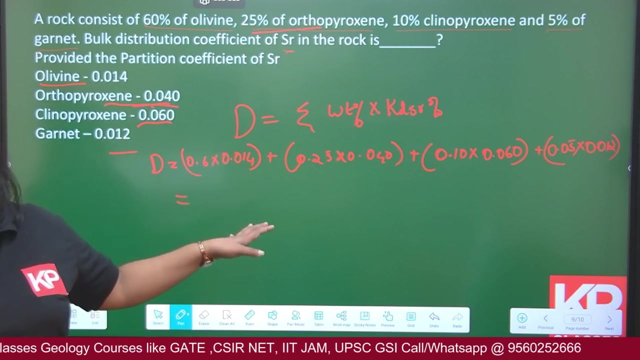 garnet weight percentage. Weight percentage is 5. percentage that means 0.05 into ah 0.012. that is the KD value of garnet, KD value of strontium in garnet. So if you solve this out you will get the bulk. 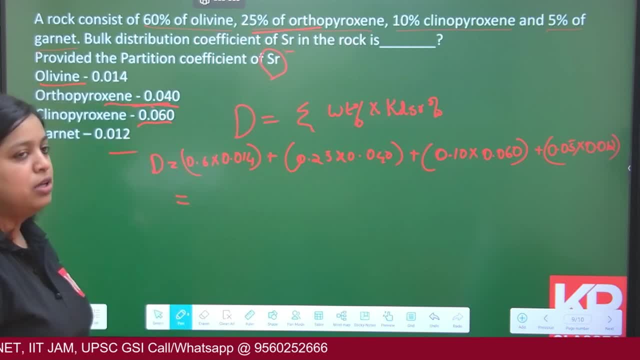 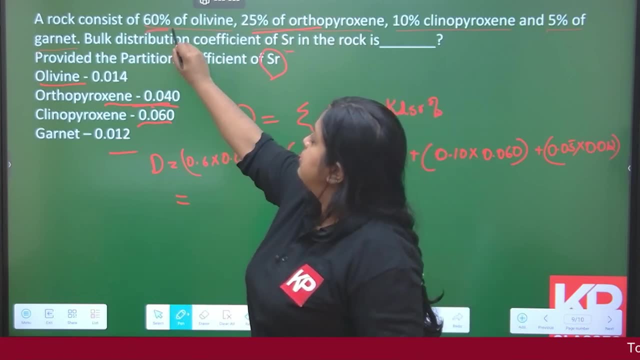 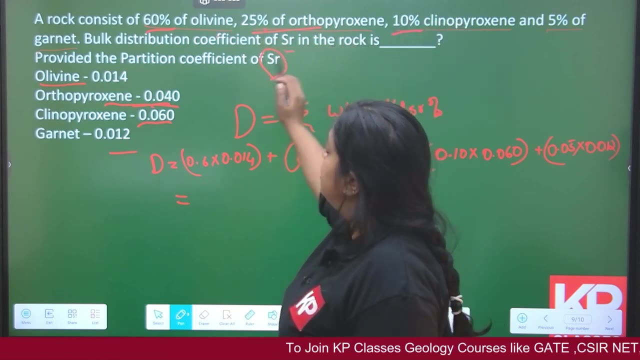 distribution coefficient of strontium in the rock. The rock that consists of olivine, clinoperoxin, orthoperoxin and the garnet in these bulk weight percentage: 60 percentage of olivine, 25%, 10 percentage of clinoperoxin and 5 percentage of garnet. The partition coefficient of strontium. 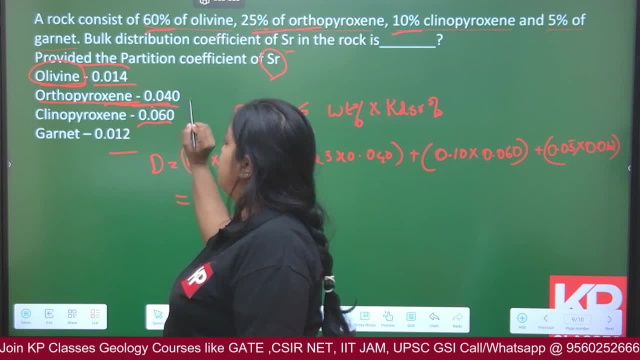 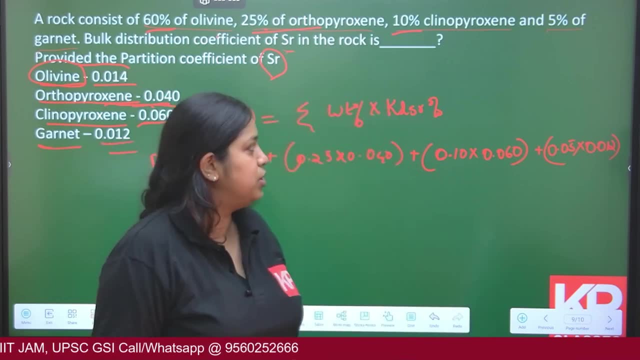 in olivine is 0.014, that of orthoperoxin is 0.040, clinoperoxin is 0.060, garnet is 0.012.. So equation for calculating the bulk distribution coefficient is summation of weight percentage. 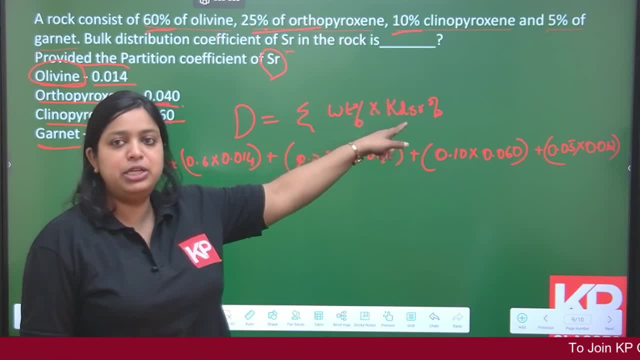 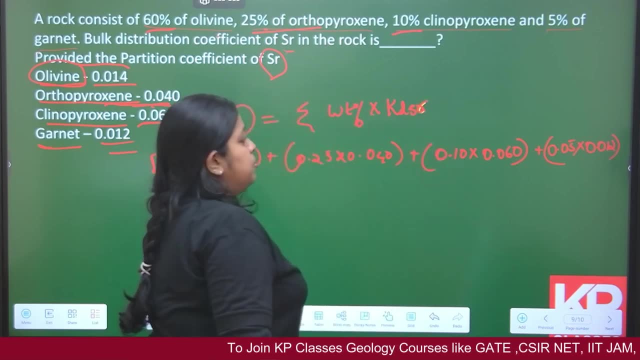 of each mineral multiplied by KD value of strontium in each mineral. So I do not know where I put this. Sorry, there is no Percentage sign. So D is equal to 0.6 means because 60 percentage of olivine. So though, 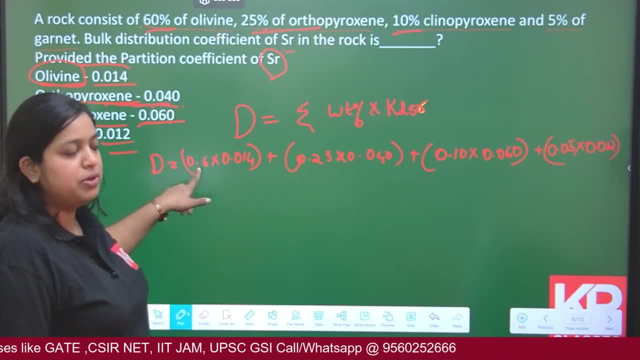 it is in percentage value. here you have to put remove the percentage. that is why it becomes 0.6- into KD value is 0.014.. 25 percentage: 0.25 into 0.040.. 10 percentage becomes 0.10. 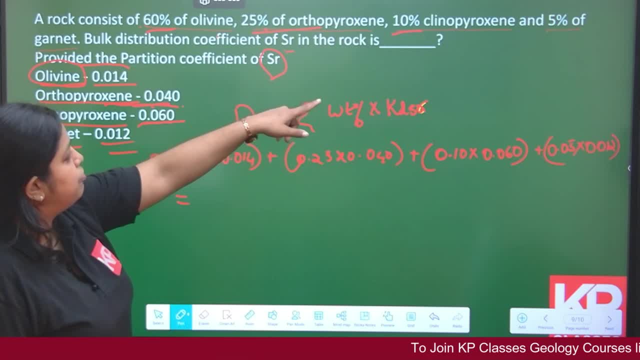 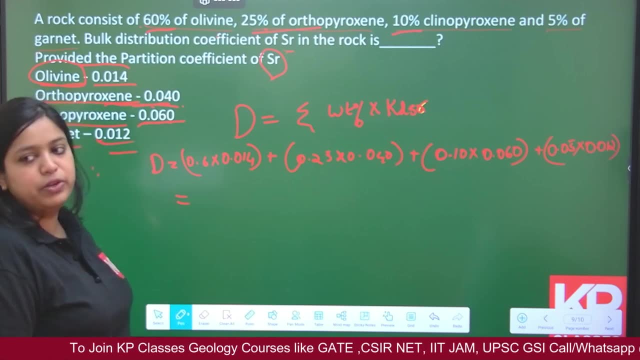 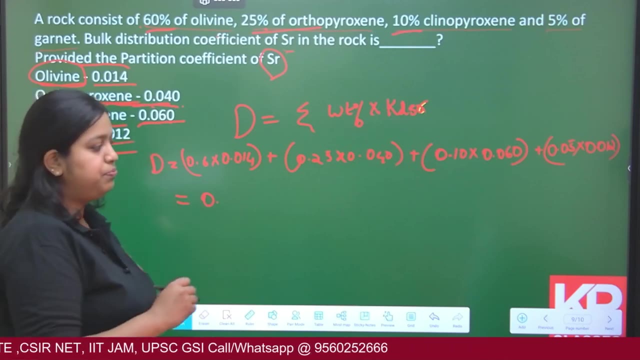 into 0.060 plus 0.05.. 5 percentage is 0.05 into 0.012 is the KD value of strontium. So if you solve it out, you will get value of 0.25- 0.025- something value you will be getting. 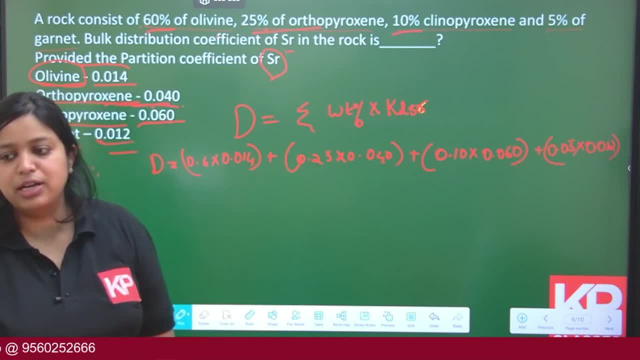 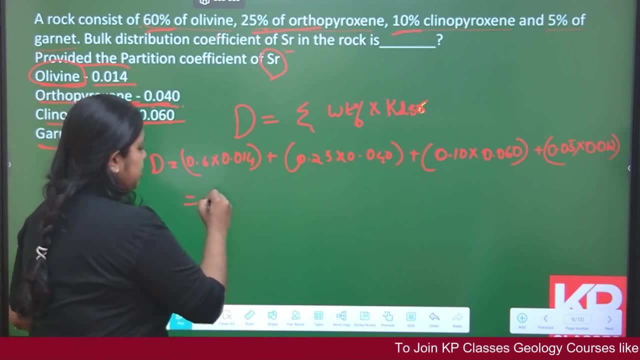 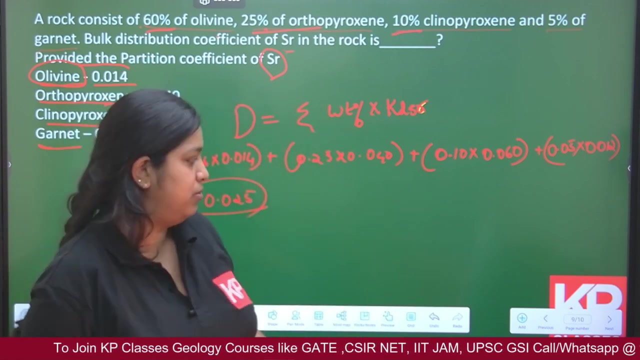 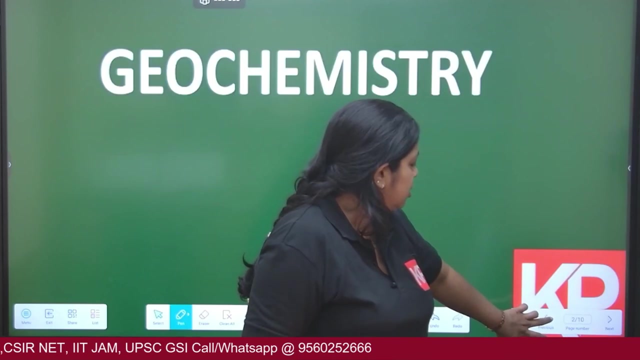 You guys check the value and if you guys have any doubt related to this section, like if you are not getting the equation or if you are not getting the value, let me know in the comment section. will help you out over there. So today, simply, we have defined about the bulk distribution coefficient, partition coefficient.